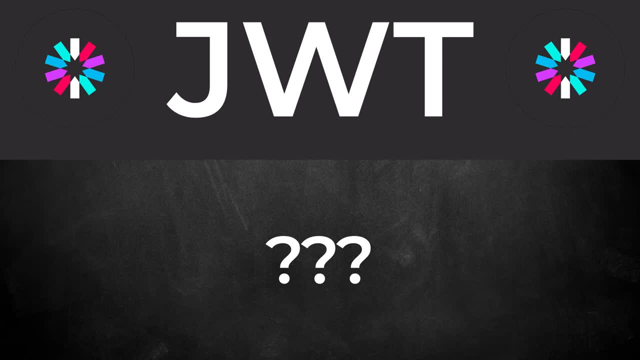 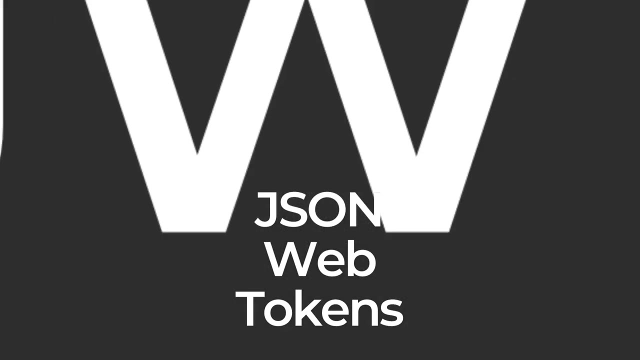 we're going to implement today. So what are JWTs? What is the acronym JWT in abbreviation for? Well, I'm very excited about the upcoming launch of the James Webb Telescope, but in this case, that is not the correct answer, Concerning our Node and Express REST API. JWT is an abbreviation. 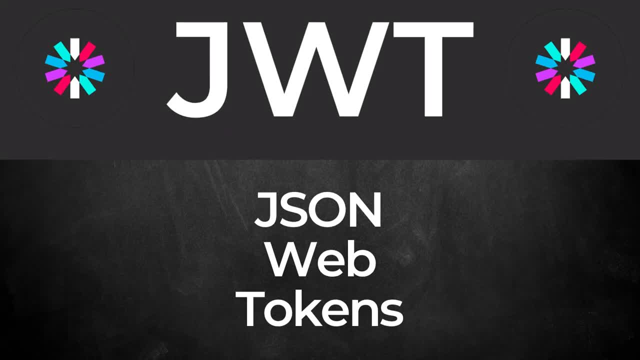 for JSON Web Tokens. JWTs can be considered to be a form of user identification that is issued after the initial user identification. So what are JWTs? JWTs are a form of user identification that is issued after the initial user identification. So what are JWTs? JWTs are a form of user identification. 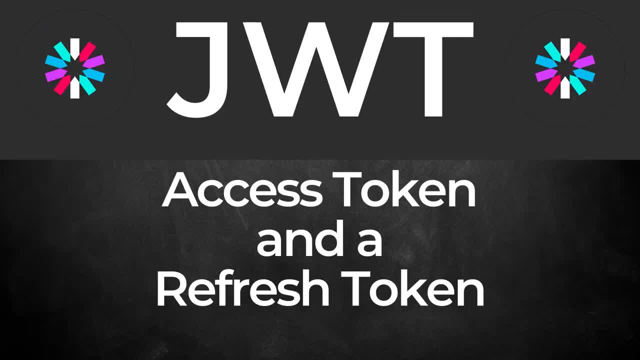 that is issued after the initial user identification takes place. When a user completes their login process and they are authenticated, our REST API will issue the client application an access token and a refresh token. The access token is given a short time before it expires, for example. 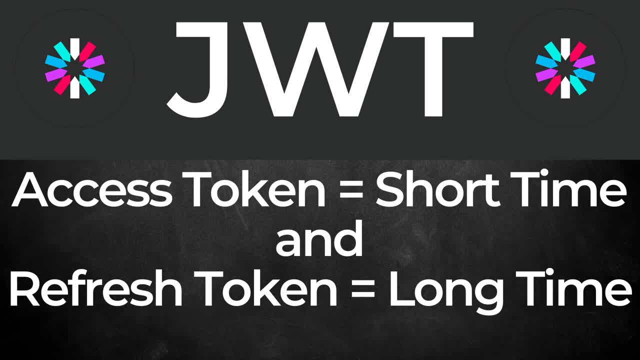 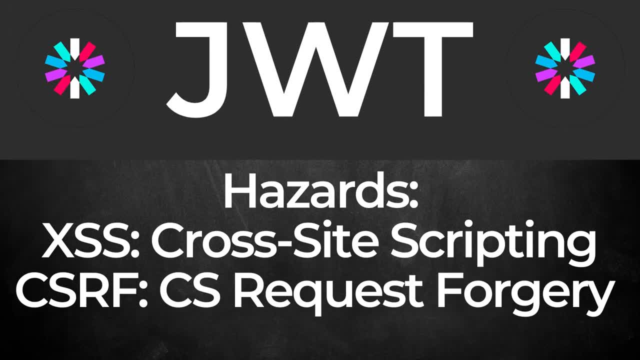 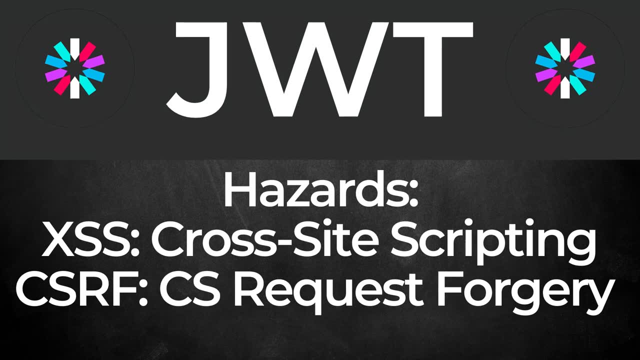 5 to 15 minutes And the refresh token is given a longer duration before it expires, possibly several hours a day or even days. While no security measures are perfect, we do want to consider the risks of cross-site scripting and cross-site request forgery. I will provide links about both in the 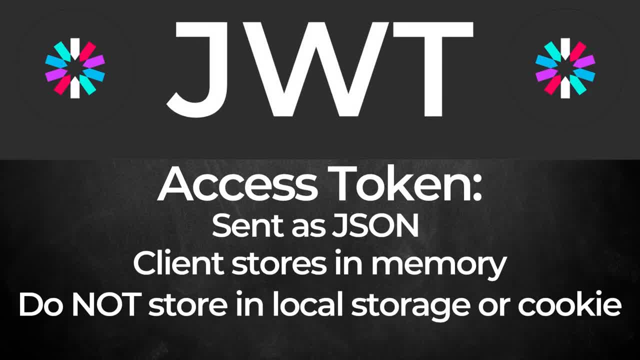 description below. Our API will send and receive access tokens as JSON data. To avoid the previously mentioned risks, it is recommended for front-end client applications to only store access tokens in memory, so they will be automatically lost when the app is closed. They should not be stored in. 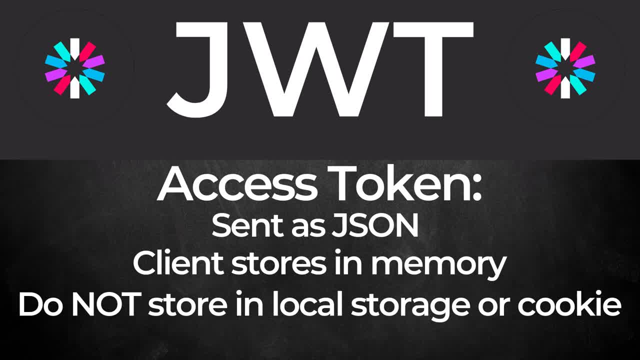 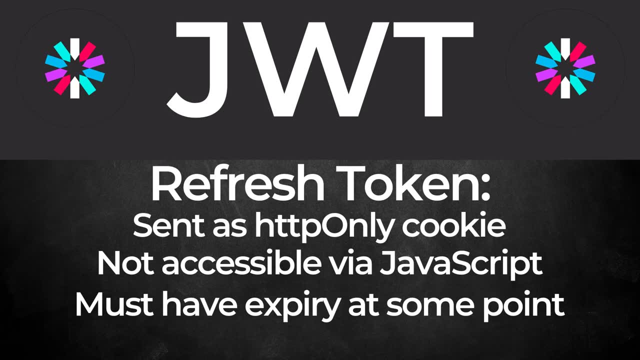 local storage or in a cookie. Essentially, if you can store it somewhere with JavaScript, a hacker can also retrieve it with JavaScript. Just keep access tokens in memory, which you might also refer to as the current application state. Our API will issue refresh tokens in an HTTP-only. 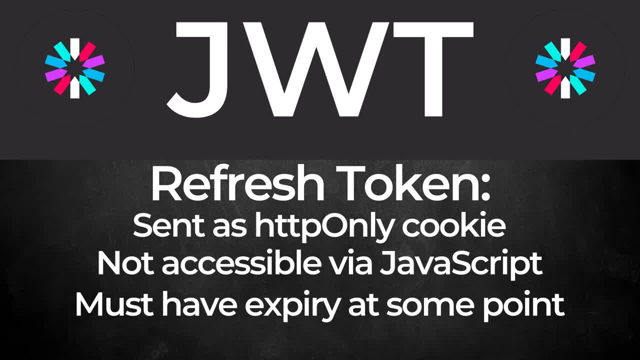 cookie. This type of cookie is not accessible with JavaScript. Refresh tokens do need to have an expiration, which will then require users to log in again. Refresh tokens should not have the ability to issue new refresh tokens, because that essentially grants indefinite access. 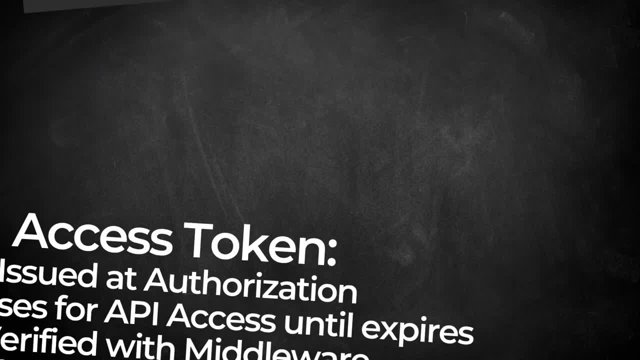 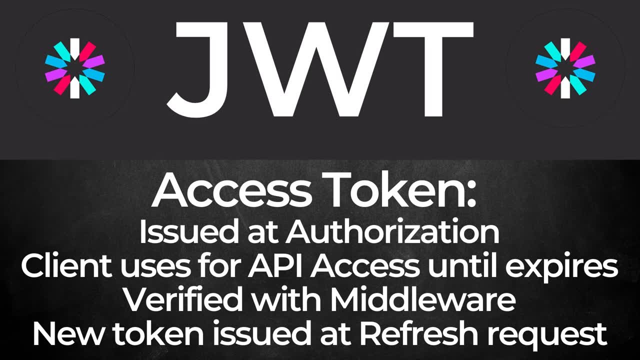 if a refresh token falls into the wrong hands. So the overall access token process involves issuing an access token during user authorization. The user's application can then access our REST API's protected routes with the access token until it expires. Our API will verify the access token. 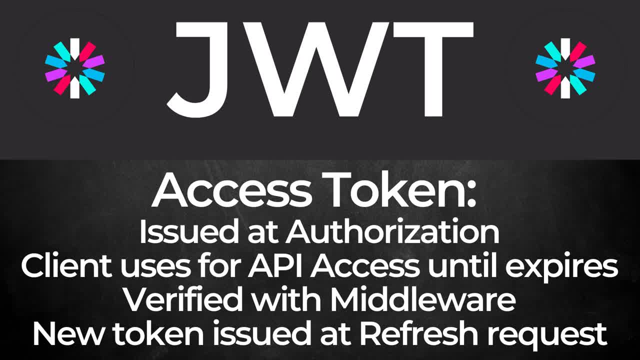 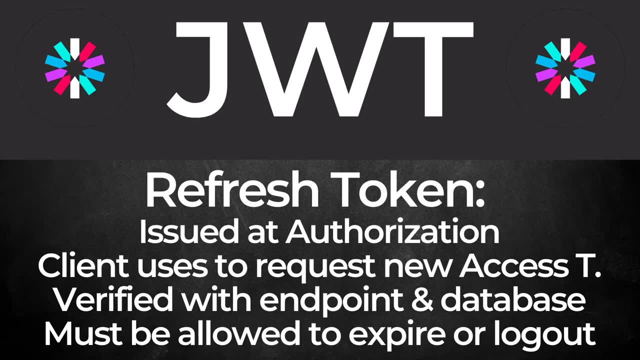 with middleware every time the access token is used to make a request. When the access token does expire, the user's application will need to send their refresh token to our API. Of course, the refresh token is also issued during user authorization. Our REST API's refresh. 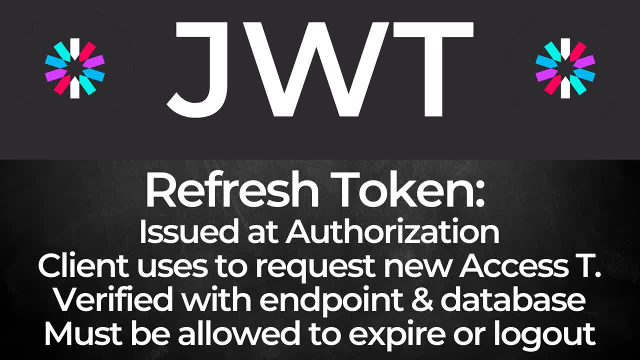 endpoint will verify the token and cross-reference the refresh token in our database too. Storing a reference to the refresh token in the database will allow refresh tokens to be terminated early. if the user decides to log out And again refresh tokens need to be allowed to. 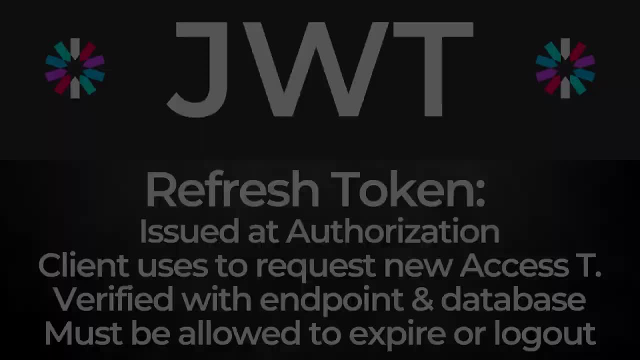 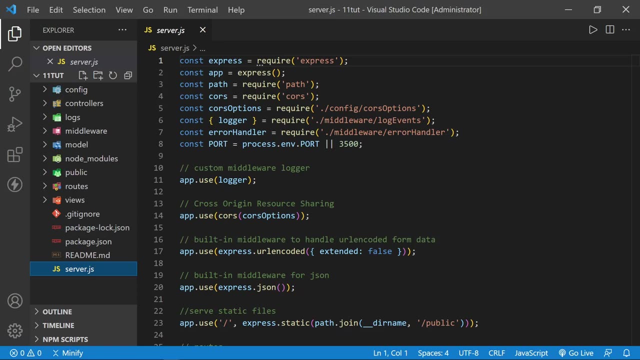 expire, so indefinite access cannot be gained. We're going to start with the code repository from the last tutorial, but if you don't have it, you should be able to easily follow along without it, or you can download or clone the starter source code from the link that I've provided in the description below. 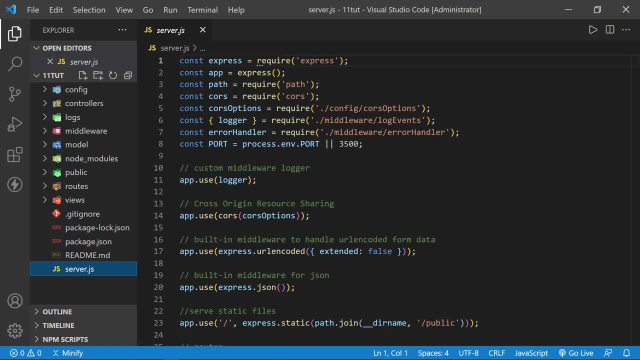 Let's get started today by installing the node packages that we're going to need. So I'm going to press control and the backtick. You could also go to the terminal menu and open a new terminal window. From there I'm going to type npm, i and then we can add all. 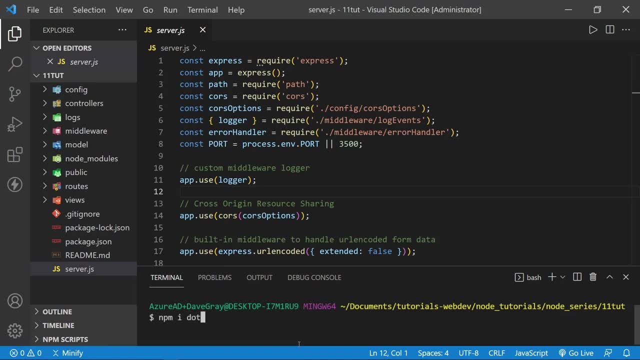 of the packages that we're going to need. So I'm going to type npm i and then we can add all of the packages that we need all on one line. So the first one is dot env, The next one is json web token, with no spaces there, And then the last one is cookie dash parser, And we'll 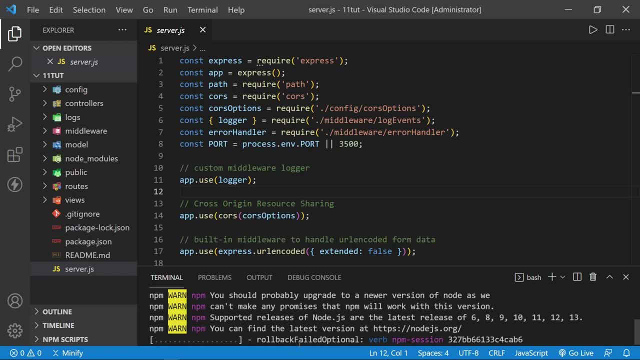 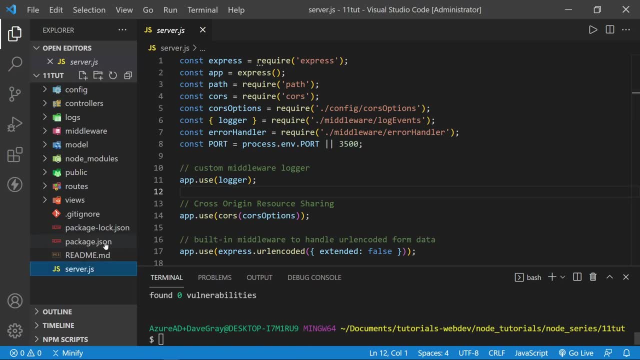 press enter and all of those packages will install. And then we'll check our package json just to make sure the dependencies have all been added. And that was fairly quick. Let's go ahead and look at the package dot json And we can see under our dependency. 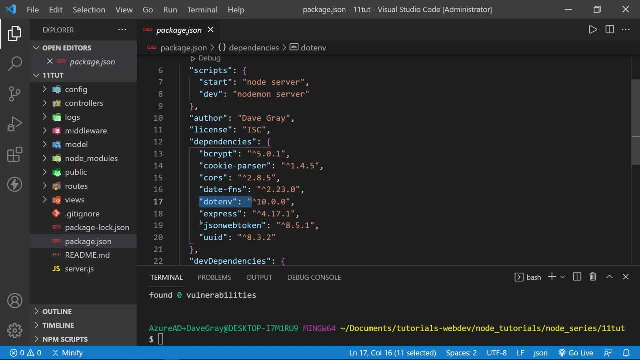 we've got the cookie parser, we've got dot env and we've got the json web token package. With that, complete, I'm going to close the terminal window And over in the file tree I'm going to create a new file at the root level And I'm going to name this dot env. 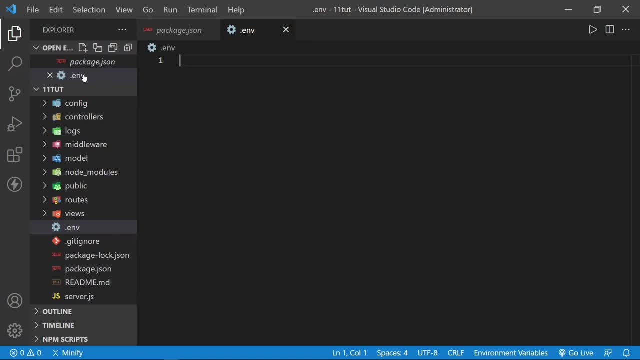 just like that. And now we can put our environment variables in here. I'm going to use all caps and type access, underscore, token, underscore secret, and set that to an env. And then I'm going to equals and then we'll get the value in a second, And then I'm just going to copy that down and 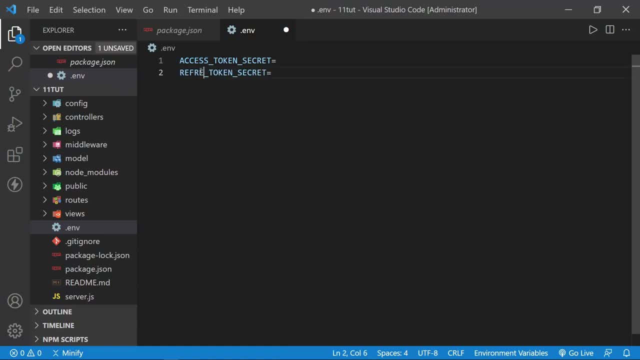 change the word access to refresh, because we're going to create an access token and a refresh token. So let's save this much for now. open the terminal window back up And now we can type node in the terminal to go into node And now we're running node at the command line interface. 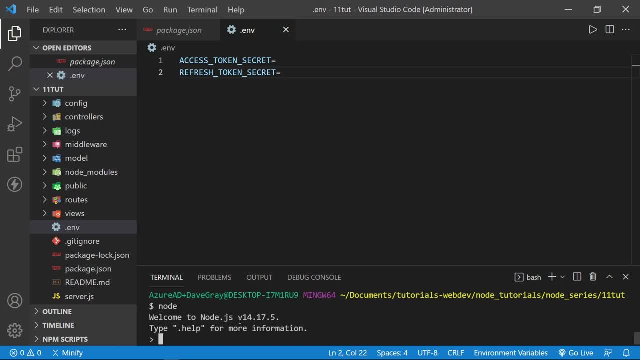 Node has a common core module called crypto. So right here at the command line we can type require And now we can put crypto in here, And from there we can add random bytes with camel case, with a capital, B, the number 64, and then dot to string and we'll say: hex. 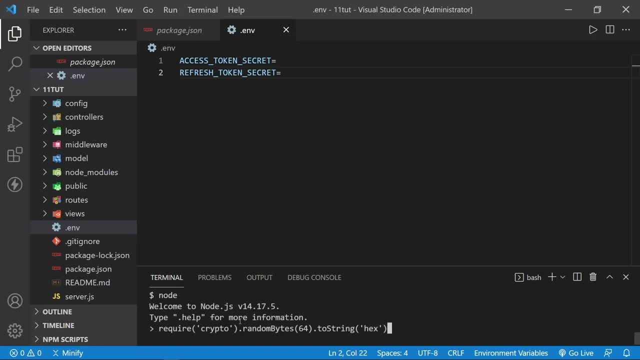 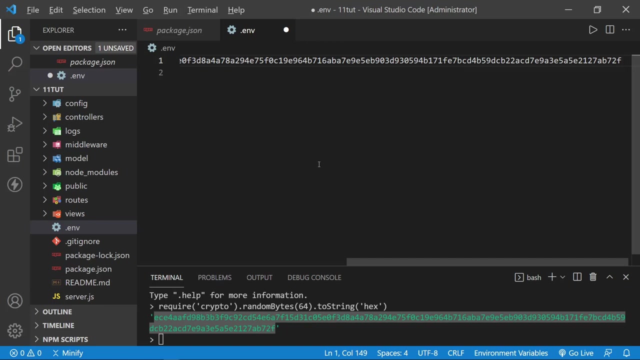 And this will give us a random crypto bytes string that we can use as our access token secret. So let's do this, And we don't need the quotes at all inside of our dot env. Now Ctrl C to copy And I'll just paste this in here as our access token secret, And I can press Alt Z in Visual Studio code. 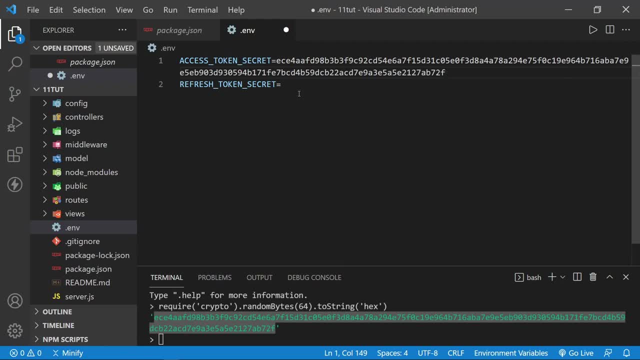 to get that to wrap so it doesn't go beyond the edge of the screen. So that is our full crypto line that we just created there. Now let's go ahead and create one more. I can press the up arrow in the command line just to pull that command back up. press enter And. 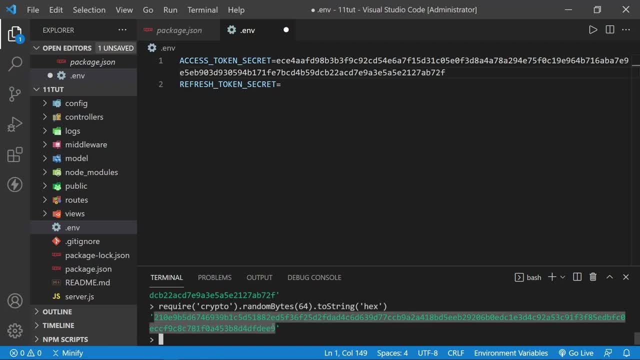 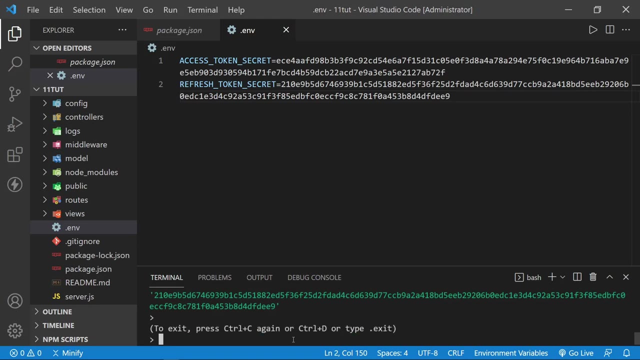 it generates another random crypto line here that we can copy and paste right into our dot env file And with that I'm going to press Ctrl S to save and close the terminal. Actually, I'm going to open the terminal back up real quick because we didn't exit node. we press Ctrl C and then 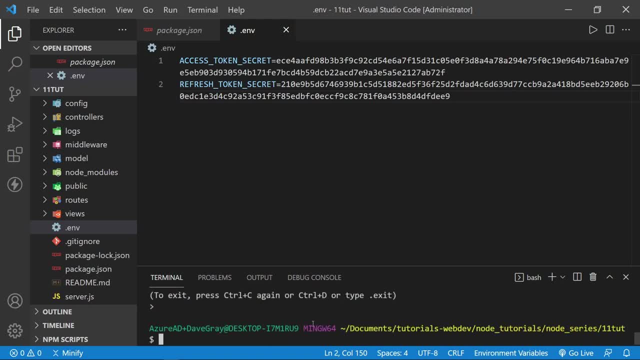 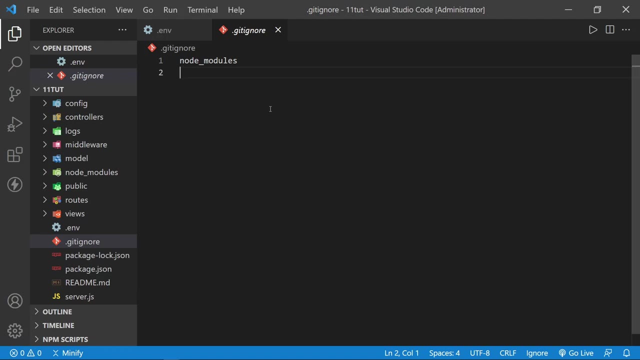 it says press Ctrl C again. So we press it again And now we have exited node at the command line. Now I'll close the terminal window. One other thing we want to do with the dot env file is make sure it has been added to our git ignore file. you do not want to send your environment variable values. 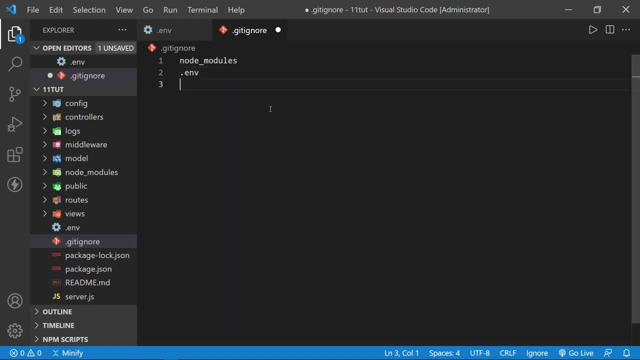 that you're storing in the dot env file. or you could just say: you do not want to send your dot env file to GitHub, you want to keep this in your dev environment And then when you host somewhere- whichever host you have- they should have a way to put the environment variables into their hosting. 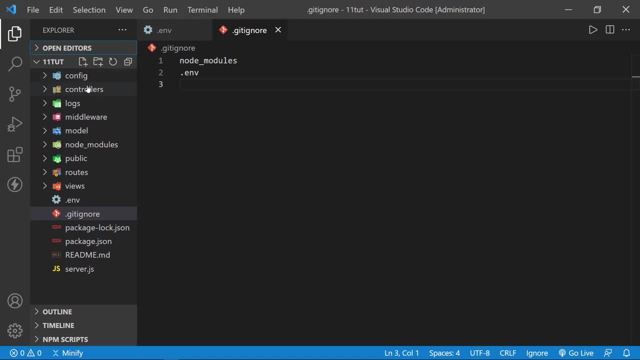 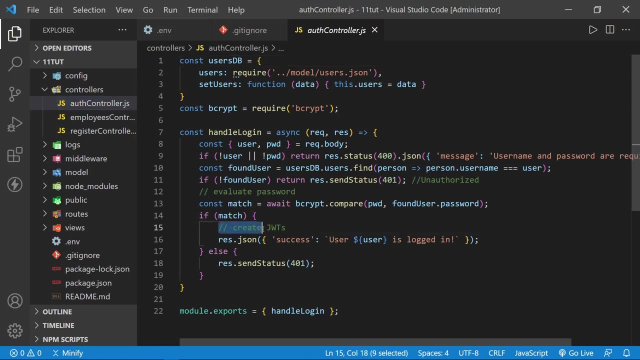 service, then you can pull those out. Now we need to go to our controller control and open up our auth controller that we've created in the last tutorial And we left a note for ourselves that this is where we want to create the JWTs on line 15.. Before we get started on line, 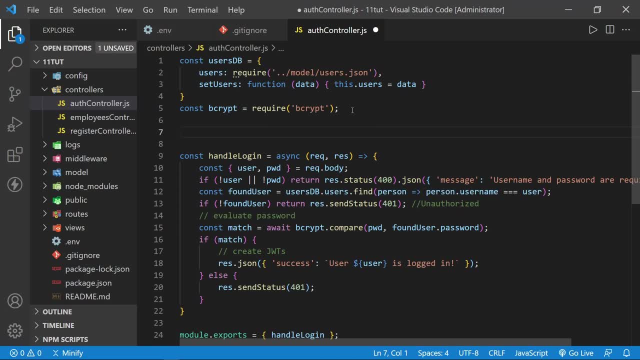 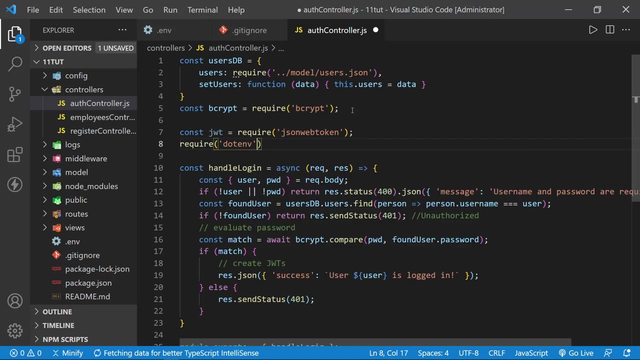 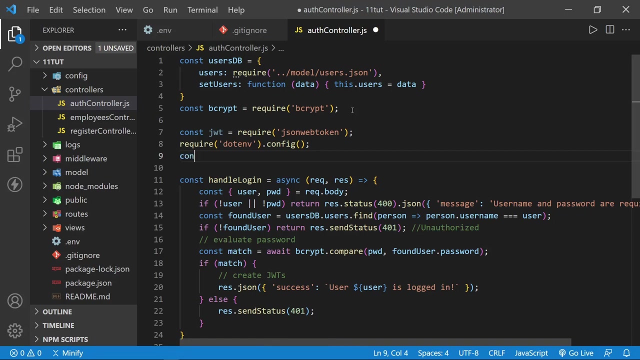 15,. let's go ahead and pull in everything we will require today. So let's define JWT, set that equal to require and then pull in our JSON web token package. After that we need to go ahead and require dot env, and then we need dot config after that, And after that we need our FS promises. 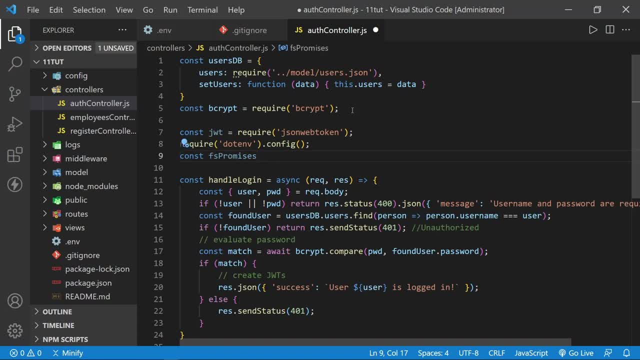 because we have not integrated Mongo or any other database technology yet, So we are still working with simple files and JSON values. So we need this FS promises and we'll set that equal to the FS module, And after that we need dot promises. 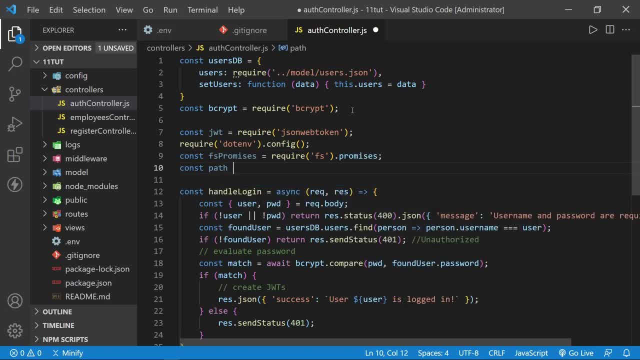 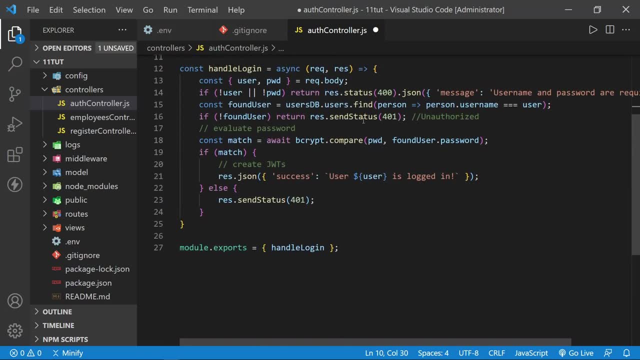 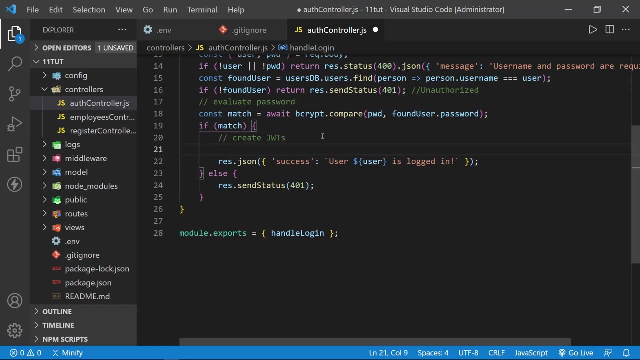 and then, finally, we need the path module and we'll set that equal to path. now let's scroll down so we have just a little more room to work on the screen and we're back here and now. line 15 turned into line 20, where we're creating our JWTs and let's define our 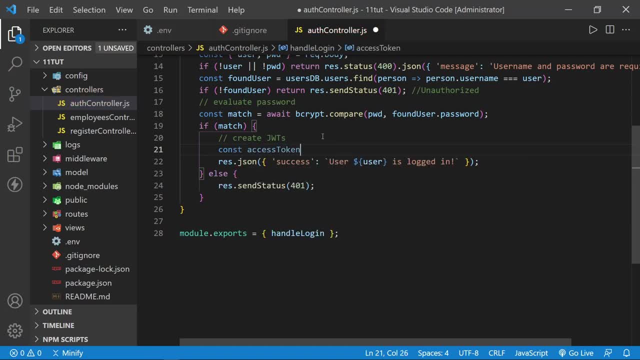 access token. we use camel case with a capital t on token and we'll set this equal to JWT dot sign. the first thing we need to pass into the JWT is a payload, so what we're going to use is our username object: you don't want to pass in anything like a password or anything that would. 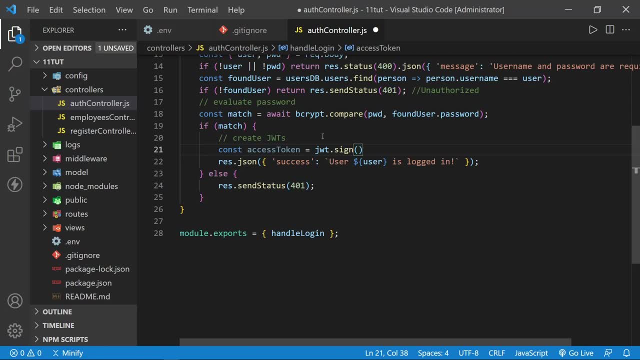 otherwise hurt your security, because this is available to all if they get a hold of your token. so what we want to pass in is just the username. I'm going to do this on a separate line, and so we'll create this object with you username and here above we had a found user and then we can say username. now this is coming. 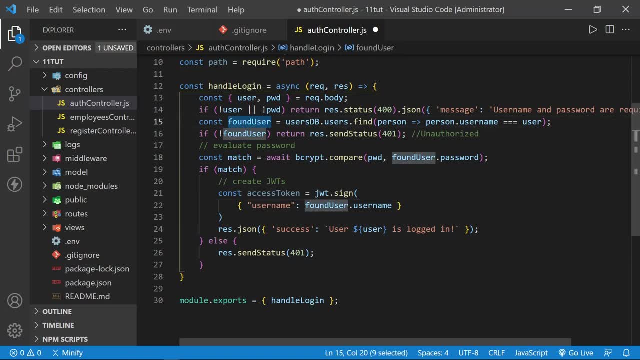 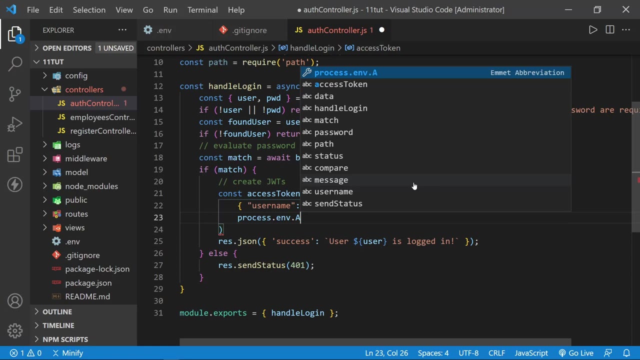 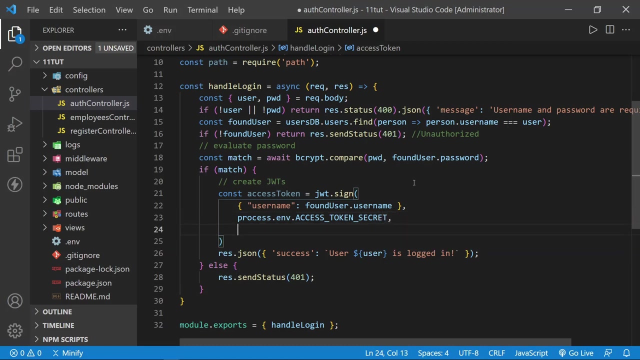 from up here where we found the user that was logging in. after that, the second thing we need to create our access token is our secret that we defined in the dot env file, so we access this by process: dot env. dot access token, underscore secret and then, finally, what we need is an options value here and we can say when this token 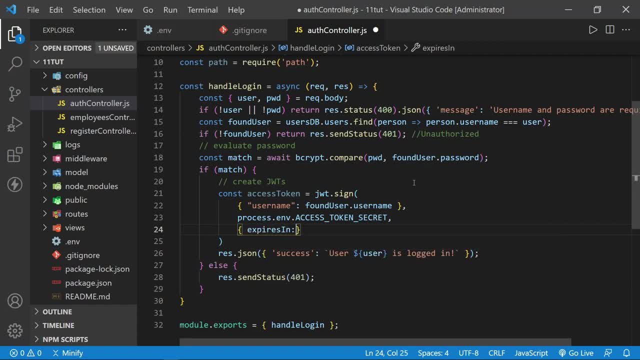 expires- and this is camel case- expires in and we're going to make this very short for this tutorial. that will allow me to show the token expiring and see what happens. but what you might want to do in production would be maybe 5 minutes or 15 minutes, some small window of time, but 30. 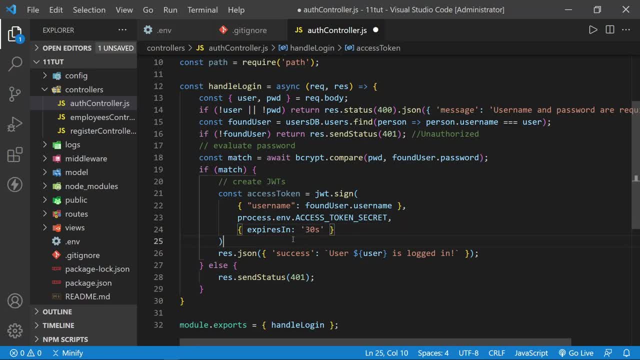 seconds might be too short, and you could have done a little bit less of that if you were doing your�. it is all a preference, though, And, with that defined, let's go ahead and highlight all of this, and then I'll just press Shift, Alt and the down arrow. 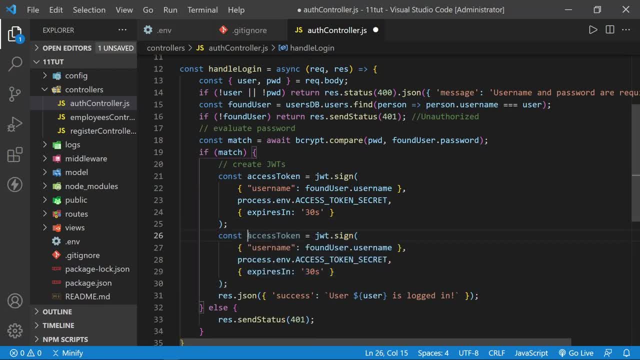 to copy it all down and we'll just make a few changes to go ahead and create our refresh token as well. So I'm going to type refresh here instead of access. We're once again going to pass in the username, but then we need the refresh token secret. 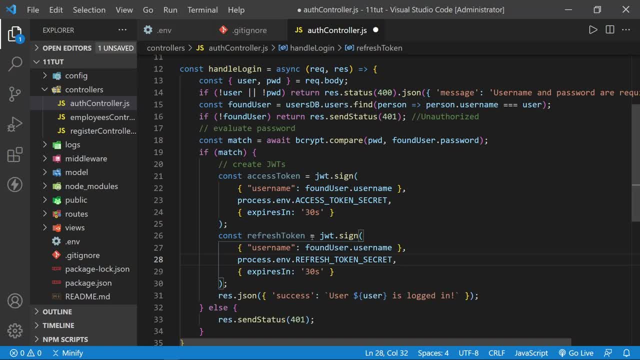 And now our refresh token needs to last much longer than the access token, but you do want it to expire at some point, And so I'm going to make this one day, and I'm going to give a link to the package, the JSON web token package on npmjs. 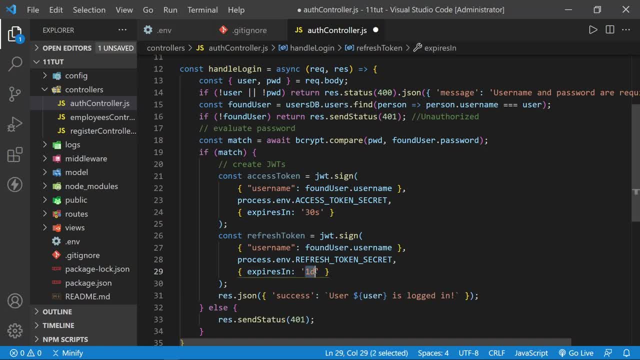 And there you can see another link and more documentation on the different values you could put in here. But one day is what we're going for And then we want it to expire and we want our users to have to log back in. You could make an indefinite refresh token. 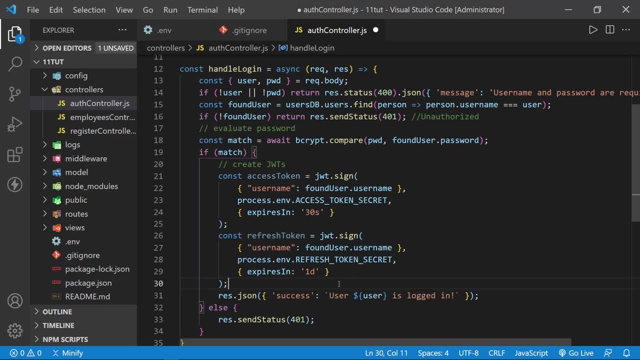 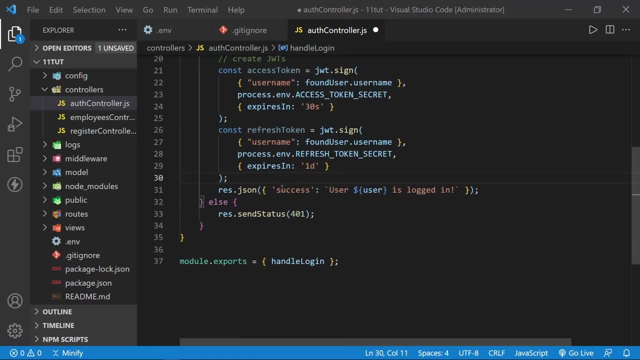 but that means if someone gets a hold of it and they're not the correct person, they will always have access And you do not want that. With both tokens created- I'm going to scroll up for a little more room again- and we want to save our refresh token in the database. 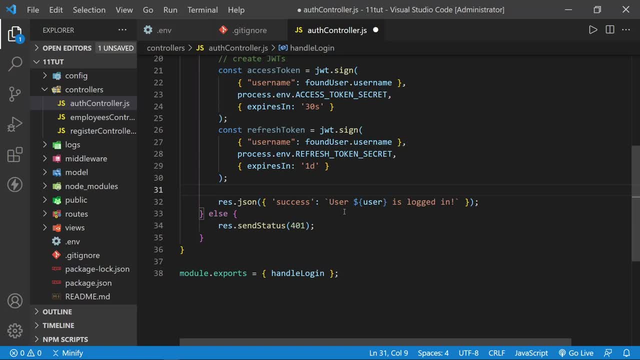 which will also allow us to create a logout route in the future that will allow us to invalidate the refresh token when a user logs out. So let's start by doing that And, once again, we're just working with our JSON files for now and we haven't connected this. 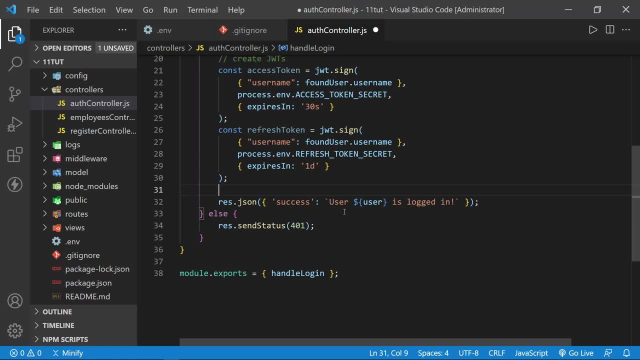 to an actual database. that we will do in future tutorials. But of course that lets us modulize these tutorials And then we can attack, say Mongo, or go over to Postgres or anything we want to in separate tutorials. So for now just the JSON file. 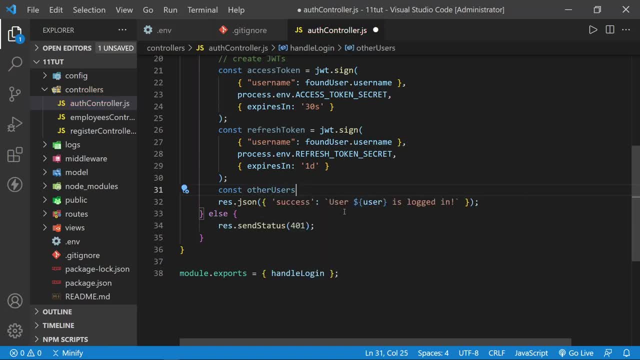 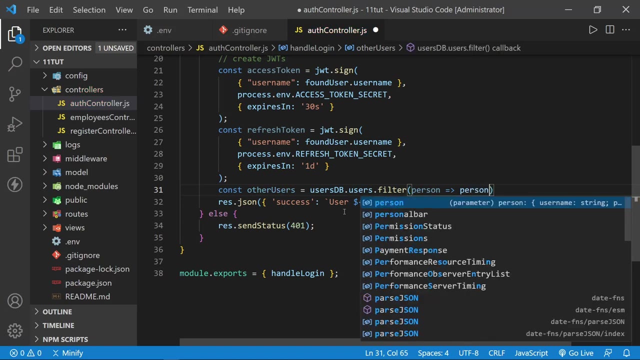 And I'm going to define other users. We had a found user, so now we'll set other users equal to the usersdbusersfilter, And now for each person that we have, we're going to say personusername not equal to, and now let's have that not equal to. 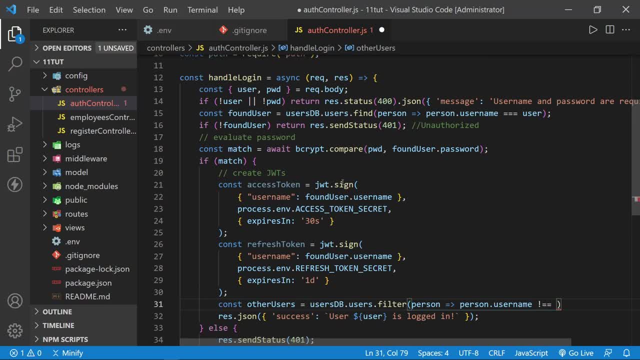 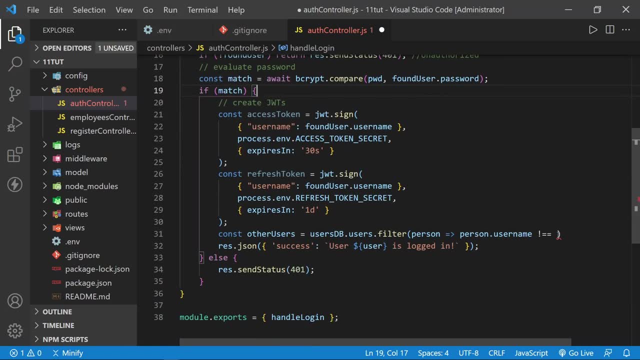 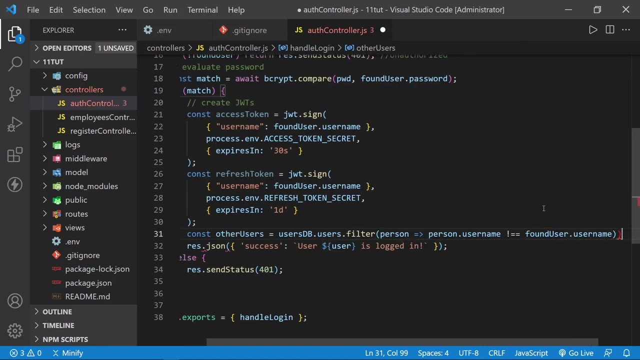 I believe it was the user that we came in with the request right here. However, we also have our found userusername and I believe I'd like to use that, since we have found it. So let's say founduserusername, and now that creates an array of the other users. 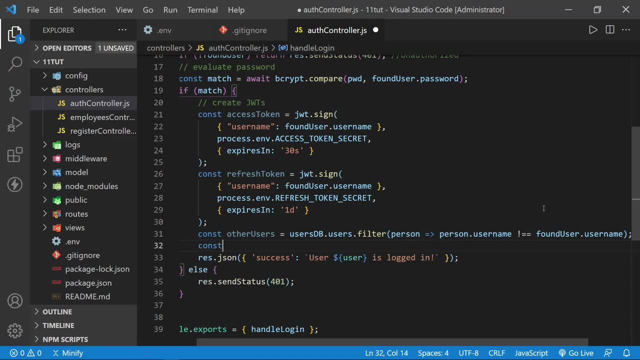 that are not the username that is logged in. And now let's create a current user. We're going to set this current user equal to the found user And then we're also going to add in the refresh token that will be saved with this current user. 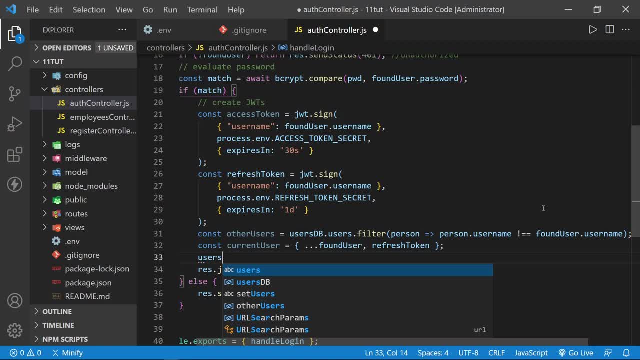 And now let's set our users once again and we can say users, dbsetUsers, and in this new array we'll go ahead and add the other users and then we'll add the current user that we just created. I really don't know why I'm putting spaces there. 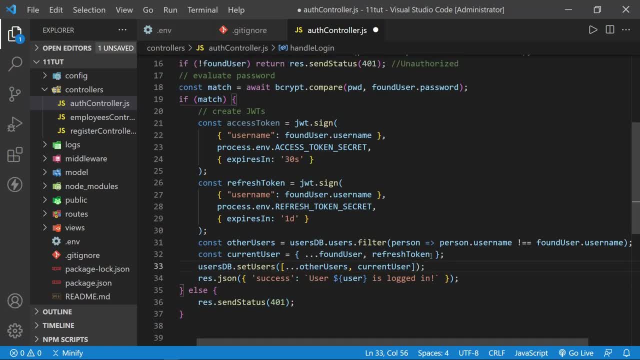 Really don't usually do that in an array. And okay, let's go ahead and put the semicolon and let's write our new users file. This would be await, and then fspromiseswriteFile, and I'll go down to a separate line. 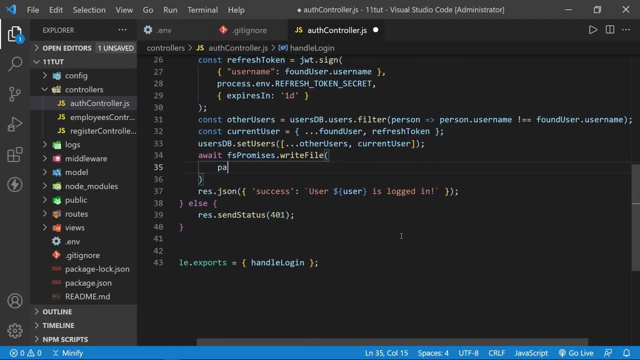 I'm going to scroll up once again just to put that in the middle. Say, pathjoin, We'll pull in the directory name. Then we need to go up one directory and then we need to go into the model directory and then we need to go ahead and name this usersjson. 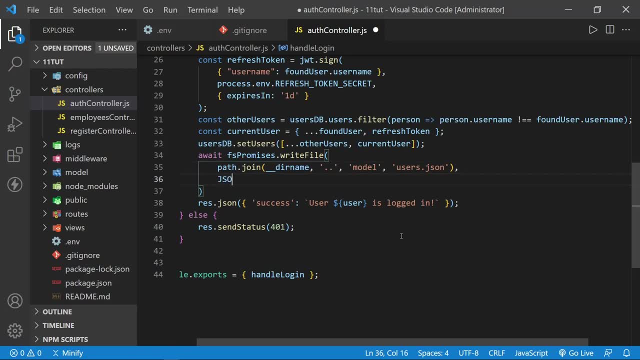 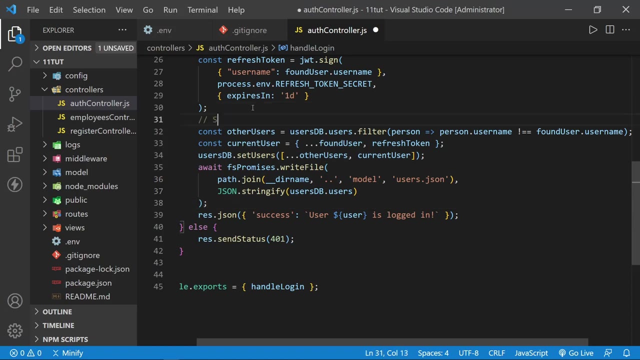 as our users file is After that what we want to put in. we need to JSON, stringify and pass in usersdbusers, which will write our new users file, and so I should have put a little comment here at the top. This is saving refresh token with current user. 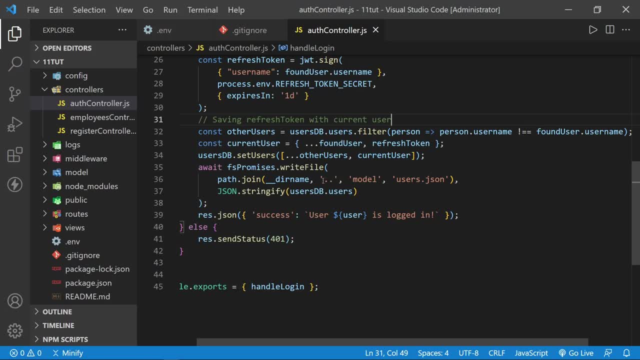 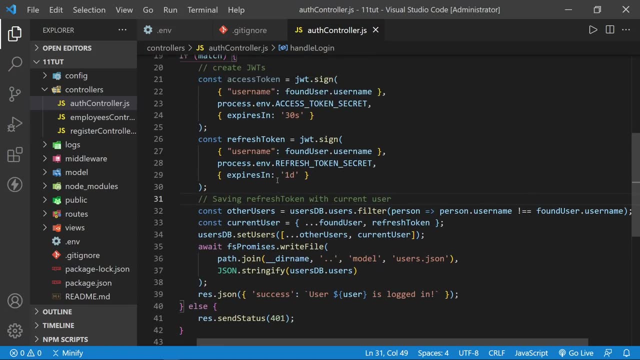 which, again doing this, will allow us to invalidate that refresh token as the current user logs out, which, again doing this, will allow us to invalidate that refresh token as the current user logs out out if they log out before their one day has expired. So, as a quick review, we have created 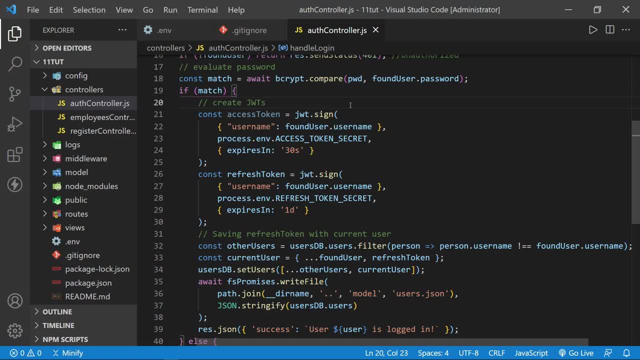 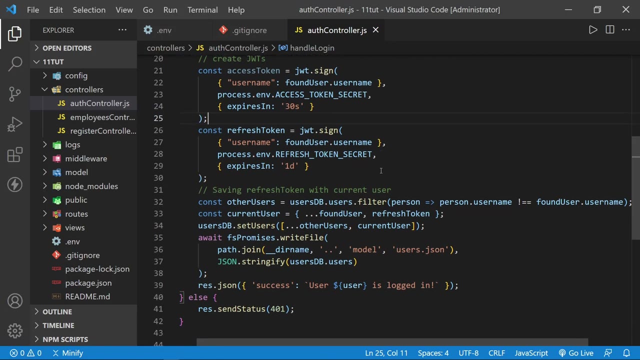 the JWTs once we have authorized the login, which was with bcrypt in the previous tutorial. But now that we authorize the login, we create the JWTs. we have a refresh token that's being saved into the online database and an access token, And yet we still need to send both: the refresh token. 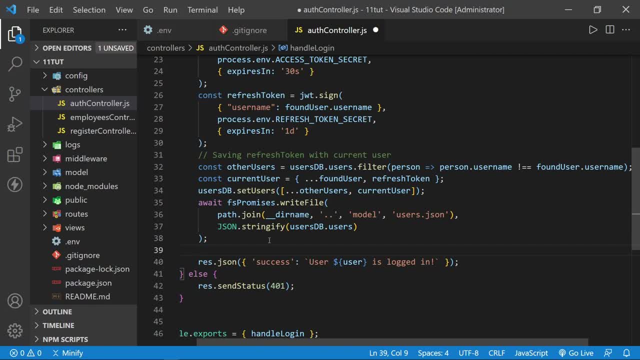 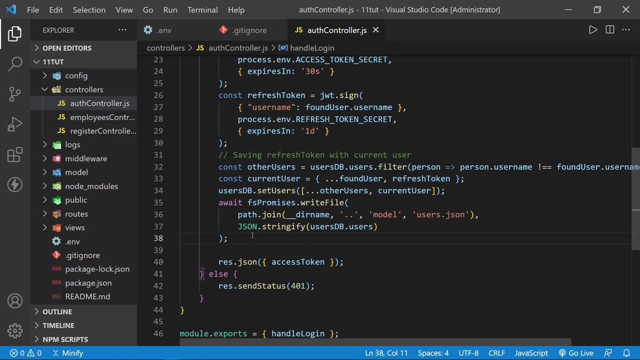 and the access token to the user. The easy part of this is to just remove what we were sending in our JSON and instead send the access token. We can send that as JSON and on the front end, the front end developer, or as a full stack developer if you're developing the back end and the front end. 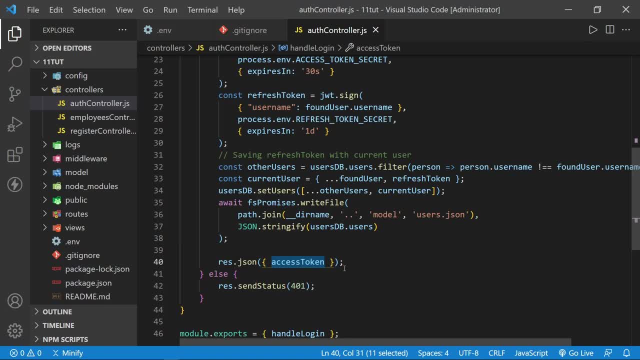 you really want to store this access token in memory. It's not secure in local storage and any cookie that you can't access with JavaScript could also be accessed. So anything that really that JavaScript can access where you would store it it's not really that secure. So if you store the access token in memory, 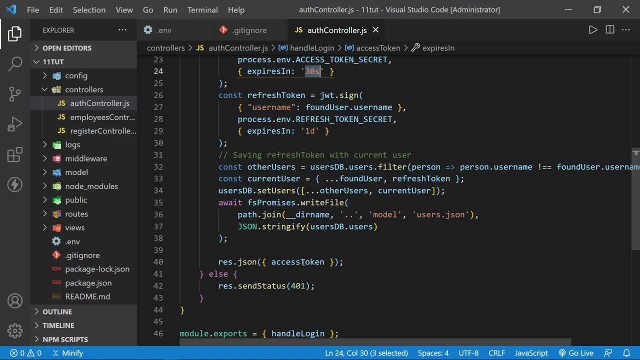 which has a very short lifespan. we only gave it 30 seconds here but, like I said, maybe you'd give it 15 minutes. By keeping that in memory, you're not storing it anywhere vulnerable. After that, the refresh token: what we're going to do. I've definitely seen tutorials that also just send it. 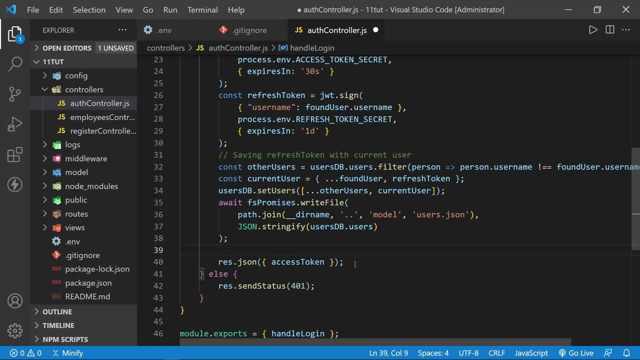 along in the JSON. But that kind of creates a dilemma for the front end developer or as you develop the front end, because you do need to store the refresh token. We want to send it as a cookie And I know I said a cookie could be vulnerable to JavaScript. but if we set the cookie as HTTP only, 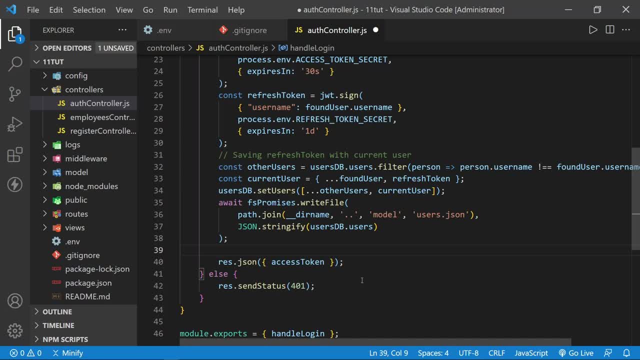 it is not available to JavaScript. So that's what we want to do. So let's say rescookie. And now here we can name the cookie. I'll just name it JWT. From there, we want to pass in our refresh token And after that we want to give options. 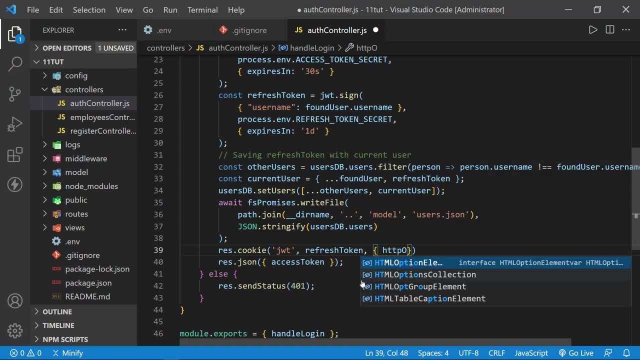 And the first option. I'll give a space here. HTTP only Set that to true, And after that we want to set a max age. Here we go, And now I'm going to set this to 24, which would be 24 hours 60 times 60 times 1000.. And this is in milliseconds here. So what we're? 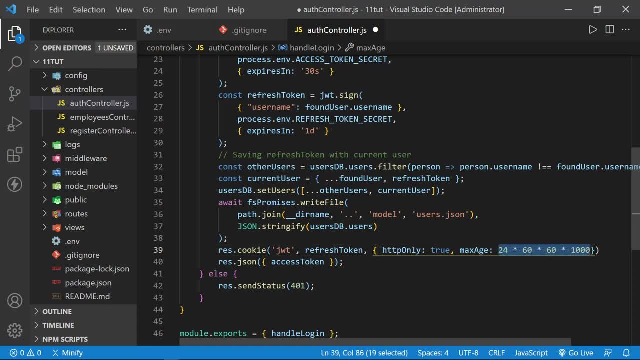 really getting is one day. That's what that is equal to, as we set the max age of the cookie- And I'll go ahead and cap that off here- You could set it for longer as well. Now, cookie is always sent with every request, But the nice thing about an HTTP only cookie is: 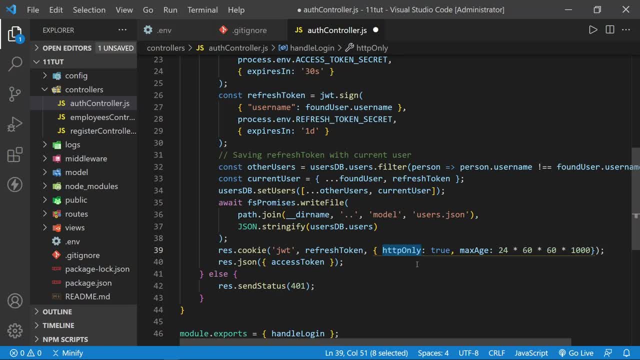 that it is not available to JavaScript And while it's not 100% secure, it's much more secure than storing your refresh token in local storage or in another cookie that is available to JavaScript. So let's save this, And now we know we are sending our 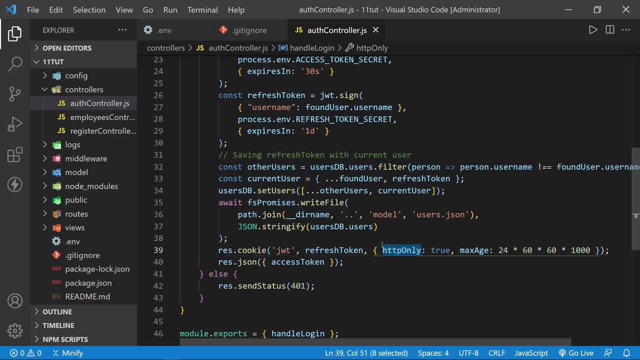 refresh cookie that is HTTP only- to the user. We're also sending the access token. Oh, here we're sending our refresh token. is what I meant to say in a cookie that is HTTP only. We're also sending the access token as JSON that the front end developer can grab. 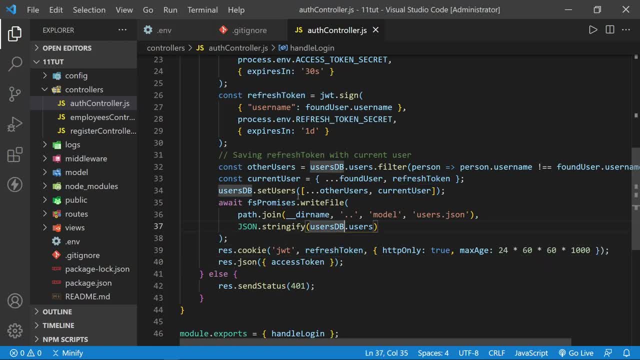 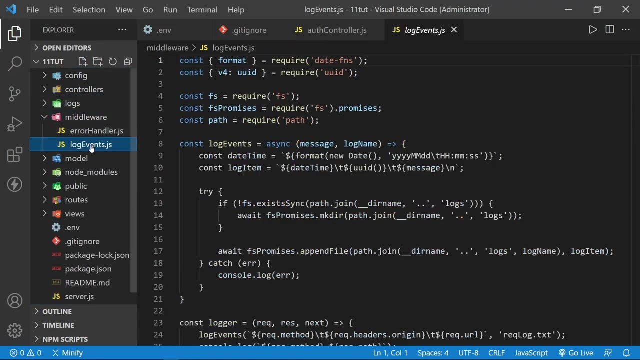 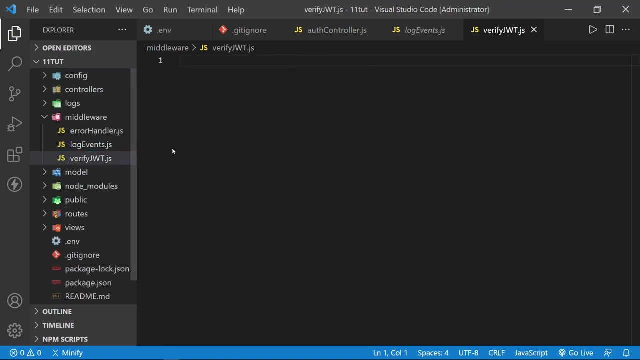 And we're also storing the same refresh token in a database here that can be be cross referenced when it is sent back to create another access token With our auth controller complete. let's now go look at the middleware folder And we need to create a new middleware file here And let's call this: verify JWT dot JS And we're going to need 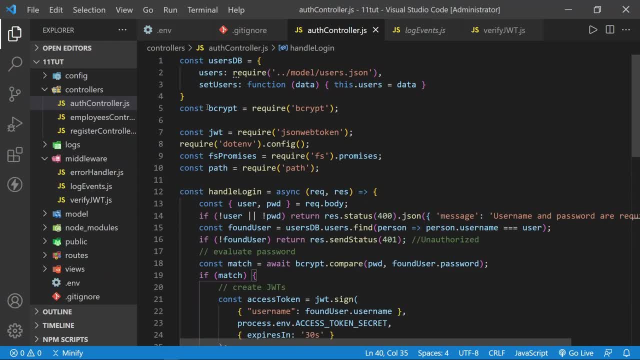 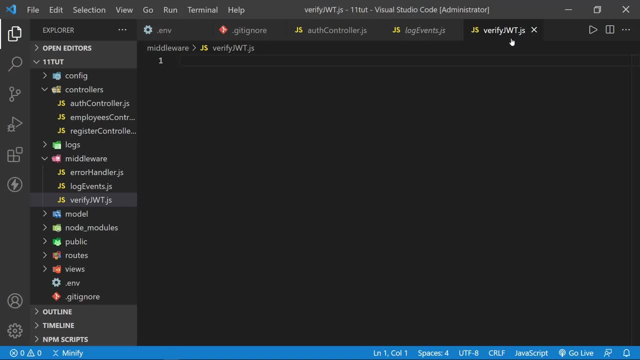 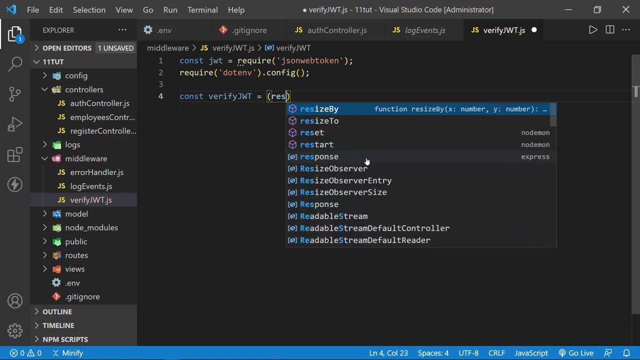 JWT and dot ENV once again in this file. So I'm back in the auth controller just long enough to copy these two And then go back to the verify JWT dot JS And I'll paste in our required packages right at the top. After that I'm going to create verify JWT. set this equal to a function that has a request. 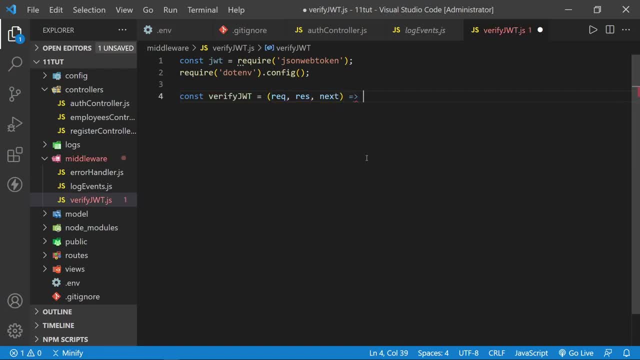 response. and next, as middleware should, And now let's define the auth header at the very top, And this is going to be equal to request dot headers. Oh, and then we need a bracket, not a dot, and then authorization, And of course we need to check to see if that is actually received. So now we can say if. 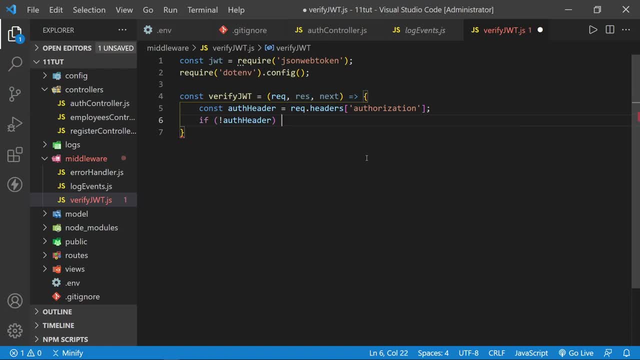 no auth header. We're going to send a response which we need to return, and then just send the status 401, which stands for unauthorized. After that, I'm going to go ahead and put a console log statement to just go ahead and log the auth header for the. 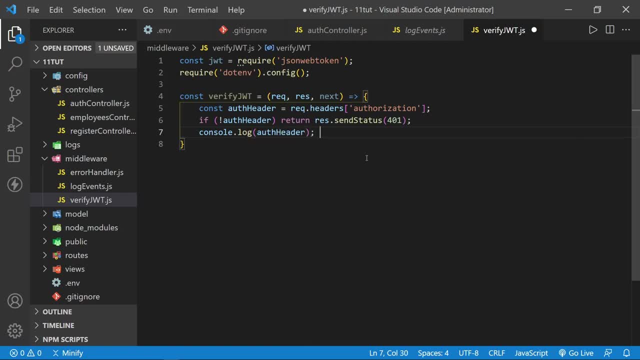 aprender or for when we test this. we'll be able to see that in the console you'll see a line that looks like this And it will say best, and there will be a space and then there will be the token after that. 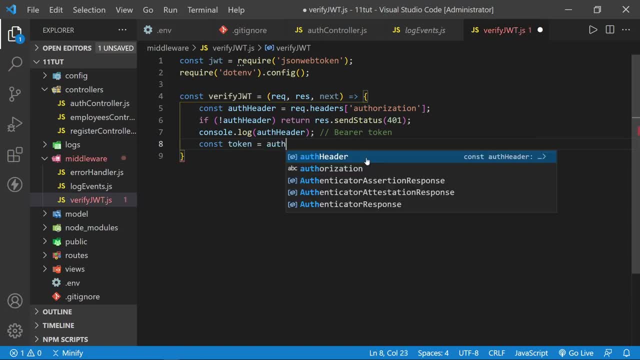 So we can define our token now and we can set this equal to the off header And then we can call split on that space that I just described And we'll put the space in here on the split, and then we need the tokens. 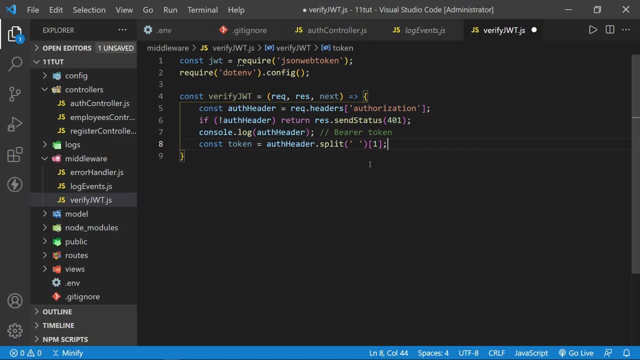 So it wouldn't be in the zero position, the one position after that. and now we can verify the token with jwt dot verify and here we'll pass in the token first. after the token we'll pull back in our secret and this will be the access. 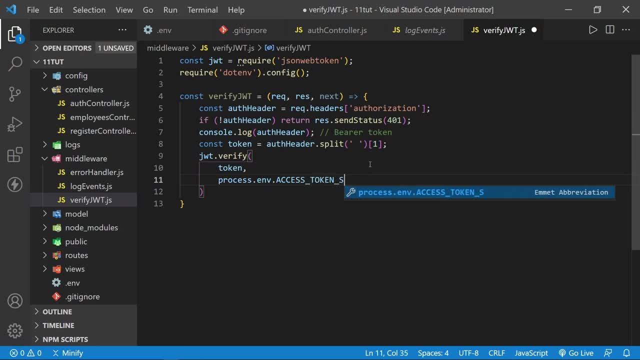 token secret, because that's what we'll verify with this middleware. and after the access token secret, there will be a callback that gets an error and then we'll call this. you could call it token if you want. we'll call it decoded, because it will have decoded. 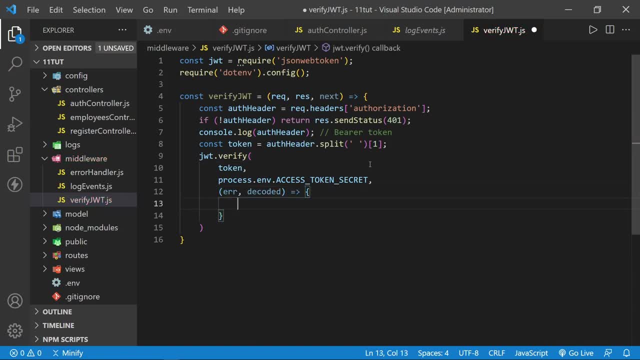 information from the jwt, and now we'll say: if we have an error, let's go ahead and return and send a status once again. this status will be 403, forbidden, because at this point we'll know we received a token, but something about it wasn't right. in other words, it may have been tampered. 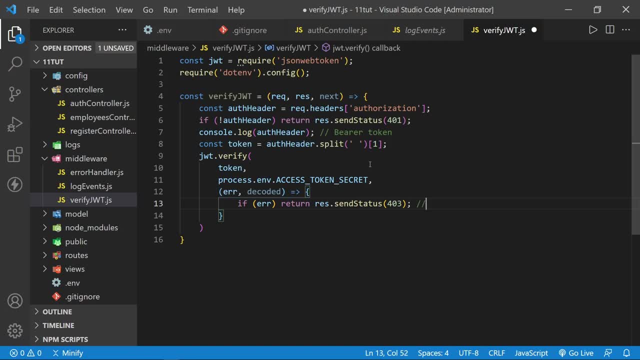 with, and so this means we have a invalid token. so we'll send a 403 instead of a 401, which means you are forbidden from accessing this, and then we'll set the user equal to decoded dot username. remember we passed in the username to the jwt, so now it's been decoded and we can read that, and then we'll call next from our middleware. 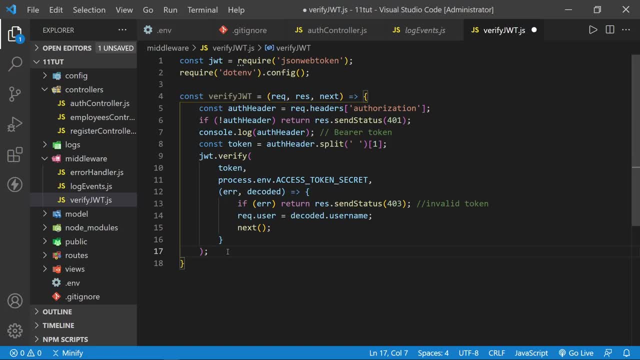 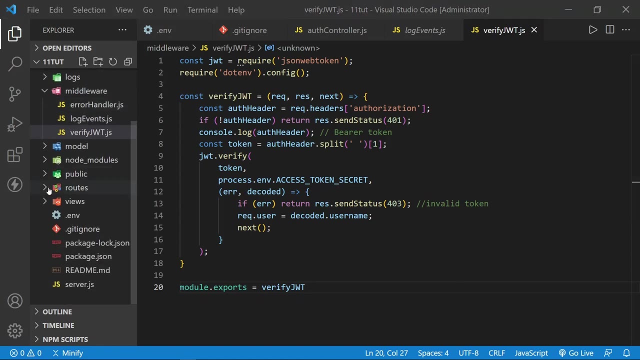 and that pretty much wraps up that whole middleware function right there. except we need to remember to export it. so we'll say module dot exports, set that equal to verify jwt and save. with the middleware now complete, we can add it to a route or routes that we 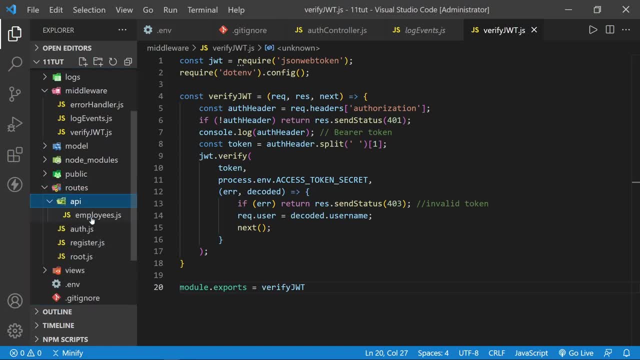 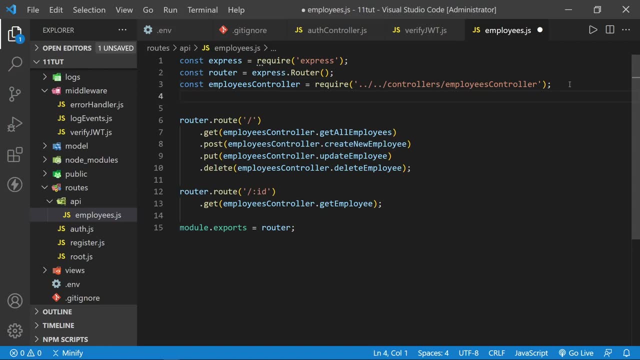 want to protect. so let's open up routes and api and go to our employees js file that has all of the employee routes in it and we need to import that middleware here. so we'll say: const verify jwt, jwt equals require. and now we need to go up out of the api folder, up out of the next folder, the. 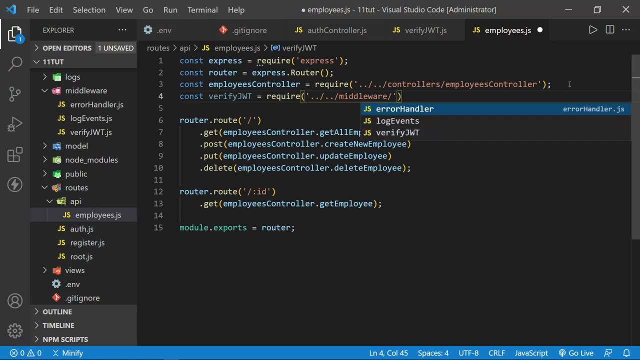 routes folder and then go to middleware and then choose verify jwt and once we have that we can just put it, let's say, in our git route- if we only wanted it in the git route before we call the controller. and so it will go through the middleware first and then go to the employees. 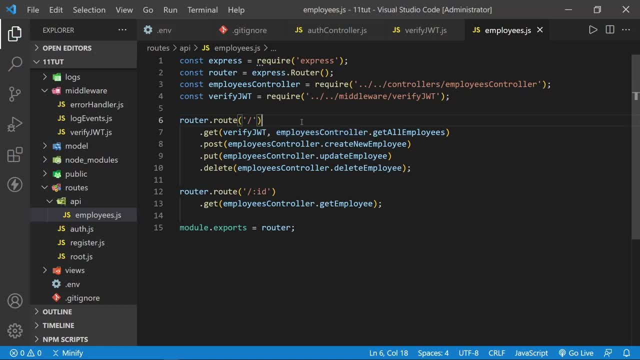 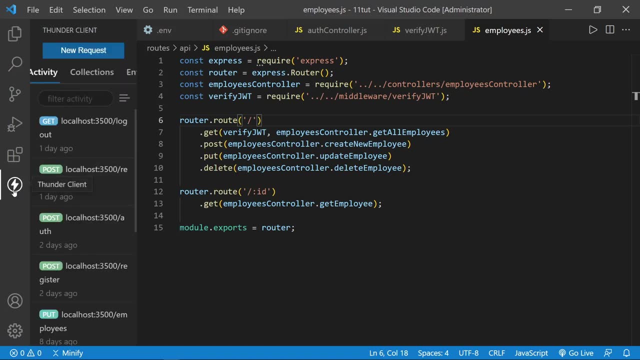 controller here. so let's save this and now let's test this with thunderclient. so over here to the left, i'll open up thunderclient and we're going to need to log in first. so i'll go to our collections and i have an auth collection that i created and i want to go to the auth route. i'll click this and 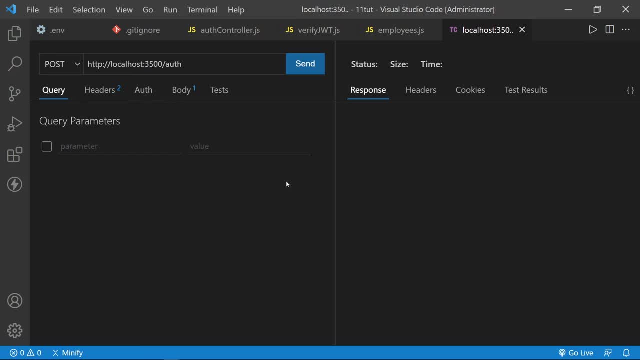 now i'm going to click over here again to hide the tree so we can see better. you and i'm also going to press control and back tick to open our terminal window. we haven't started the server yet, so that's something else we need. so we need to type. 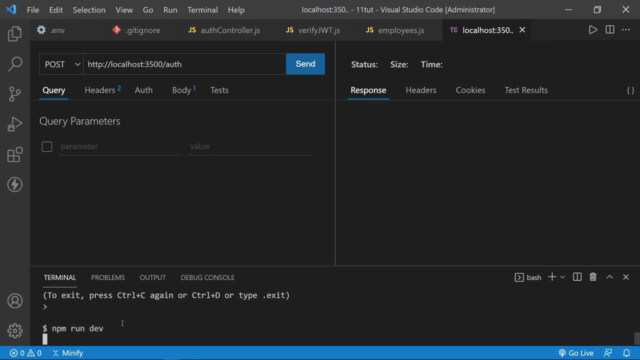 npm run dev to go ahead and start our server and it's running on port 3500, and so you can see the route we're going to go to is a post route. it's localhost 3500 off that we had previously set up to log in with the password. 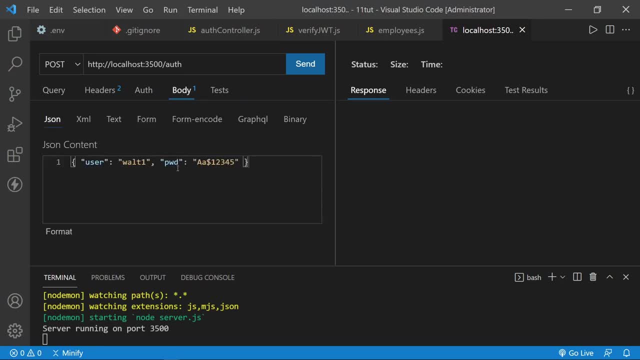 so in the body, we're sending walt one and password and the password that we had in there previously and this is in the users file that i have. if you haven't done this, you need to go ahead and either create this in the file or use the register route that we previously created and create a new user. 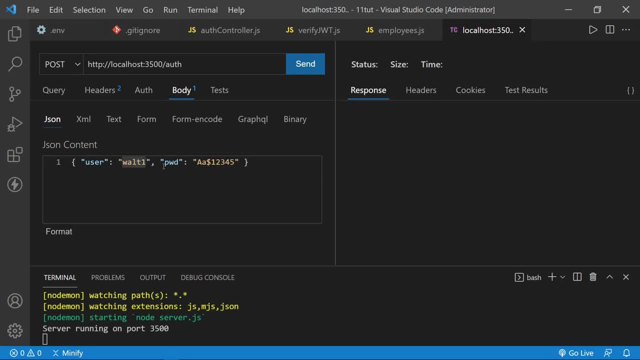 and then this will work. but we're right now we're going to log in with user walt one and this password using this route. so i'll go ahead and send and you can see over here on the right. the response we get is a 200. 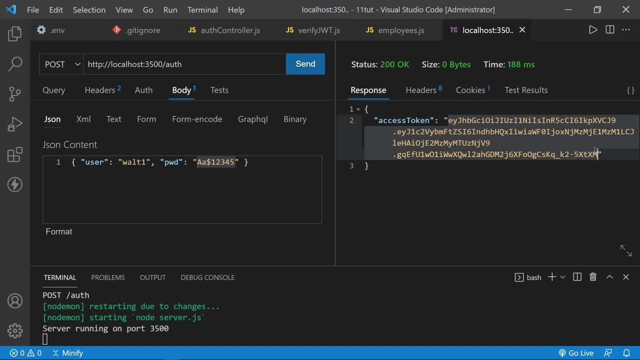 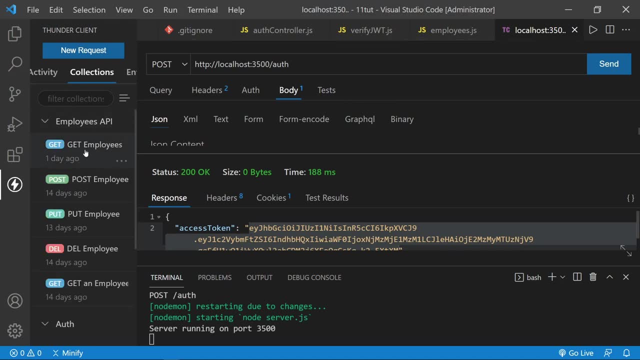 and we get this access token. this access token will only be good for 30 seconds, though, so let's see if i'm fast enough to come back here to our collections, open the employees, api, and now let's look at this, and i need to go ahead and, in our 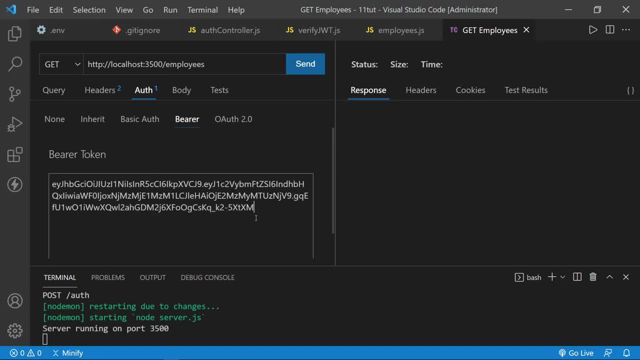 auth. i need to send a new access token. now we can send and we got our employees back, but this will expire. and notice down here: we also got the console log statement i put in here's bearer and then the space and then the token. so now, if i send this again, the token should have expired. 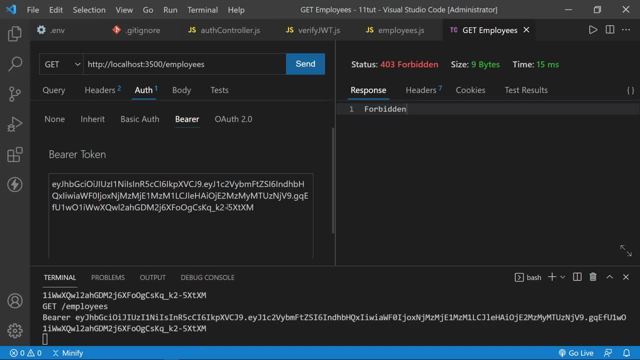 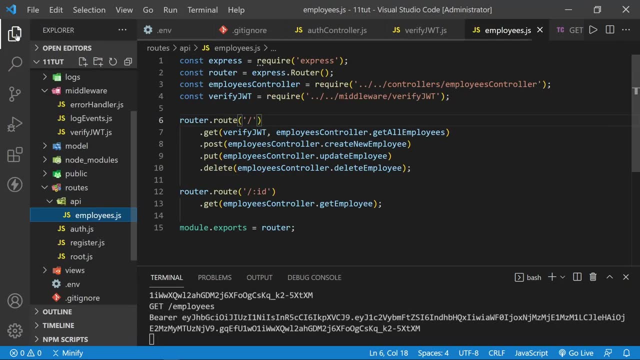 and now we get the 403 forbidden because the access token that we sent was only good for 30 seconds. now let's look at the employeesjs file again and i will go ahead and click the file tree so we can see our files. also, we're only applying this verified jwt middleware to the git route right now, and this is a good way. 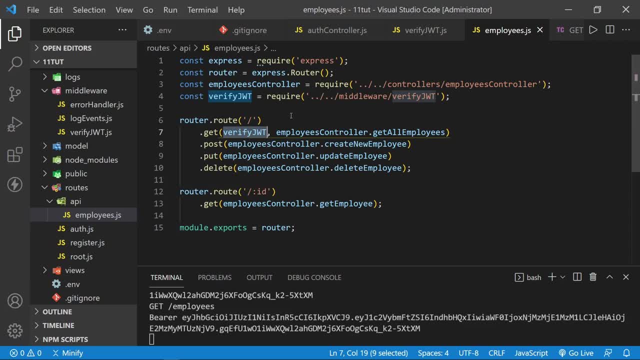 to do this if you have select routes that you want to protect or verify, but not all of them. however, if you know you want to protect all of the routes in your api, there is an easier way to do this, so let's go ahead and remove this and we'll pull this out of here. 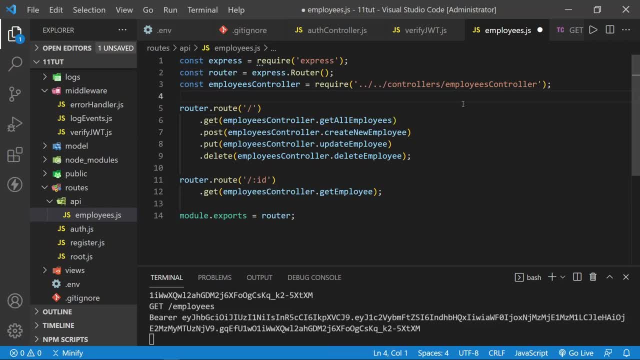 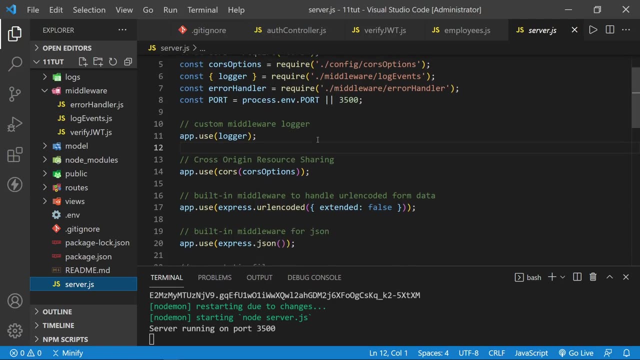 as well, and i don't think we'll just retype it in the server file, because that's where we're headed next. so we've removed the verify jwt from the employeesjs file altogether. let's go to serverjs, our main file, and here we can just pull this middleware in. so i'm going to do it right. 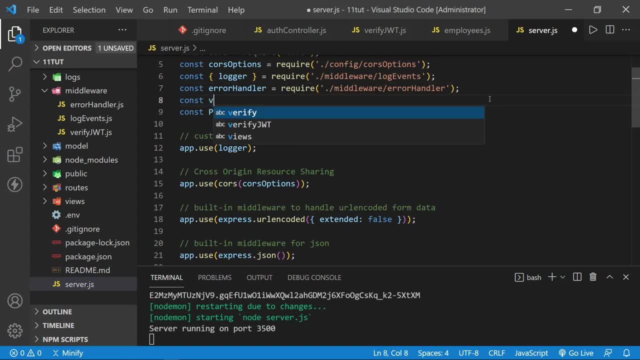 underneath the error handler that we had middleware for. so we'll say: verify jwt, set this equal to jwt-verify-jwt and here we want to go into. we don't need to go up at all, actually, we just want to go into dot slash, middleware, slash, verify jwt and now that we have that we can use this just. 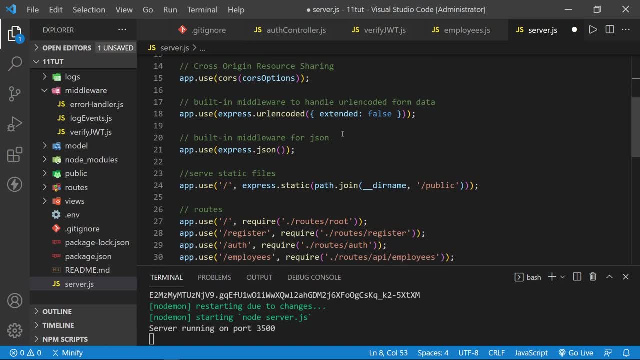 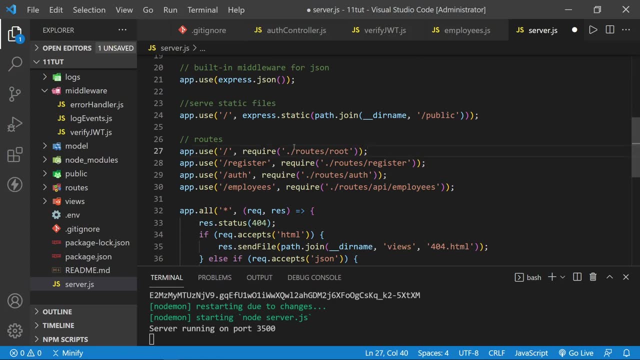 like. we've used other middleware in our file, but we probably don't want to use this verified jwt middleware for all the routes- probably not the route that we have here- definitely not to register a new user or we'd never be able to register in the first place and not even to auth, because they have to visit auth first to get the token. 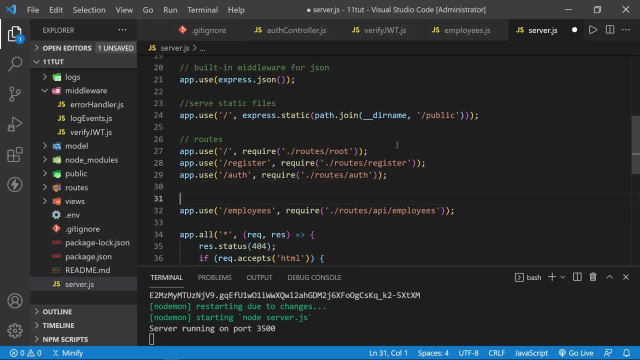 but we do want to put it before the employees route, so i'll put an extra line there and then right here we'll say: use verify jwt and if you remember, this works like a waterfall. so in this order, everything after this line will use the verified jwt middleware. so any route, we do not. 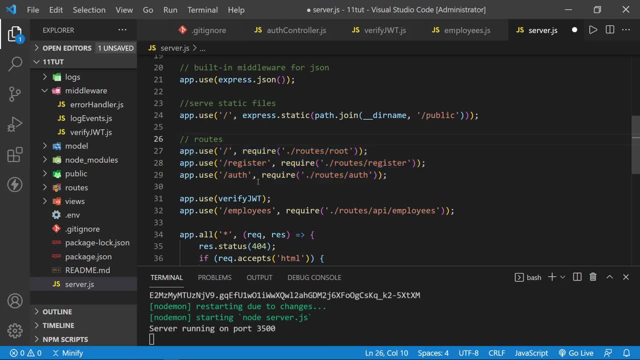 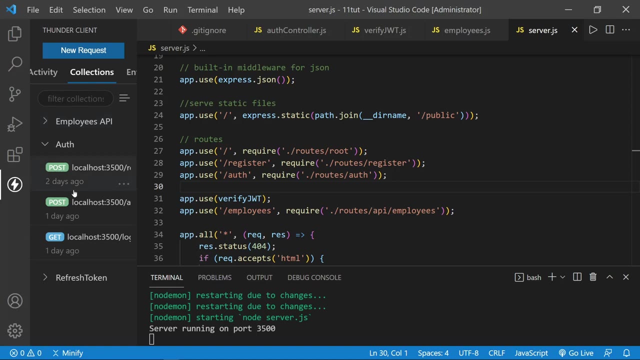 want to have verified with a jwt. we need to have above this line right here. so let's go ahead and save this once again. and now we can go back and let's log in again and get another. well, we close up the api there. there we go. here's our auth line. let's log in and get another 30 second access token. 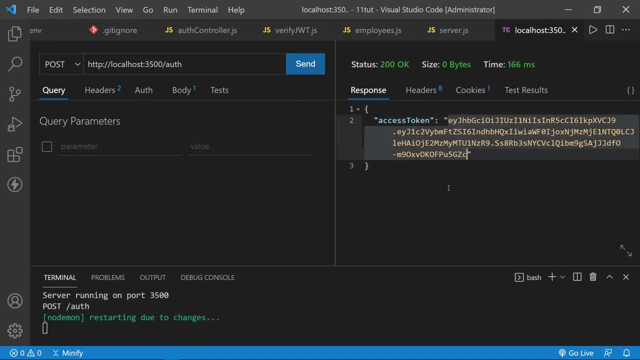 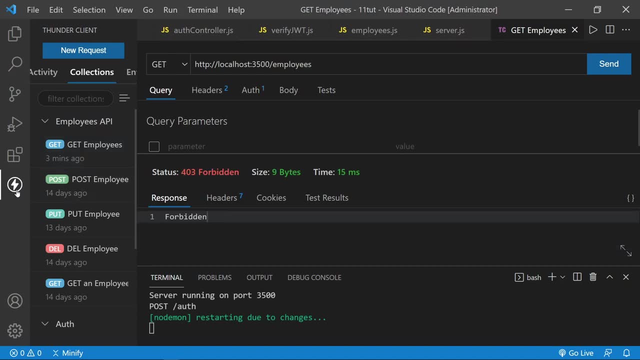 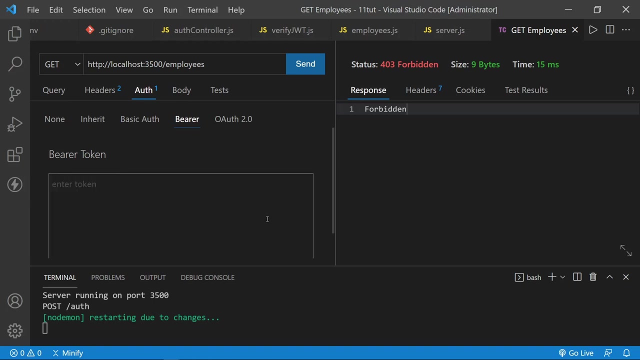 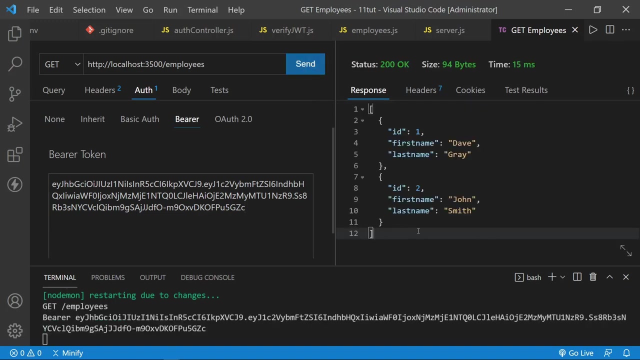 here we are okay. now let's go back to the employees and once again we can just use the git route. before it was forbidden because it expired. but now let's go to the auth tab here in thunder: client select all, delete that, paste in the new token and submit and we've got our employees list once again. but if i continue, 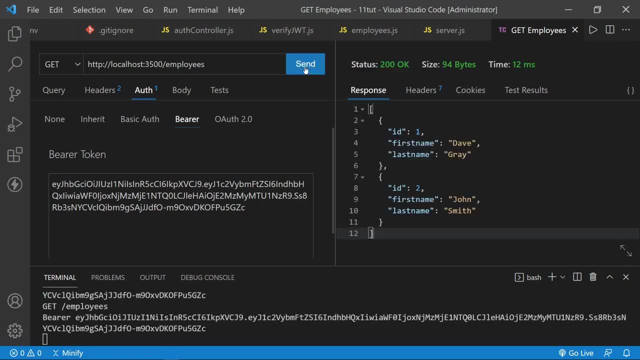 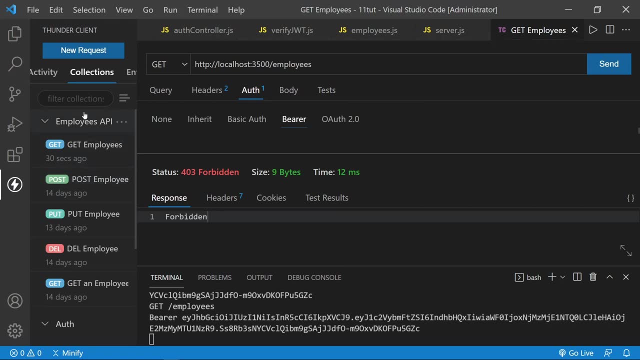 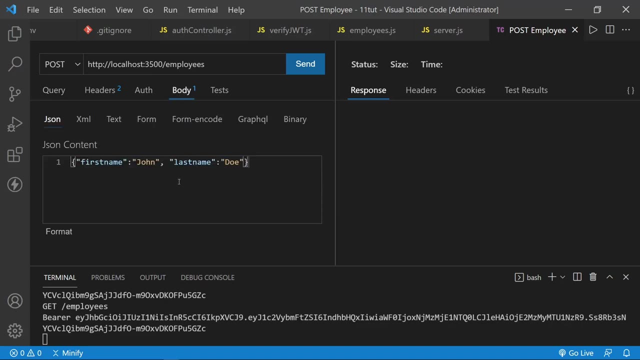 to submit. it will expire as soon as the 30 seconds is up. and there is our 403. and just to show that now let's go back to our employees, api to the post route for posting an employee, here in the body we've got john doe, so that looks like we could go ahead and post to the employees for john doe, let's. 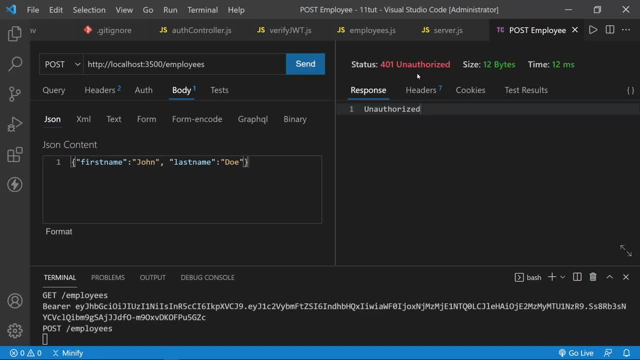 see if we can send this and we get unauthorized. so our verify jwt middleware is working on all routes. okay, let's go back to the file tree. we can close the terminal once again. we can close out of thunderclient for now. let's go back to the file tree. we can close the terminal once again. we can close out of thunder client for now. 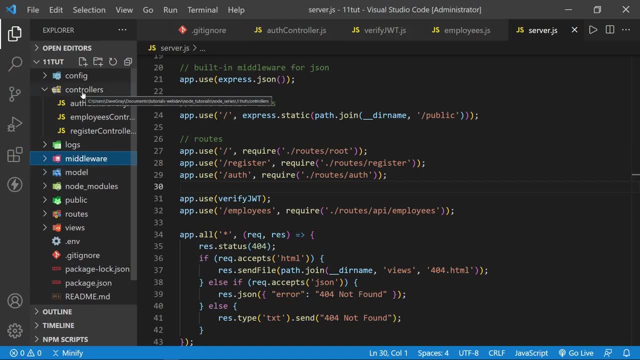 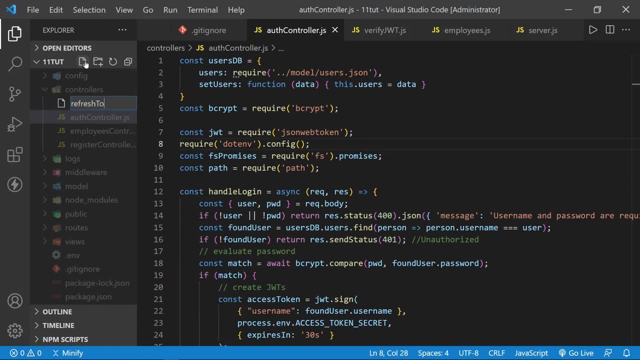 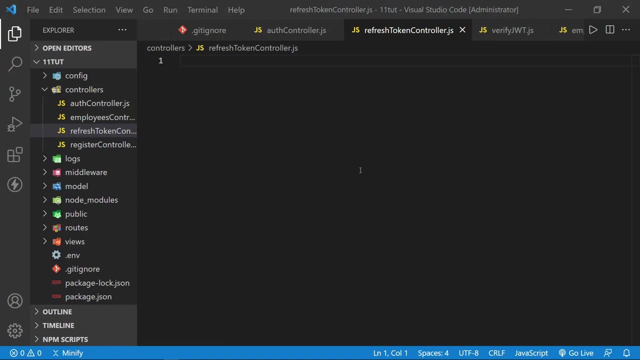 and let's close up the middleware. what we do want is to go back to the controllers and we're going to create a new controller here called refresh token controllerjs, because we're going to have a refresh token route. and before we get started on our refresh, 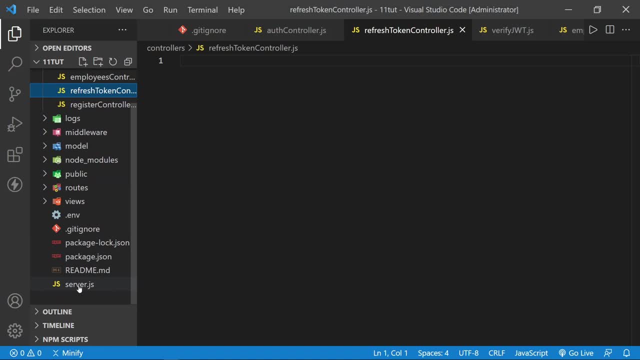 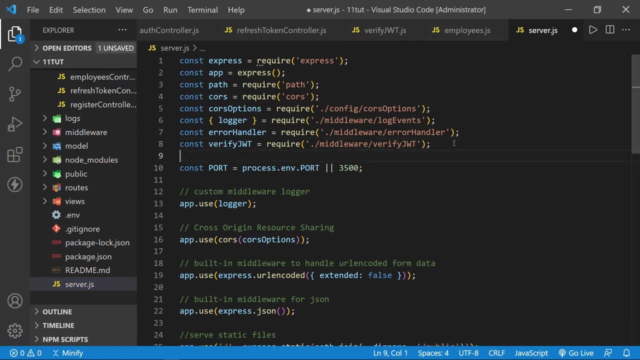 token controller because we're going to need it. let's go back to the serverjs quickly and at the top of the serverjs we pulled in the verified jwt. we also need to go ahead and define cookie parser, the other package that we had required at the beginning of the tutorial- and let's require cookie-parser. 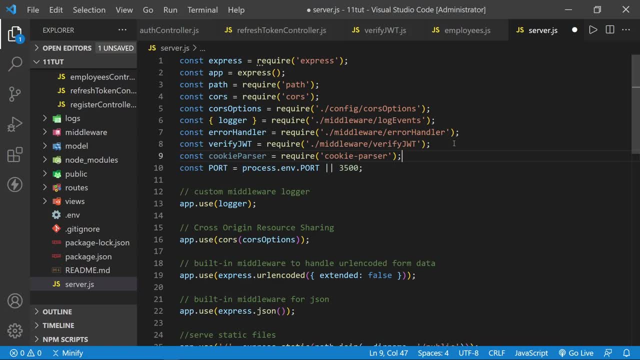 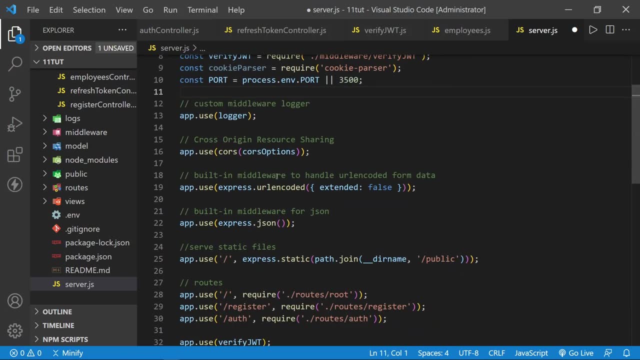 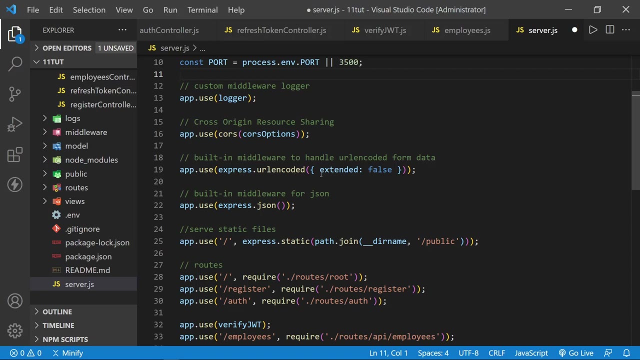 there we go, but we'll define it with cookie parser capital, p, camelcase right here, so i can go ahead and copy that now, much like where we used the expressjson and expressurlencoded that we use for formdata. and of course, option is pointless if we don't know which account to match it to. but we'll всегда vibe it. and when they load there's añ, here's going to adding it to theDiejeuner folder there again, as we said, if we do that, you have to kind of note that. and of course, if we switch to the- here's a picture- we're going to need to empty this file. 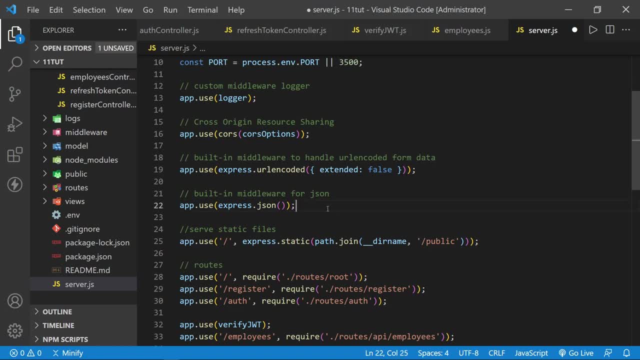 there's something else to do, but i'm just going to create another folder here and we're going to add an pathь course. expressjson is for JSON data. We just want to add middleware for cookies right here. So we'll say appuse and now we'll pass in cookie parser and we want to call that into action, right. 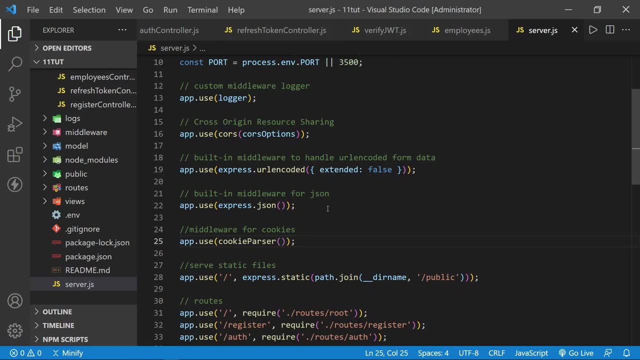 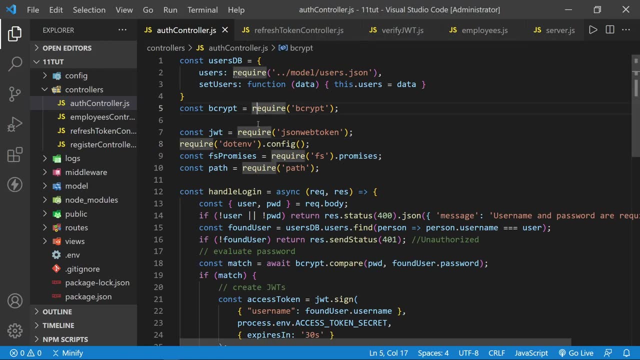 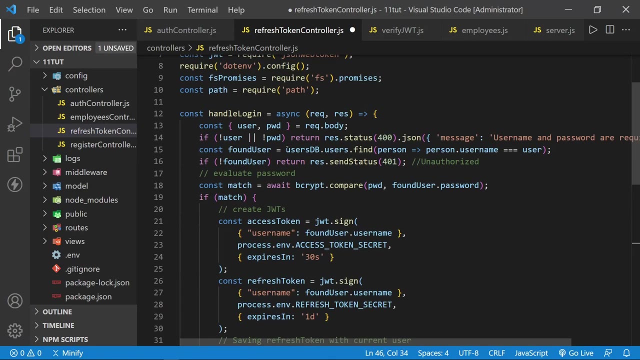 there and save our serverjs file. Now we're ready to go right back to that refresh token controller and we'll begin by copying the auth controller, Control C. I'll just copy everything and paste it in, but we will make some modifications. So we need the user's DB. We will not need bcrypt. 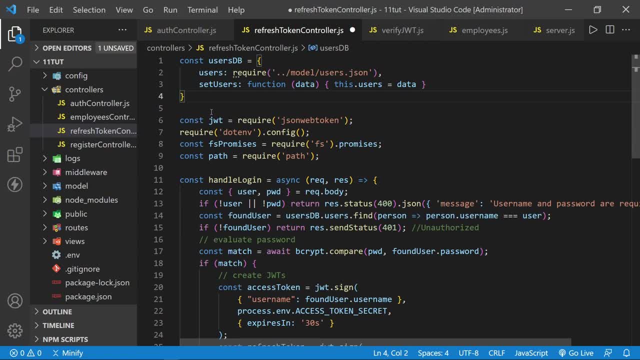 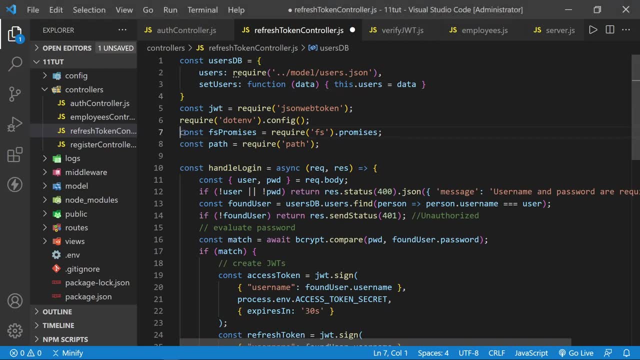 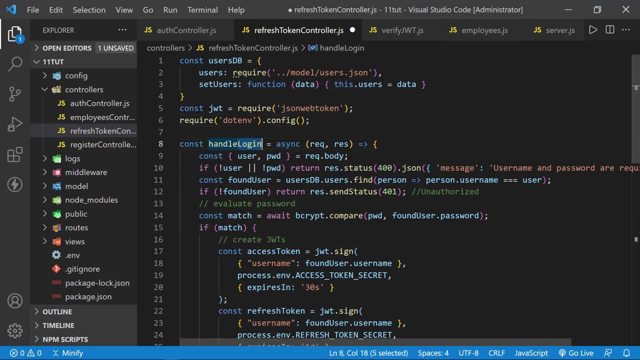 because we are not doing user password authentication there. We do need JWT and env, but we won't need fs promises or the path in this either. So we can remove those dependencies Now. instead of handle login, let's call this handle refresh token, and this does not need to. 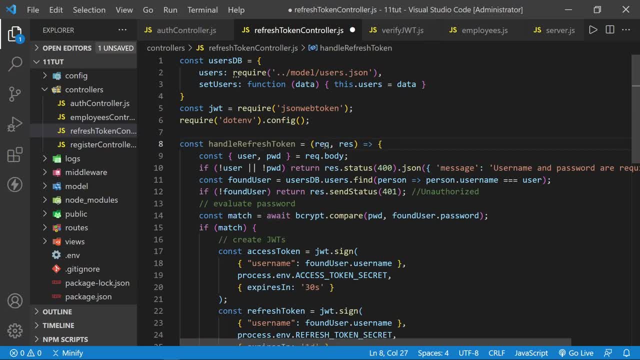 be async, So we'll just have the request and response here. After that we won't be looking for a password, but we will be looking for a cookie. So let's say const cookies and set this equal to requestcookies, And so we will have a similar if statement here. 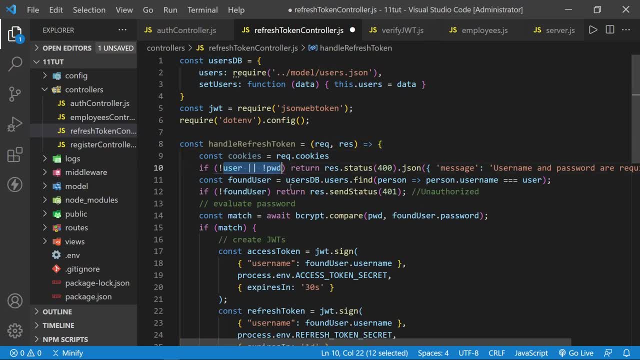 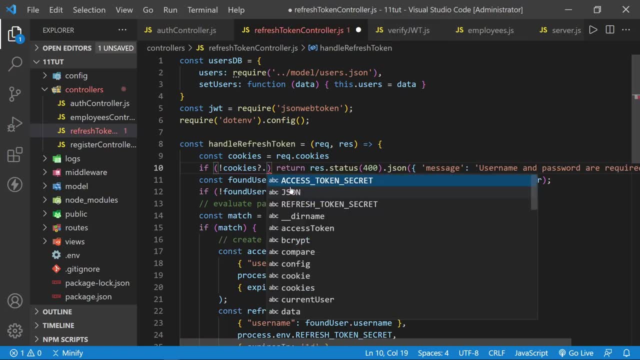 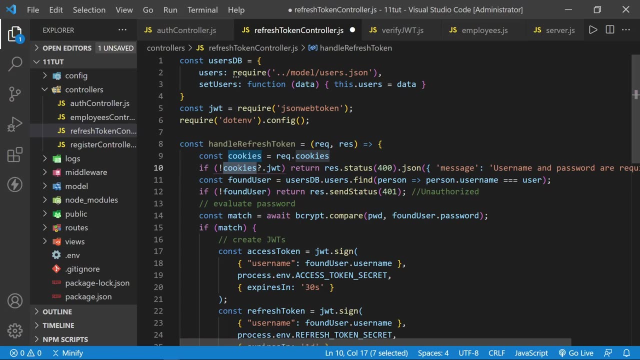 But we'll be checking for a couple of things. One is to make sure that we have cookies. But now let's use optional chaining with a question mark and a dot the optional chaining operator and put JWT after it. So we're checking to see if we have cookies and then, if we do, 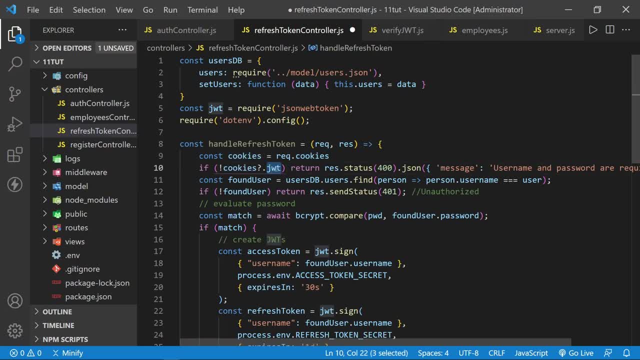 have the cookies. we're also checking to see if there is a JWT property. And this is saying, of course, if these do not exist, then we're going to return something here And we're going to return a 401 and we do not need a JSON message after that. So I'll just eliminate. 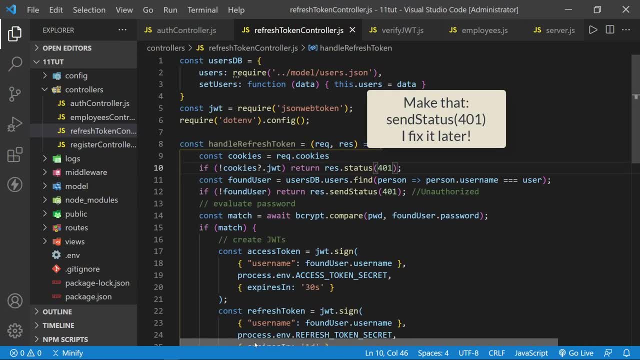 that portion of it and save this. It looks like I may need to go ahead and press alt Z to wrap any lines that exceed the edge of the screen. So there, we've got a 401 if the cookies do not exist, And maybe we have cookies but no JWT. Either way, that gets a 401, which is unauthorized. Now let's go. 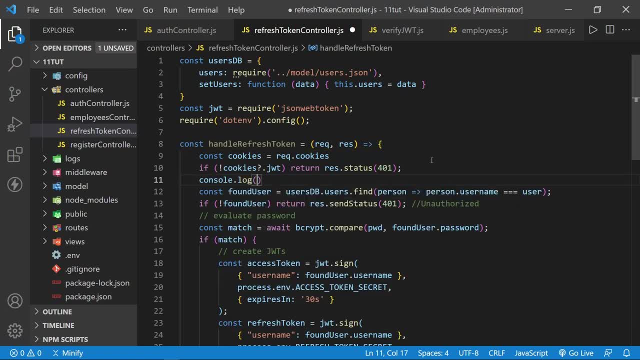 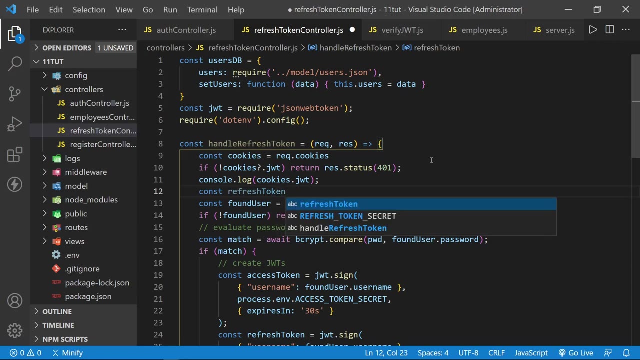 ahead and confirm that at least. and let's log to the console cookies dot, JWT, So when we run this you'll be able to see what values we get from that. And likewise, let's go ahead and find the refresh token Now that we've received, now that we know it exists within. 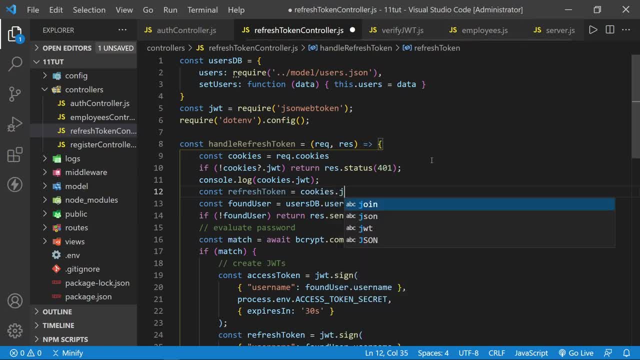 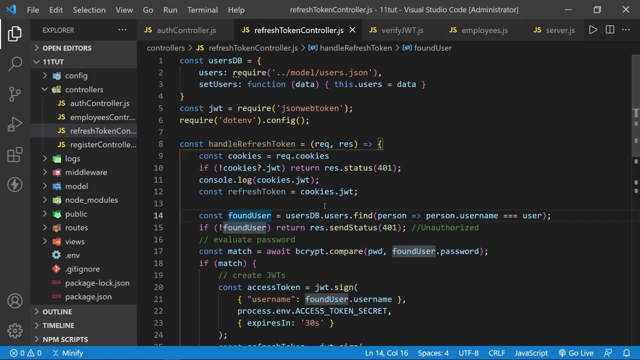 the cookie and we'll set that equal to cookies. dot JWT. And once again we do want to find a user, But now we're receiving a refresh token and not a user, So we'll say person and there is a refresh token that should be saved with each user if they have. 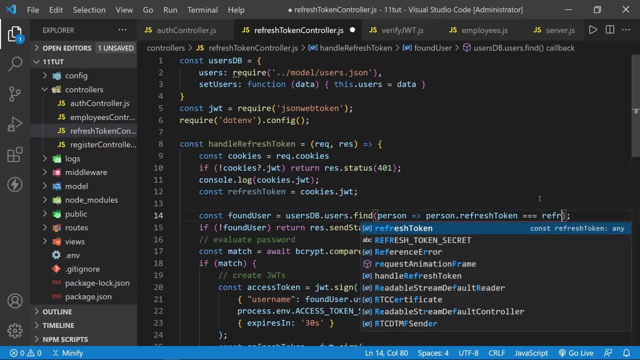 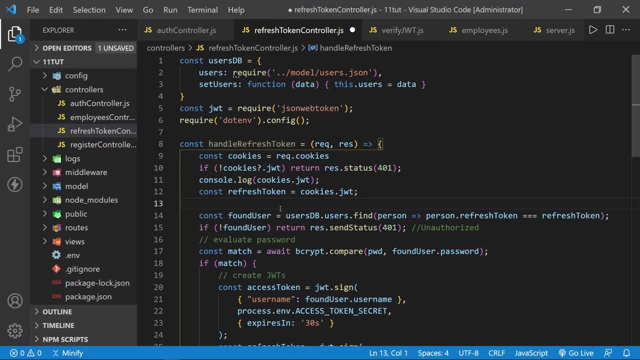 created one, And so here we'll just match that to the refresh token that we have now defined here, So this would be our found user. then if that user exists, And once again we can say: if we do not find a user, let's now send the status forbidden here, And I'll just highlight that. Okay. 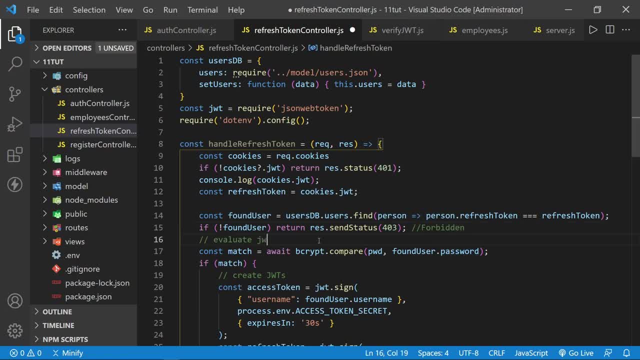 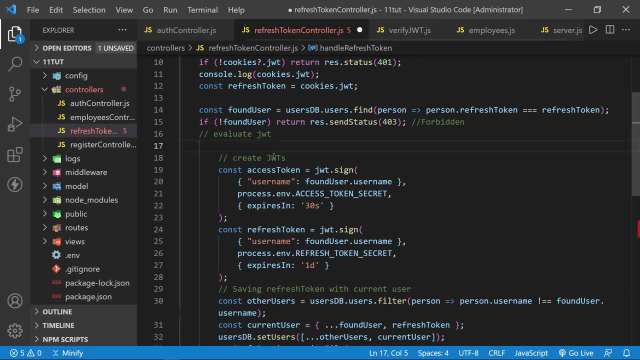 we're not evaluating a password here. We are evaluating a JWT, though, So these lines will change as well. So we can get rid of the const match line And instead- well, we can even get rid of the if match here as well, And instead of that we'll type JWT, dot verify. And now we'll. 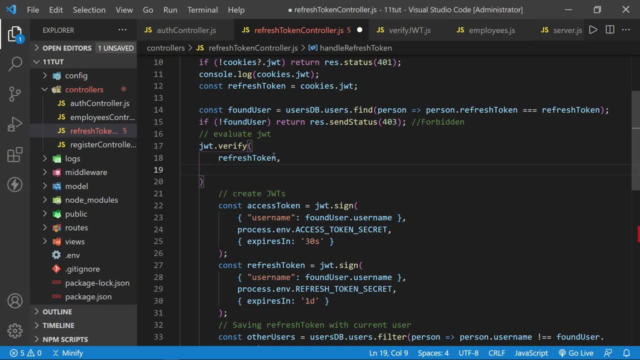 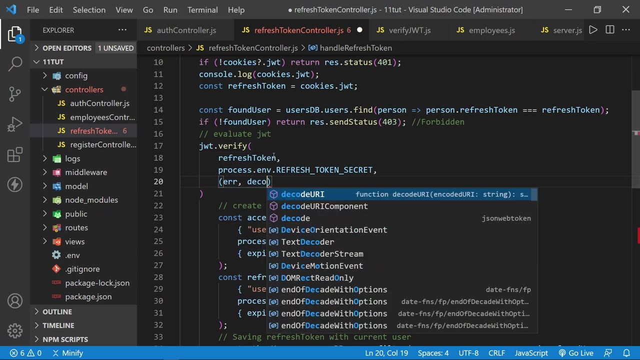 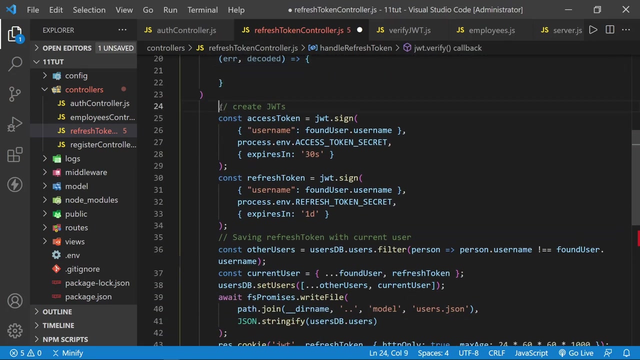 pass in the refresh token that was received. Now we'll say process dot. ENV. dot. refresh token secret. And then we'll have an anonymous function that once again has error and decoded its callback function. And before I type the rest, I think I'm just going to get rid of. 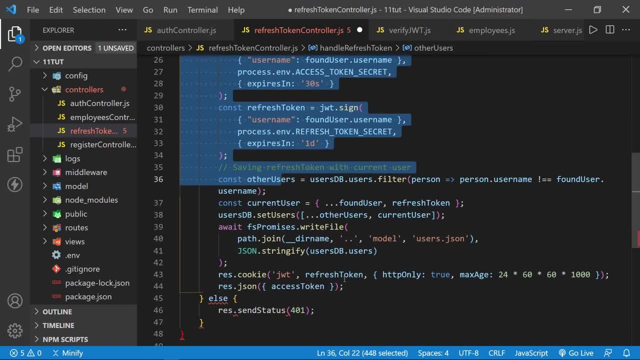 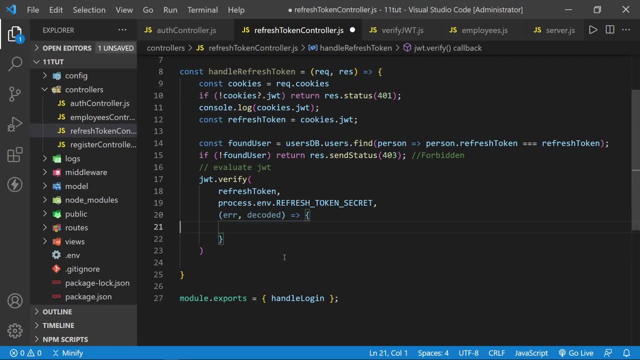 this because it doesn't need to be there at this point either. So let's just go ahead and clear it out now And with that cleared out, we can finish our function here for the token verification, And if we do not have a valid token, we can say if we have an error, or we can also check the found. 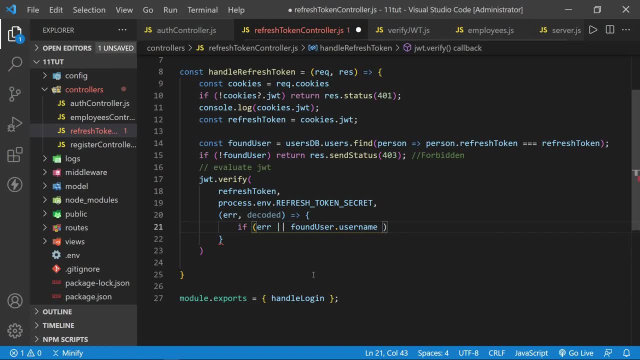 user dot username, because we did have the username encoded in the token. So if it's not equal to the decoded username- in other words, maybe it was tampered with again- then we can return a response with a send status And say 403 once again. Otherwise, everything is good And we're ready to create a new access token. 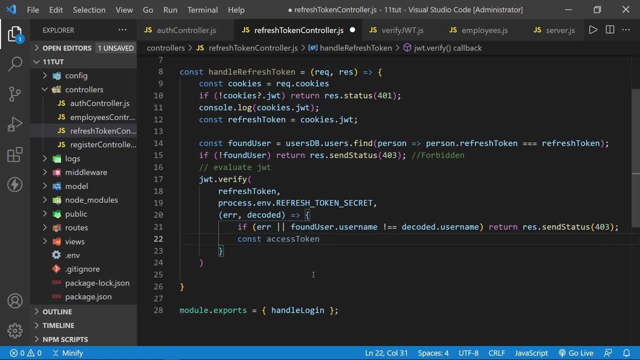 to send because the refresh token has verified. So we'll set this access token equal to JWT dot sign And then inside of the access token we'll once again have a username, And this username will be the decoded dot username, because it should be the same username that was verified before. 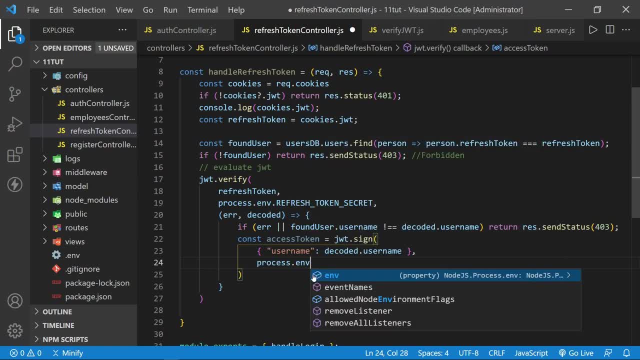 And after that we can say: process dot, env, dot. access token secret. If we can find that access token secret, there we go, And then we need to put an expires in once again. Let's put expires in And let's set this to 30. 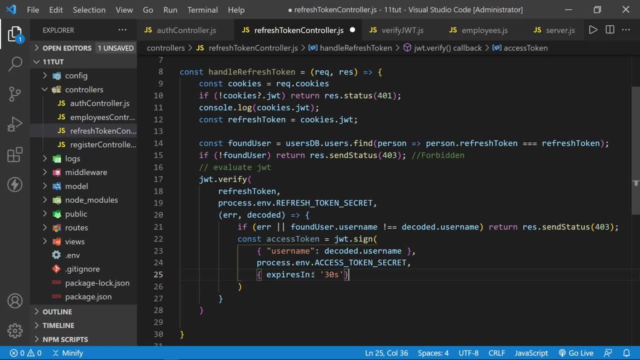 seconds as well. However, remember you might want to set this longer in your production app. This is just for the demonstration of this tutorial, So I can show it Expire. And then, of course, after we've created this access token, we need to go ahead and send. 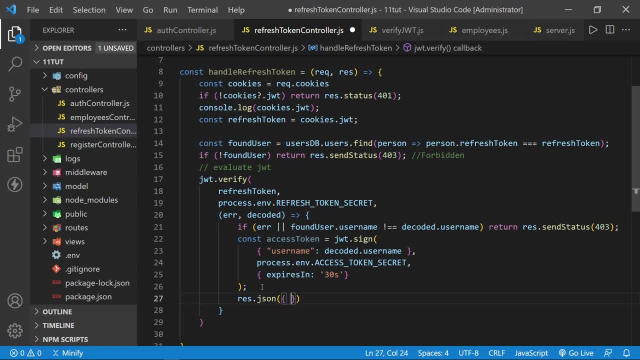 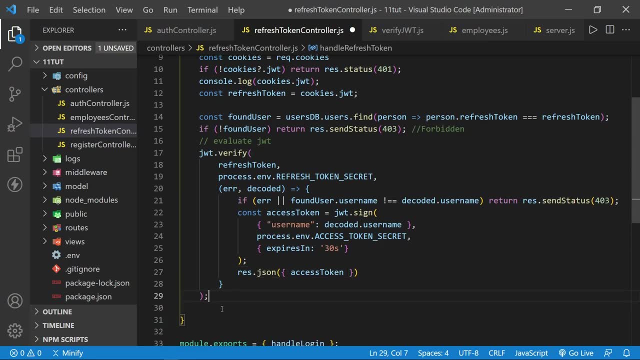 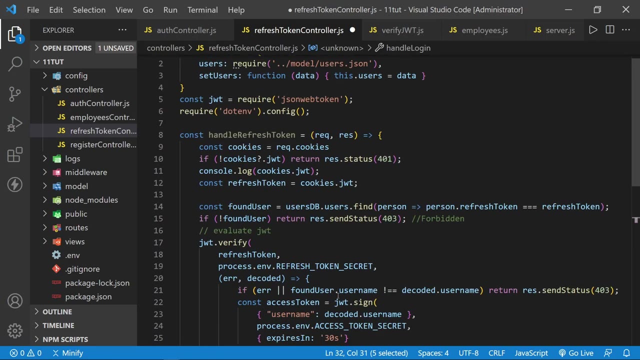 the access token. So we'll send this JSON down and it'll say access token, And once we've created that much, all we need to do is export it. So now, instead of handle login, we once again have handle. I believe it was refresh token, Yep. 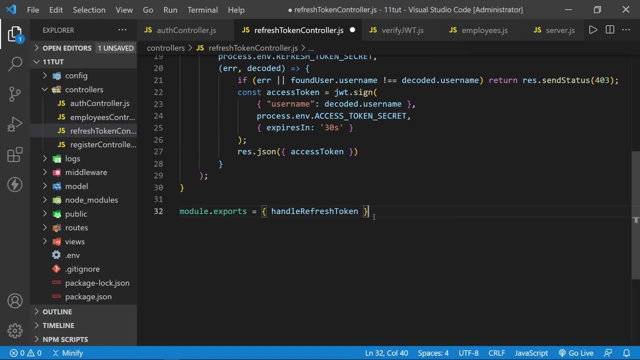 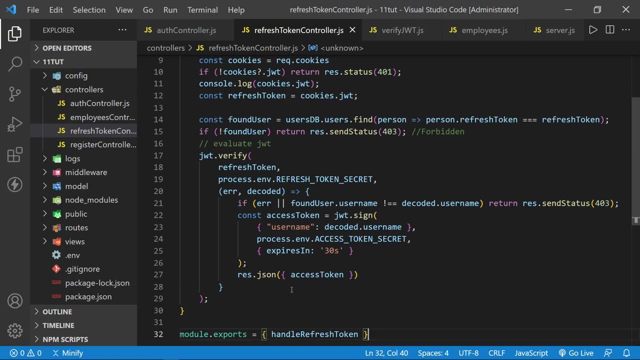 And we should be able to save that. And I don't know why I put a semicolon there, It's not really needed. So once we have saved that, we should be good to go with our refresh token controller and we can create the refresh token route. Okay, In our routes file. now we can open that up and we 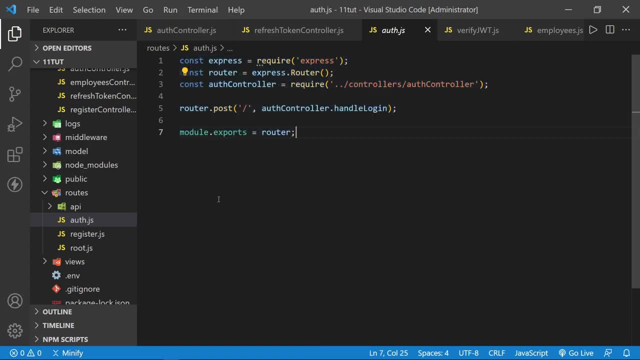 can look at our auth route. I'll just highlight all and copy and we'll create a new route called refresh dot JS. I'll go ahead and paste that in And then we can go ahead and save that And we can paste that in. But instead of the auth controller we need the refresh token controller. So 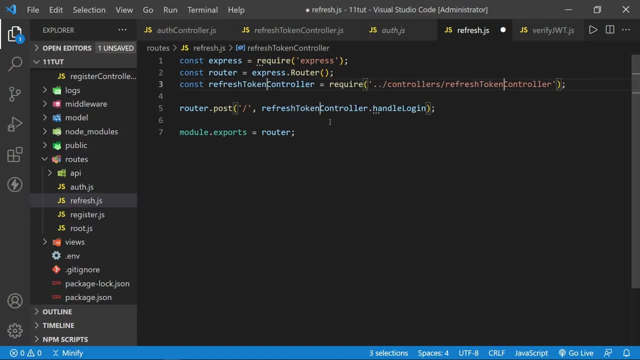 spell all of that out. And instead of handle login, we need handle refresh token. And before we're finished with our refresh route, let's change the HTTP method from post to get as well. So this is now a get route for refresh. Okay, Now we need to insert this route. 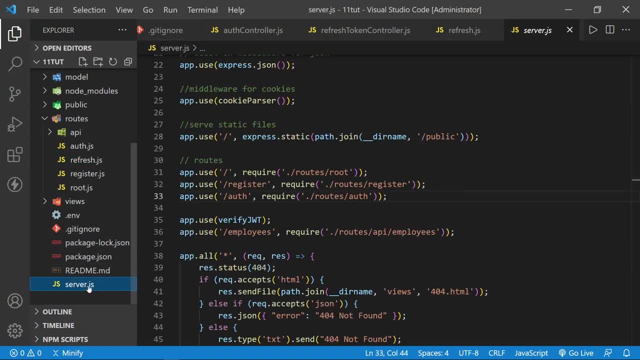 into the server along with the other routes. So we'll go to the server JS file and you can see we've got root register auth. And of course we want this to also be before we verify the JWT, because the refresh route actually issues a new access token And that's what verified JWT. 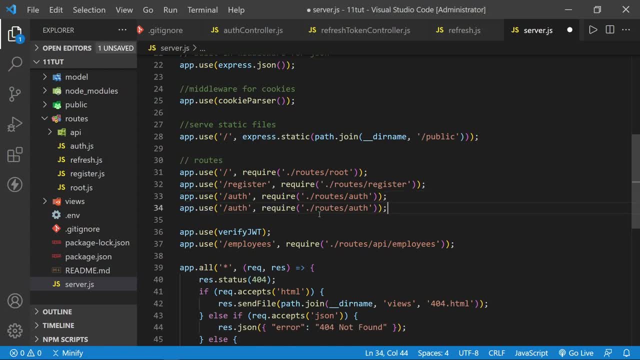 verifies. So what we want to do now is just copy a line down. I pressed shift, alt and the down arrow in windows to do that And I'm going to just copy and paste that in And I'm going to change auth to refresh, And now the refresh endpoint will receive the cookie that has the 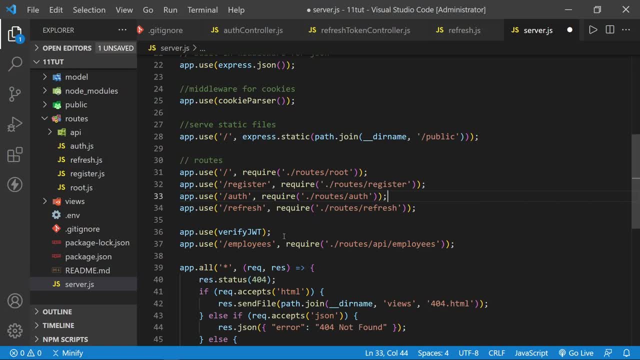 refresh token And then that will issue a new access token once the access token has expired. So we'll save this and we should be ready to try it out. So I need to open up the terminal window again And we can see our server is running on port 3500.. Now let's open up Thunder Client. 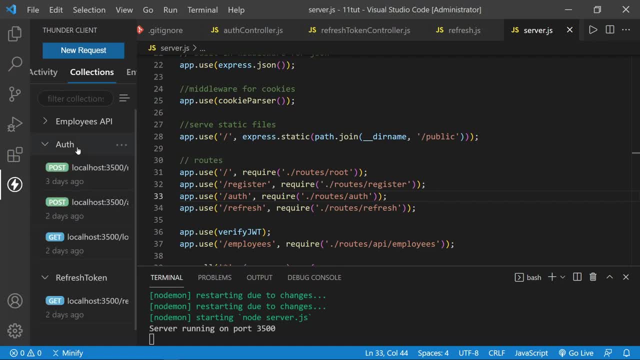 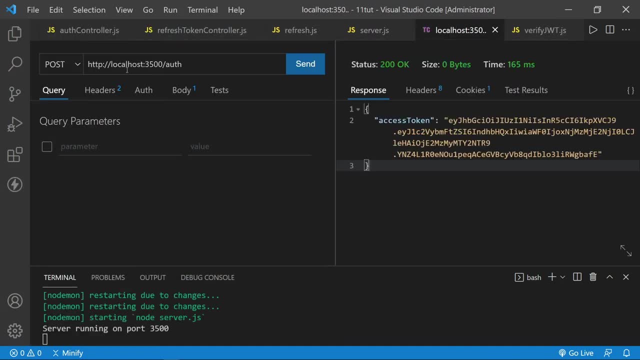 And we're ready to check out the refresh route. But first we need to go to the auth route, And here it looks like the auth path. I'll hide the tree over there. And so now we're going to localhost 3500, auth. We're once again going to authorize Walt here with his password. 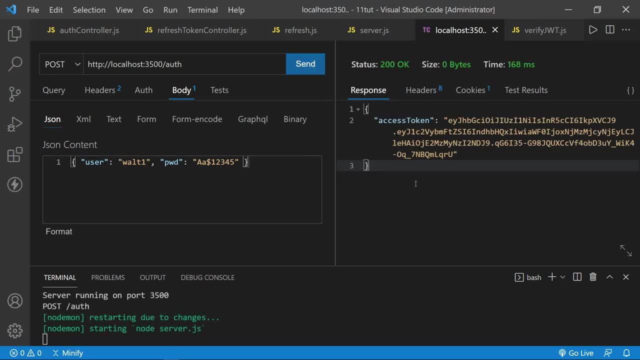 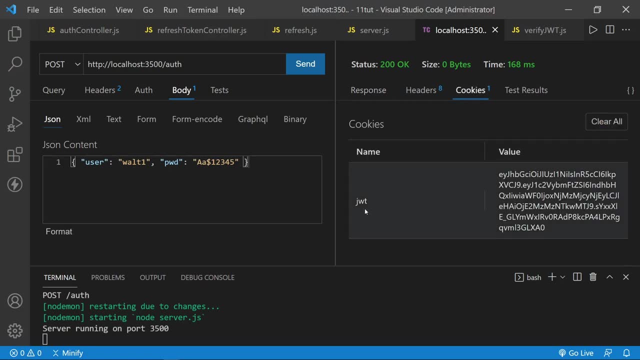 So let's send this And we got a new access token. But what we also get from our auth route is a cookie, And this cookie has our refresh token. And here's the JWT name for the cookie And here's the refresh token. Now a cookie is sent every time. We don't need to. 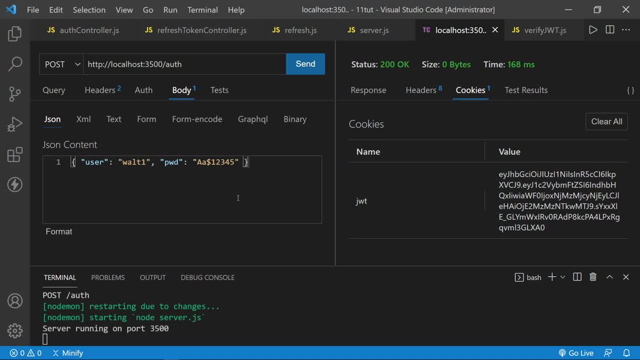 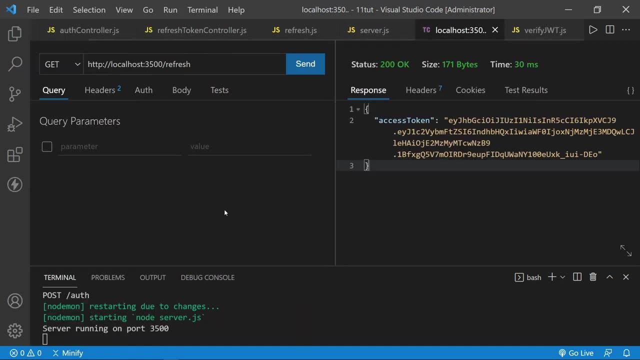 paste it in in an auth area, like we did with our access token. The JWT cookie is sent every time we make a request to the domain that it's associated with, So we'll go back over here to Thunder Client, We'll come down to our refresh route And I'll hide that tree. Now we're going. 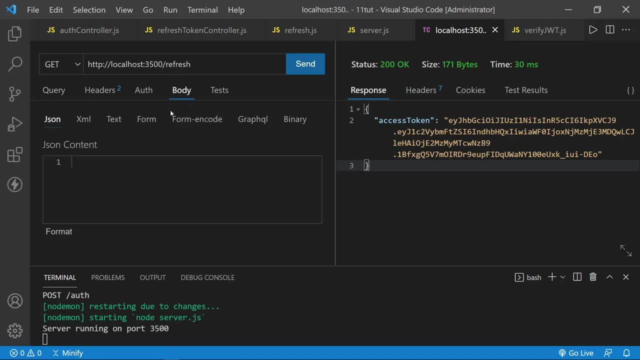 to localhost 3500 refresh And you can see we don't need to post anything in the body, We don't need to post anything in the auth because we have the cookie that we're going to send. So let's send this cookie. And now we got a new access token And you can see we also logged. 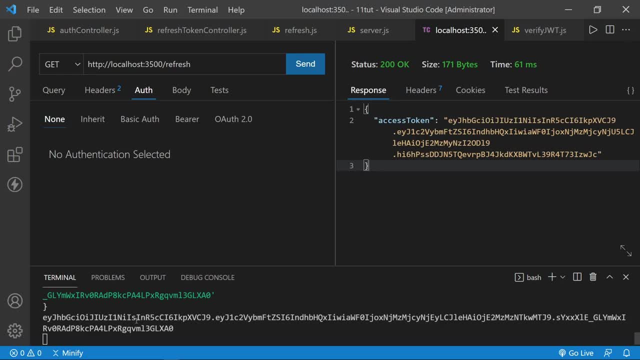 our information as we set it up in our path to log the refresh token that we received from the cookie down here. So we've got a new access token And our refresh token is used to do that. So now every time we hit this refresh route and we send our cookie with the refresh token we should get. 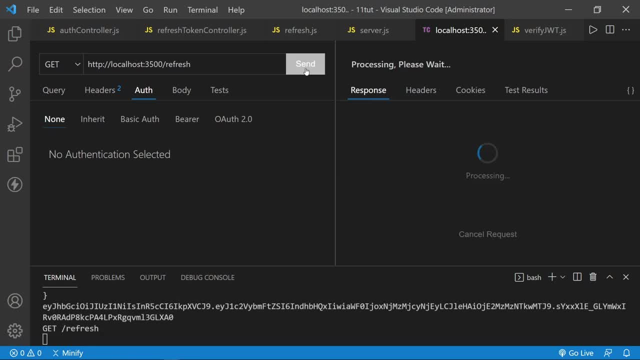 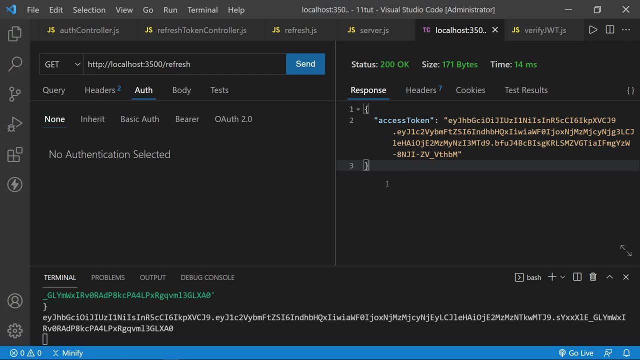 a new access token And you can see every time we're getting a different access token over there. So that is what refreshes our access And that's why it's called a refresh token. And so now we have a new limited time access token to use Again in production. you might want to set it to. 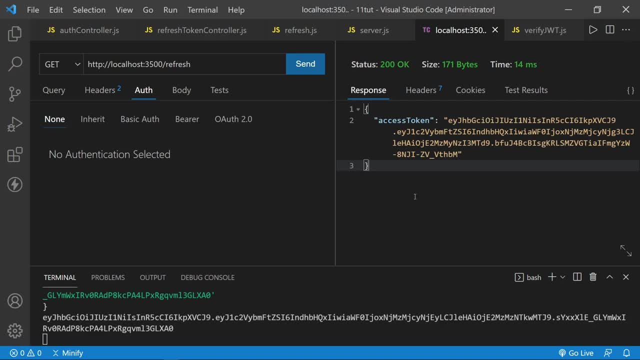 five minutes or 15 minutes instead of 30 seconds, or something like that. But then our refresh token has the longer duration that we store in an HTTP only cookie, And that's because we don't want it to be available to us. So we're going to set it to five minutes or 15 minutes instead of 30 seconds. 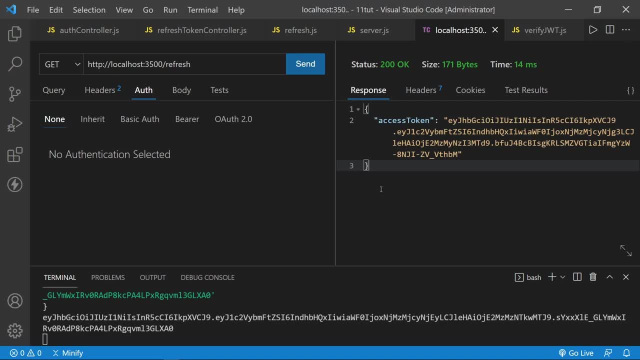 via JavaScript, So it increases our security. Nothing's 100% perfect, but it's the best way to go, I believe, for that. So we're sending the HTTP only cookie that has the refresh token and that issues us the new access token Now that we've finished testing the refresh route. 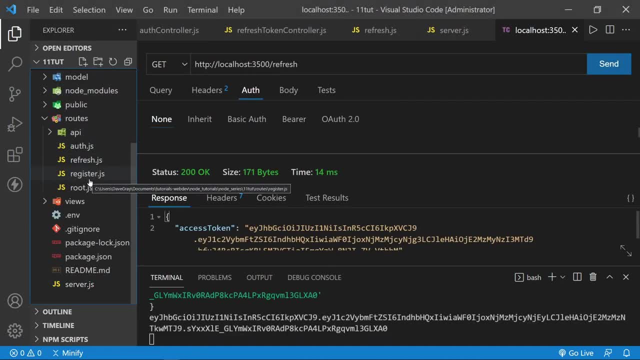 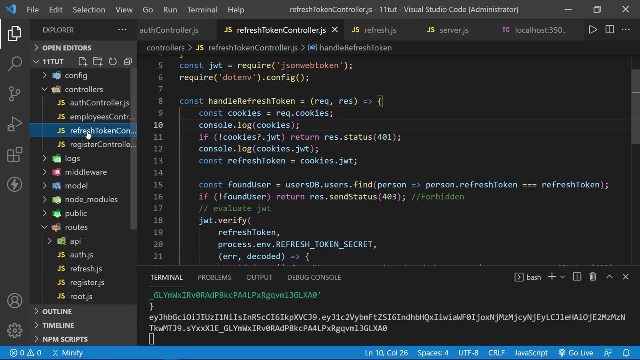 one extra measure of security or one extra step we can take is to offer a logout route, And with the logout route we could actually then delete the refresh token and not let it last for the full duration, And that just gives our users the opportunity to log out and, of course, delete any. 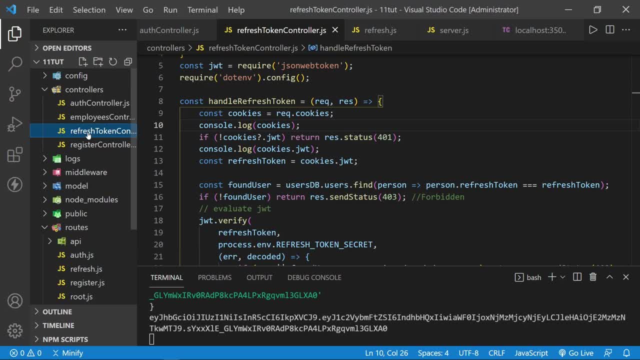 existing tokens And of course, the access token should also be erased on the front end when the login or logout link or button is clicked as well. Of course we're working on the back end, So we won't be doing that today, But let's go ahead and add this new controller for the logout, So we'll 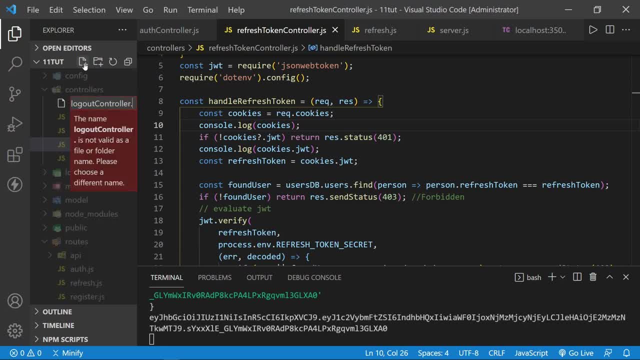 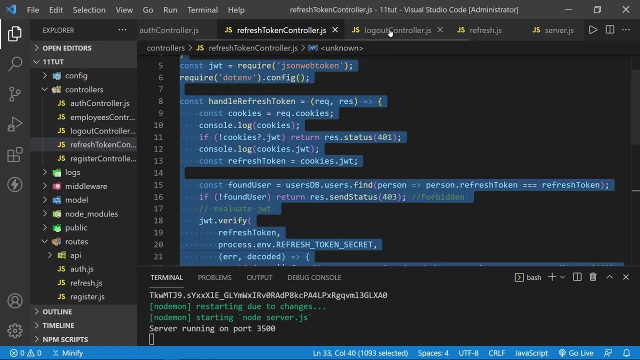 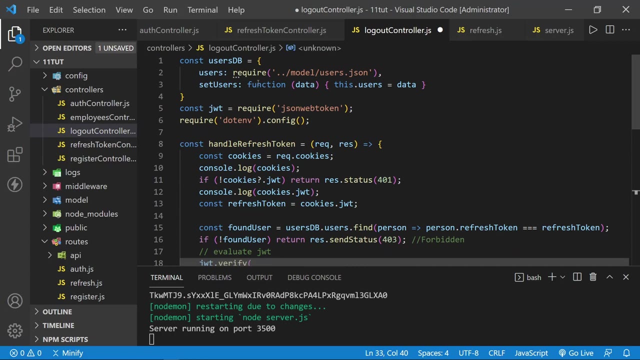 have logout controllerjs And now that we have that, let's go ahead and copy our refresh token controller And we will just make some modifications to handle the logout because we need the same requirements at the top. we've pulling in the users so we can check our database. We've got the JWT requirement and we've 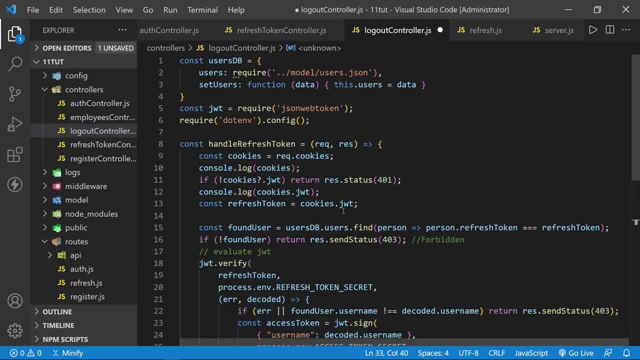 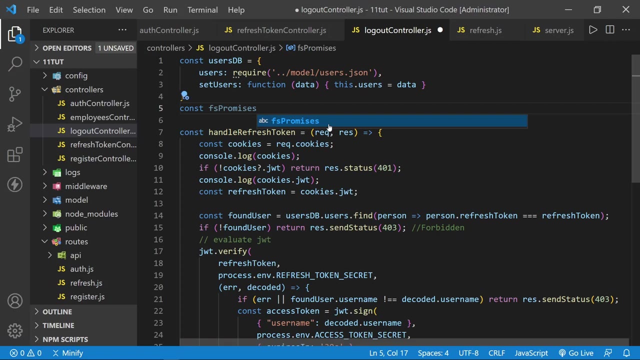 also got dot ENV. I'm going to close the terminal window And now I said we had the same requirements. we don't quite have the same requirements, I'm sorry. we don't need the JWT or the dot ENV. What we do need is the FS promises that goes with accessing our database, because we're just 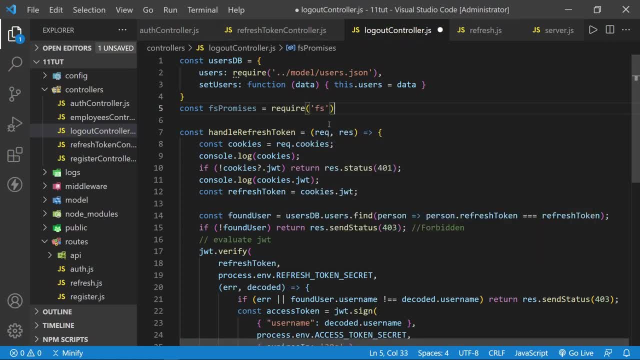 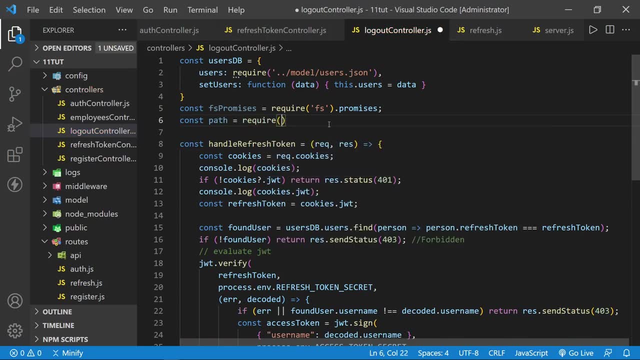 using a JSON file, So we'll require FS dot promises And we once again need paths, So we'll require the path. And again, these are only to access the current JSON file we're using for our user's database. This is a mock database. this will be replaced, of course. 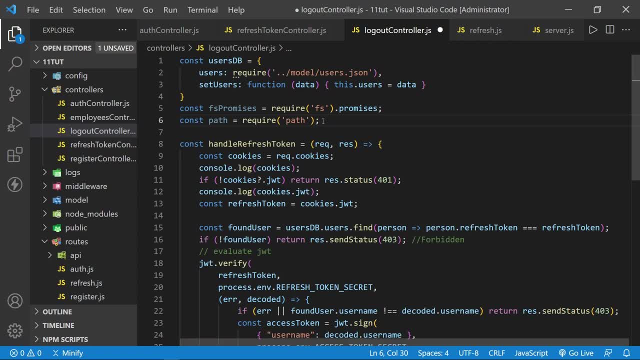 with Mongo or Postgres or whichever database technology we work on in a tutorial in the future. So we've got this down for the requirements And let's move forward with the logout. So instead of handle refresh token now, we're going to handle the logout And we'll have a request and response. 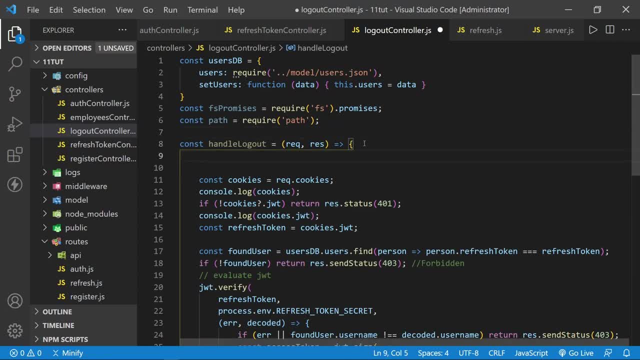 And then let's just add a note here for the front end: If you're doing full stack development, like on client, also delete the access token. we can't do that here on the back end. you need to do that in the memory of. 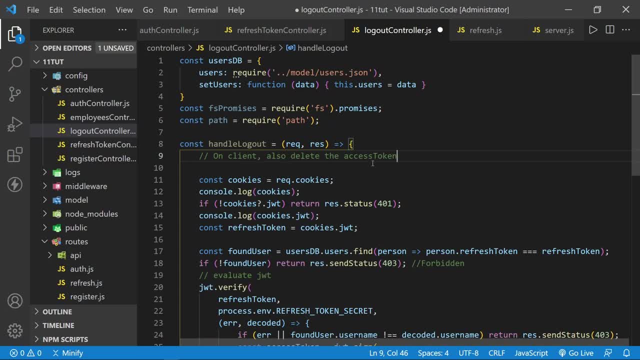 the client application, just zero it out or set it to blank, or whatever, when that logout button is clicked. What we can do, though, is take care of the refresh token, So here, once again, we need to get the cookies as they come in. Now let's erase our logs here. we were doing for the cookies, and 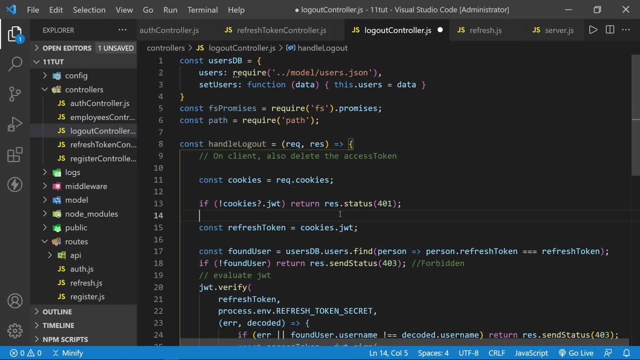 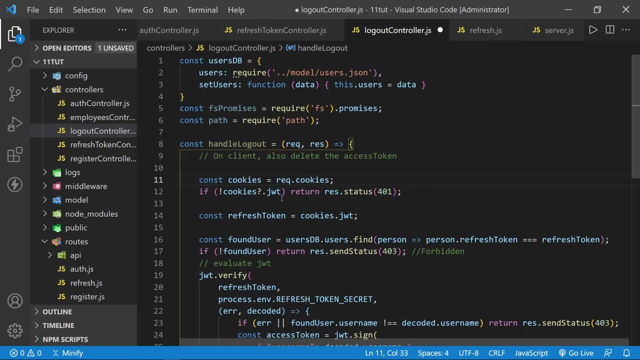 the cookies JWT before. If you wanted to see the cookies, you could see them in the cookies. but you can see those in the console And we'll once again verify that we have got cookies and then that we also have a JWT in the cookies. And if we don't, well that's okay, because we were just 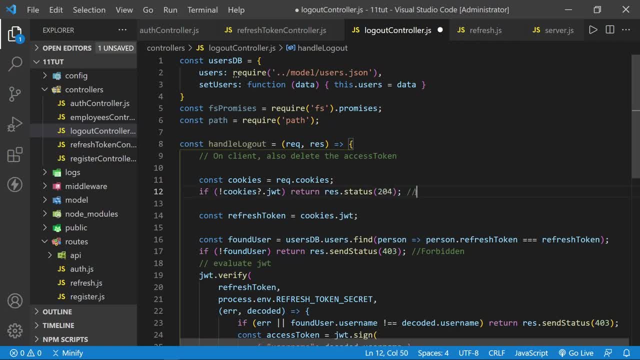 going to erase it anyway. So let's send a status 204.. That means it's successful And there's essentially no content to send back. That's what that status is. So you've had a successful request and we're not sending any content, And this needs to be send status instead of just sending content. 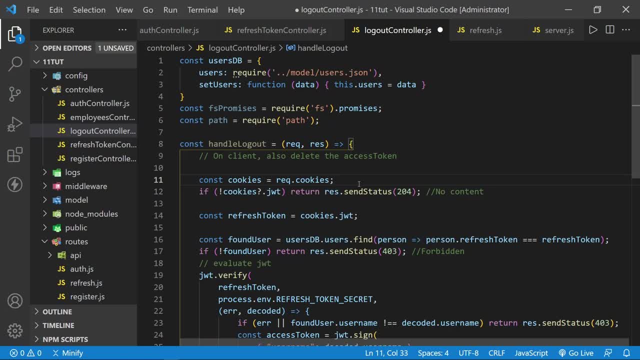 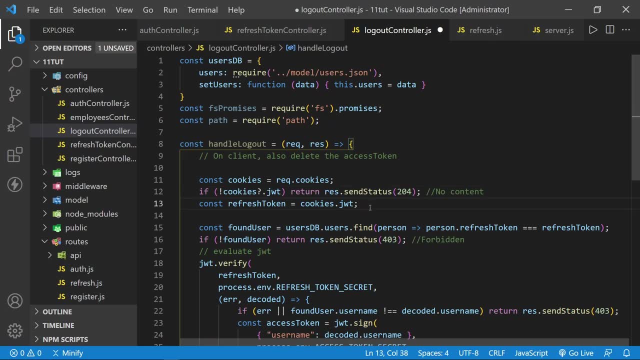 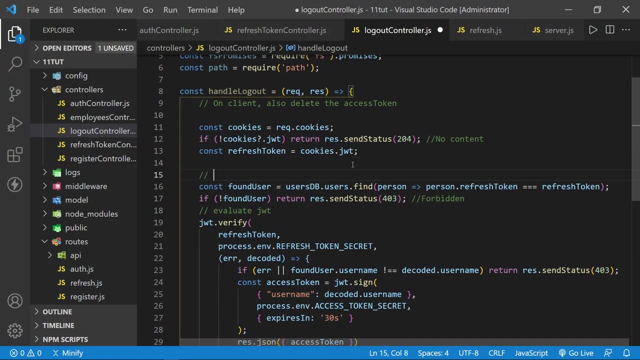 Just status. There we go: Response dot. send status. Got that. Now let's go ahead and define our refresh token, And we'll do that in the same way, setting it equal to cookies dot JWT. Now let's see if we have that refresh token in the database. So that's what we're checking here is refresh token. 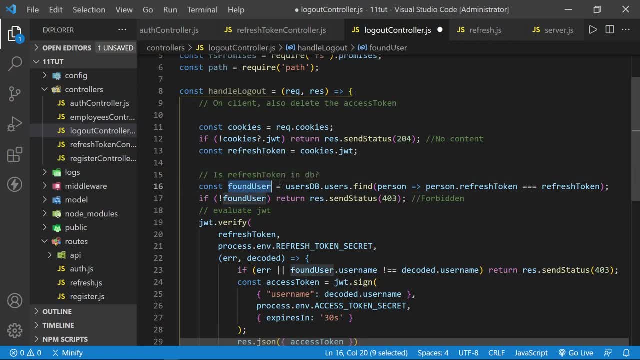 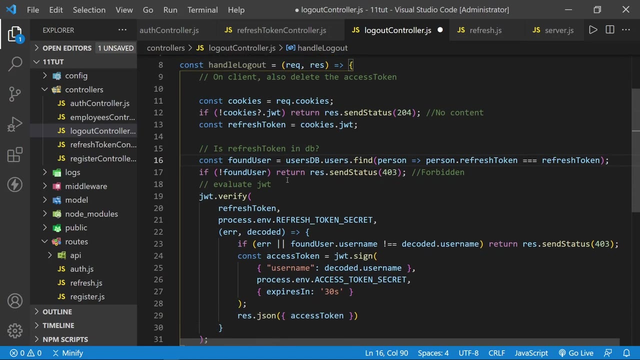 in DB. So once again, we try to find a user that has this token. So setting this equal to the user, Just as we did in the previous refresh token controller, is exactly what we need, And if we don't have a found user at this point, we can go ahead and clear the cookie. So we're going to 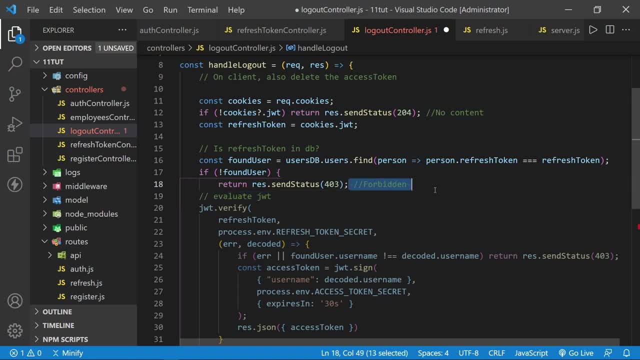 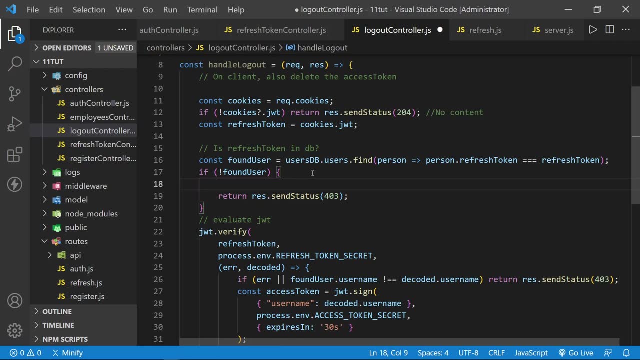 do something just a little different here, And it won't be forbidden either. So we'll get rid of that And let's go ahead and look at how we clear the cookie first. So if we don't have a found user, but we did have a cookie to get to this point, we can just go ahead and erase the cookie that. 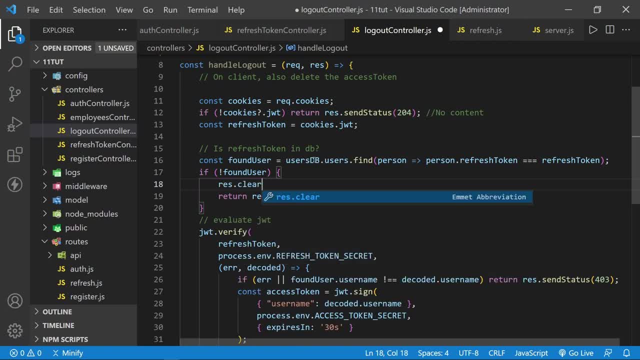 and that's going to be with response dot, clear cookie and then inside there we'll look for the JWT cookie and then you have to pass in the same options that it was set with. So once again we'll say: HTTP only, set that to true, and that should be all we need to do there, except for sending the. 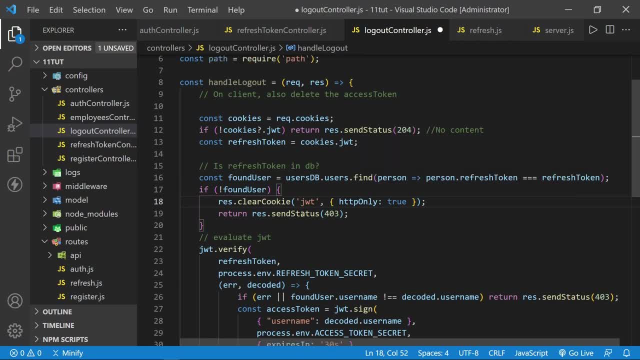 proper status. So once again, we're going to return and send the status not of 403 but of 204, which once again means this was successful, but no content. Okay, I'm going to scroll up just a little bit and now we can pretty much erase everything here and we're going to create some. 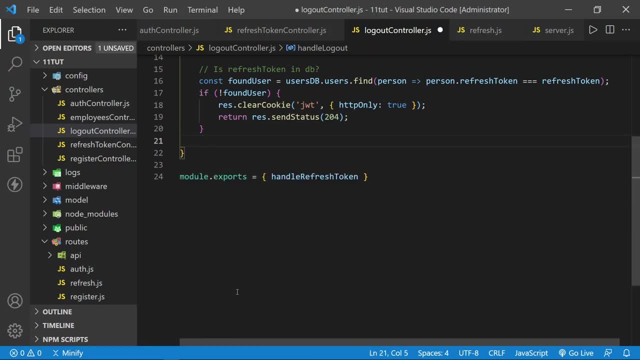 new content below, because if we've reached this point, that means we did find the same refresh token in the database. so now we need to delete the refresh token in the database Right here, and we're using file system of course for that instead of mongo or postgres at this. 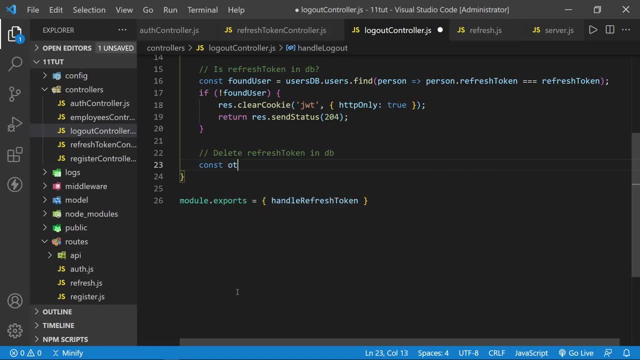 point, but we will change that in the future. Right now, let's define other users, which would be all of the other users that are not the user that we found, and set that equal to users db dot, users dot filter, and we'll just filter this out. we'll pass it in the person and now the person dot. 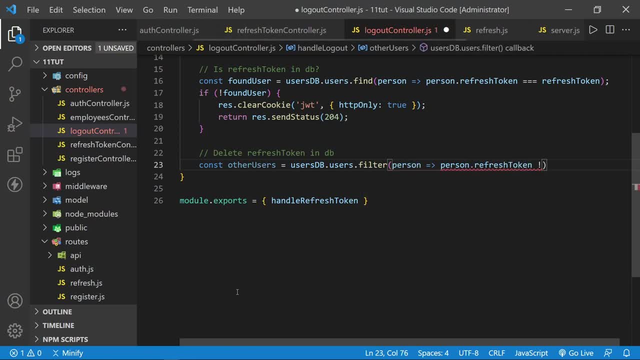 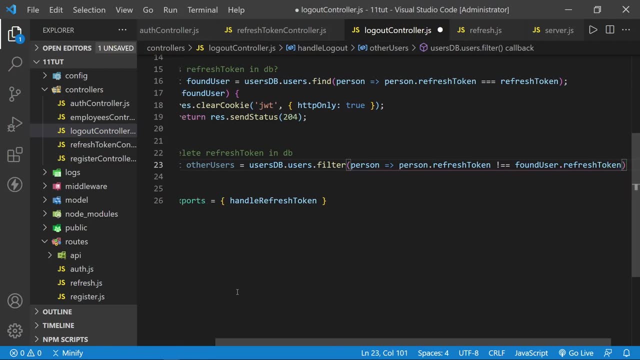 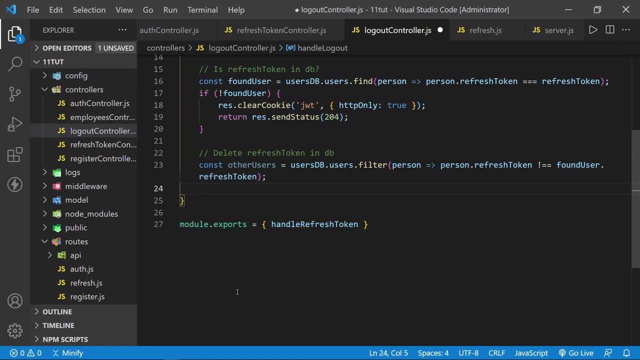 refresh token is not equal to our found user. dot refresh token as well. there we go, okay. so I'm going to press alt z to wrap that line of code so we can see all of it, and that's all the other users. so now our current user is going to be equal to our found user, and then we're going to 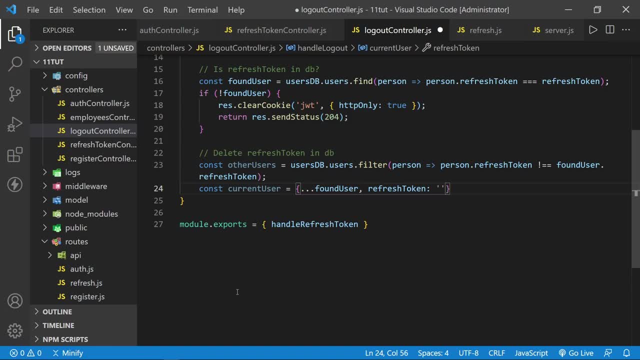 set the refresh token to our found user and then we're going to set the refresh token to our found user blank, so we'll leave the refresh token property, but now we're just erasing it from the user and now we can update our users db with our set users and we'll go ahead and pass in our other users. 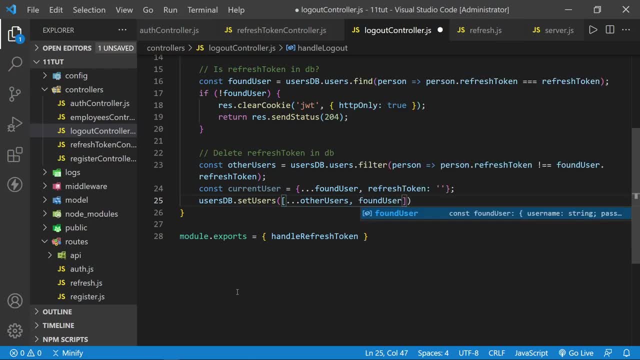 and then we'll pass in our found user. oh, and I'm sorry that's not found user. that should be the current user that we just defined. there we go. so found user was before we erased the fresh token. now the current user has the updated refresh token that is zeroed out or blank, if you will. 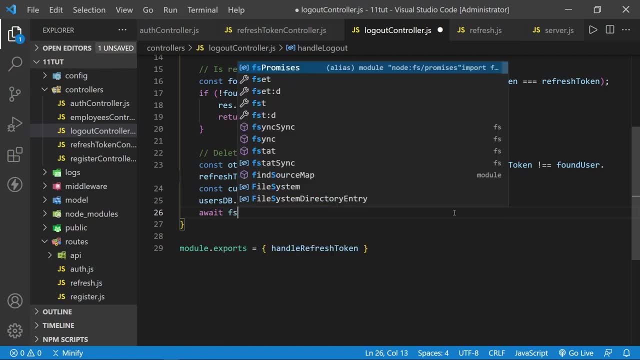 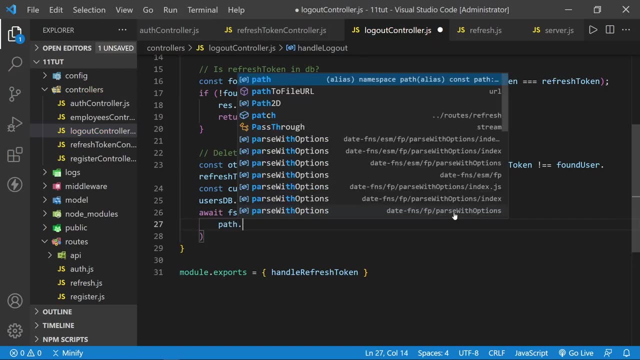 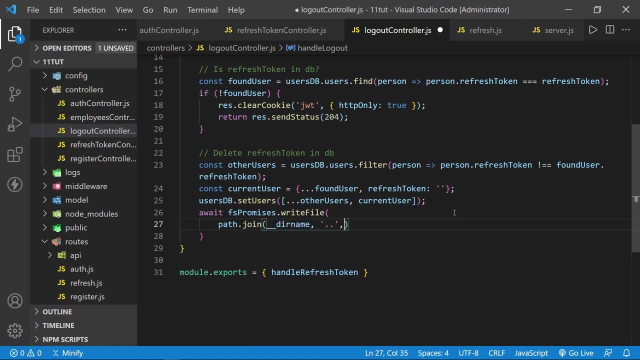 now let's just write this to the file. so we'll await fs promises dot write file. and now on a separate line here I'm going to say path dot join, pass in the directory name. after that we'll need to come up one folder and then we'll say in the model folder and then we'll name the users. 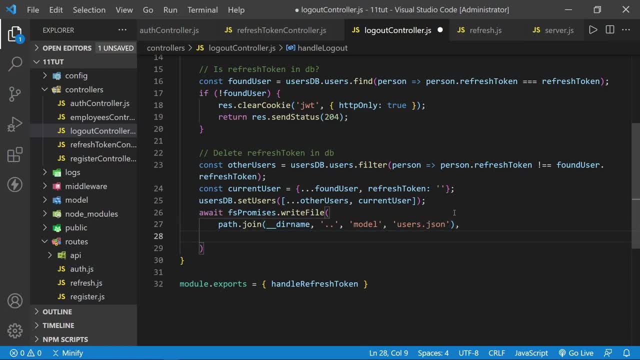 dot json file. okay, then we need to go ahead and use json dot stringify and write in the users db dot users, and that should update our users file, and so after that we need to go ahead and delete the cookie, which we saw how to do before as well. so we use clear cookie. 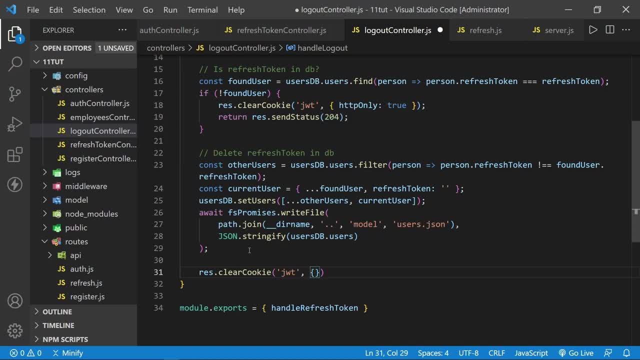 and we reference a jwt and we need to pass in the same options as well. http only set to true. now I will add in production both when we send the cookie and when we delete the cookie. you also want to add the flag secure. true, and that will make it. 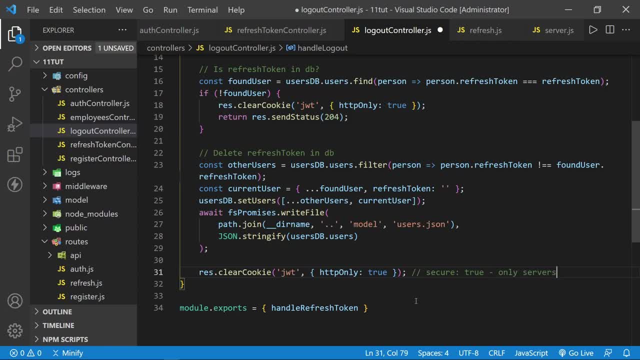 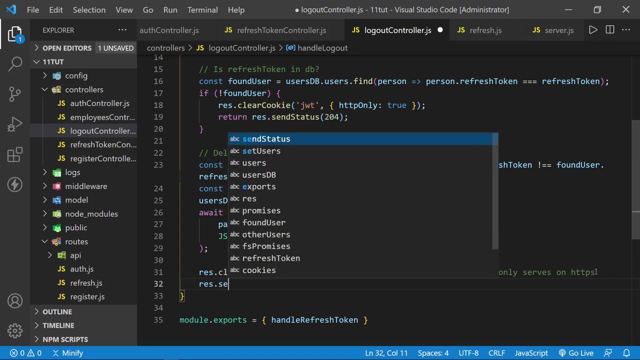 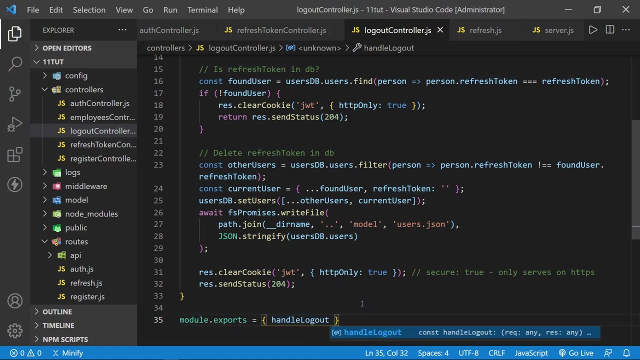 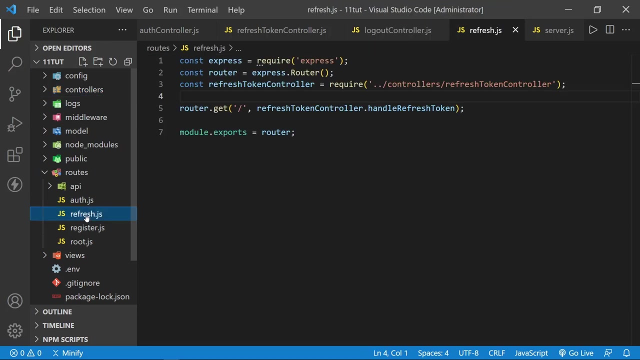 only serve, so it only serves on https. we're just using a dev server that uses http, but you want a secure connection with the. okay, with the controller, complete. let's create our route file and we can just go here to the refresh file we created, select all and copy. and now I'm going to 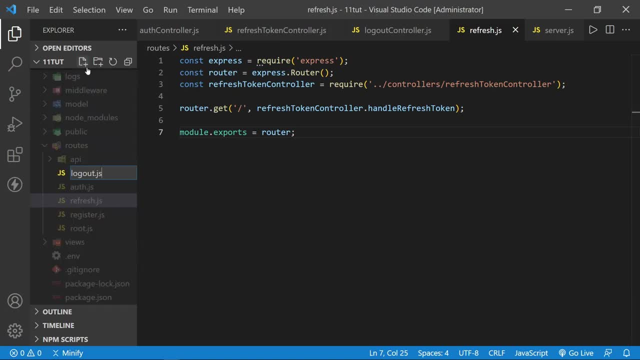 create a new file in the routes called logoutjs, and now I'll just paste everything in from the refresh route and we'll change that. so we need express, we need the router, but instead of refresh token controller we'll select all three of those with control d and I'll just type logout. 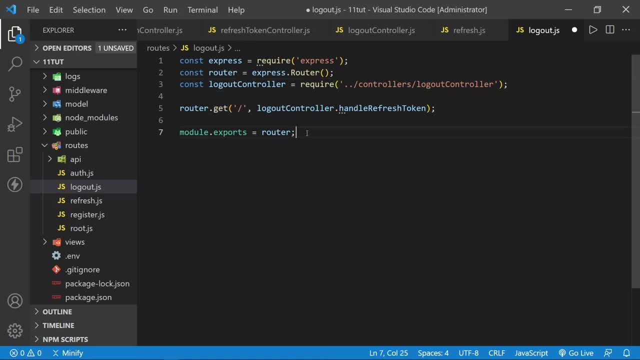 and this will be a git route again, and the export to router is correct. but we do not have handle refresh token here. we also have handle logout as the function for the controller and with that complete. now we can go to the server and add that route as well. we won't need to verify a jwt to log out. so I will just once again. 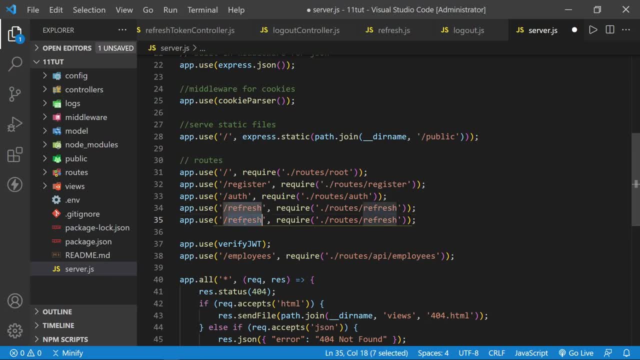 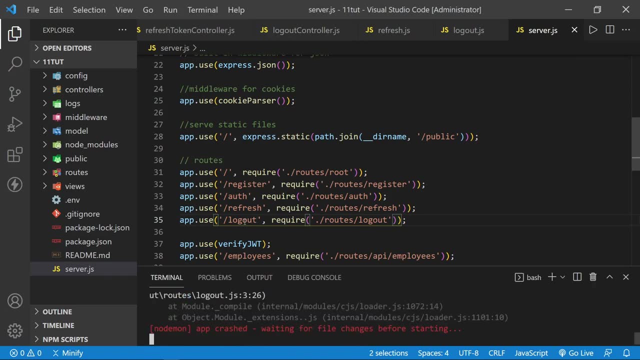 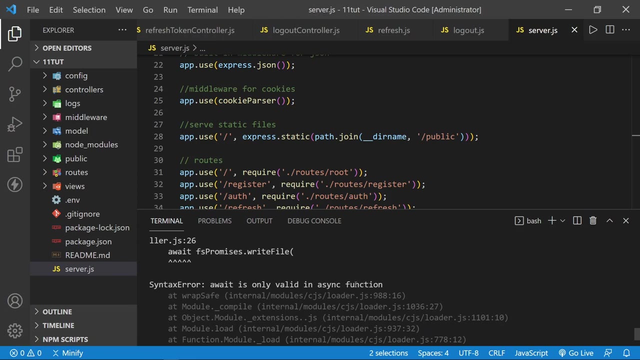 shift, alt and the down arrow to copy a line down and I'll change. refresh to log out and save. now let's open a terminal window again. oh, and we've got an error. so let's see what our error is here in node await is only valid in an async function. ah, we did not. 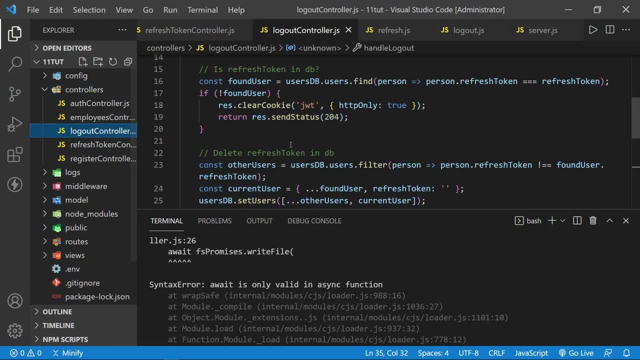 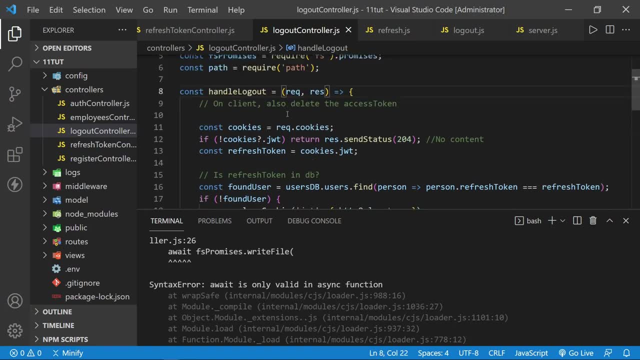 do that in our controller. let's go back to the log out controller and we used a wait when we used fs promises, so let's make the handle log out an async function and save and let's see if node restarts. and yes, that's going to do that. I'm going to go back and refresh our route and now let's click the save button and save. 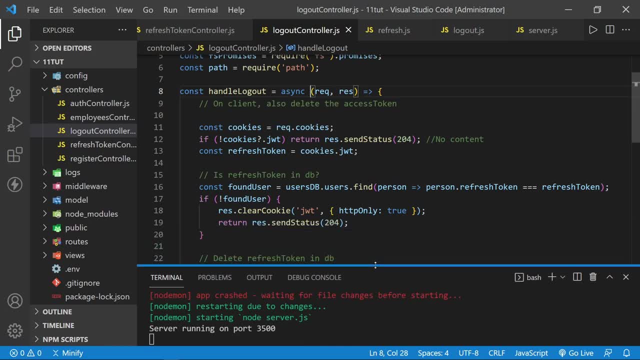 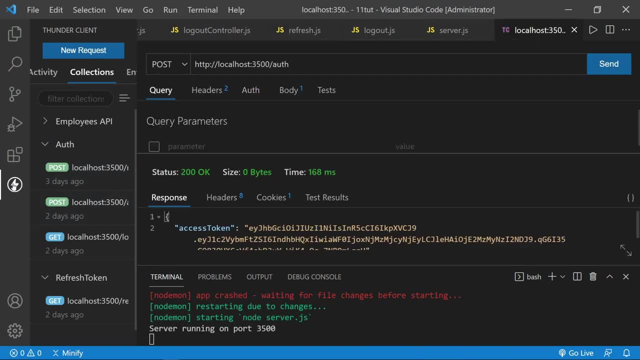 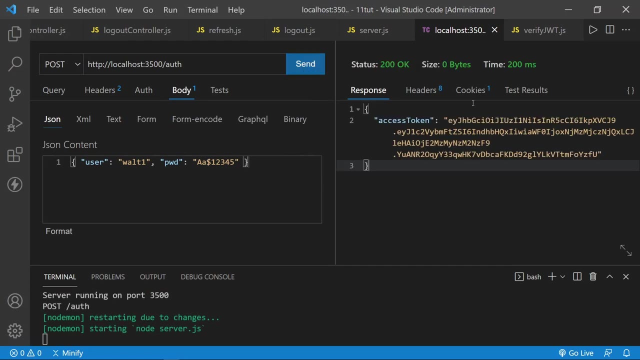 the server is running on 3500.. All looks good there. So now we can go to Thunder Client and we'll hit our auth route to make sure everything is logged in. We're going to log in our user Walt1 and we've got an access token and we've got a cookie. So now let's go back to. 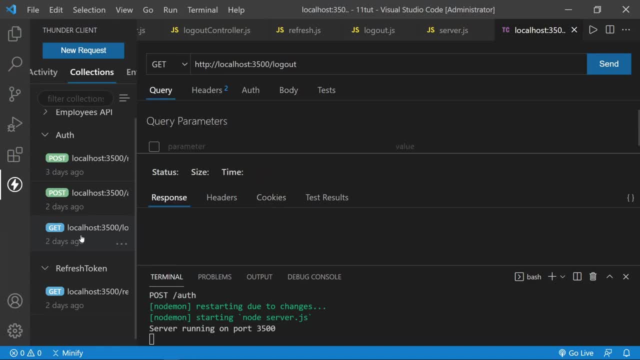 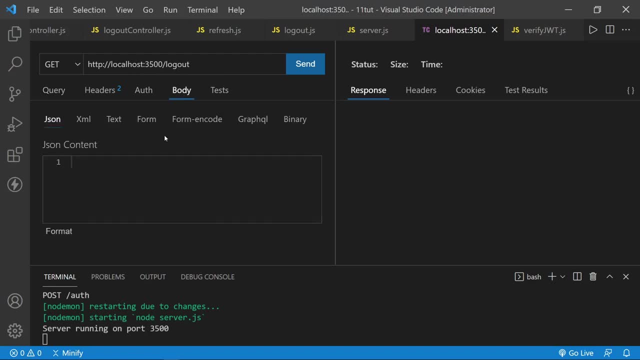 Thunder Client and I have a logout route that is a git route as well. So we have git localhost 3500 logout. You don't need to pass anything in the body or the auth when we log out. but let's go ahead and do that And we hit logout and everything seems to be fine. We can see our. 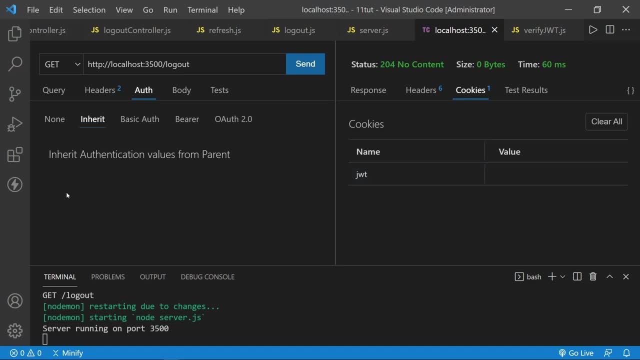 cookie has now been erased. So now, if we go to any of the other routes, like refresh, that would use our refresh token cookie. we don't have a cookie to refresh with. So now let's try localhost 3500 refresh and it's a git. 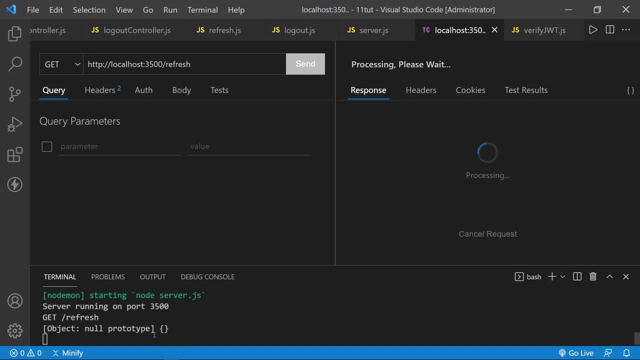 route and see what we get, What we can see in the console. we logged, or attempted to log a cookie, but it didn't exist here and we're not getting a response, So let's look at that. I can cancel this here in Thunder Client. Let's go ahead and look at our refresh controller and see what's. 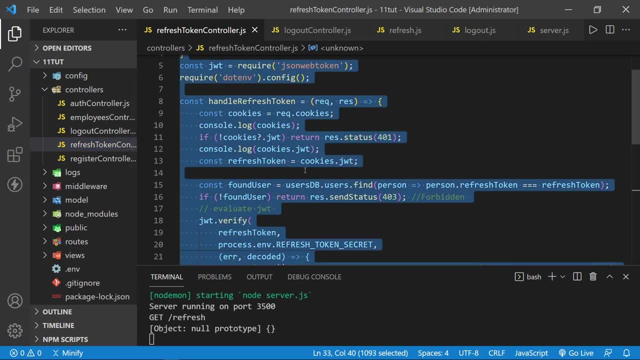 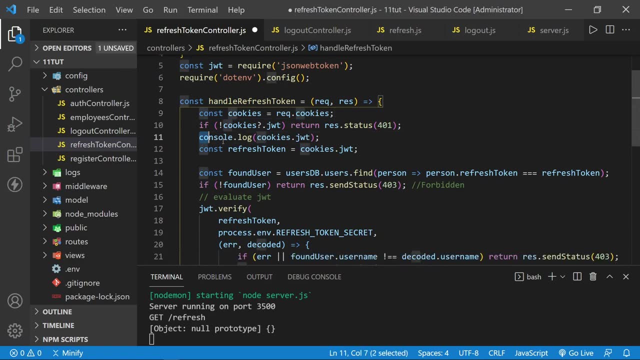 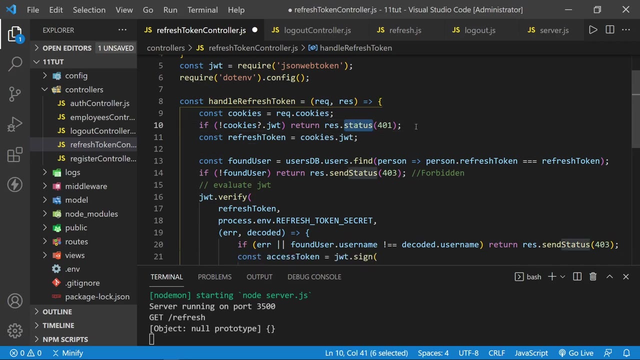 going on there. So refresh token controller and here is where we're logging the cookies. We can get rid of these lines actually now, So we don't need those, But let's see if we can figure out what is going on. And yes, here's the error. I said responsestatus401. 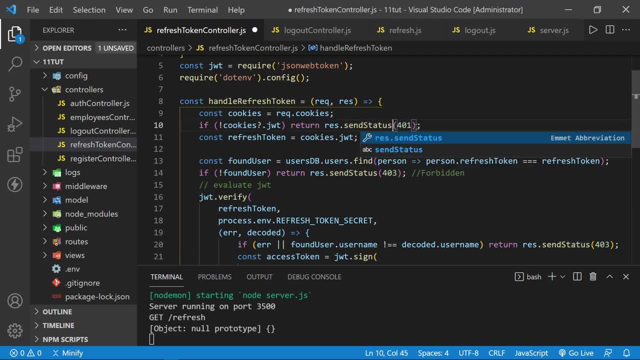 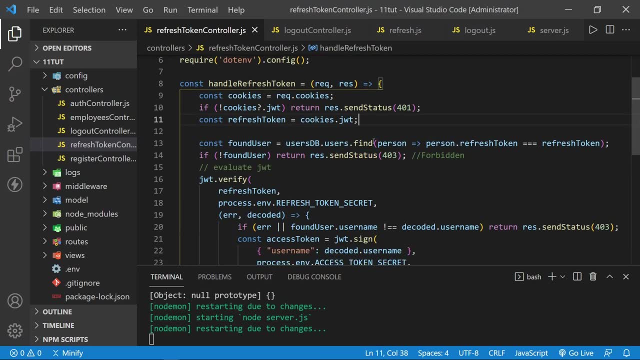 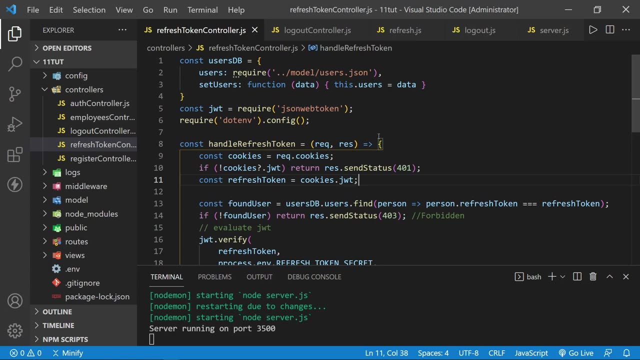 It needs to be responsesendstatus401, just like we had down here with sendstatus403.. So if I've typoed any of those others throughout this code, it looks like I had sendstatus everywhere else. But just in case you see that to actually send the status it needs to be sendstatus instead of just 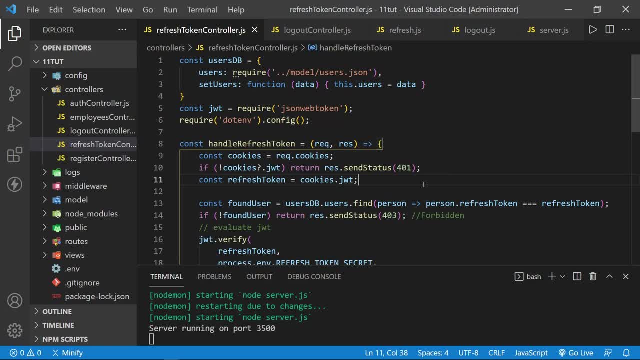 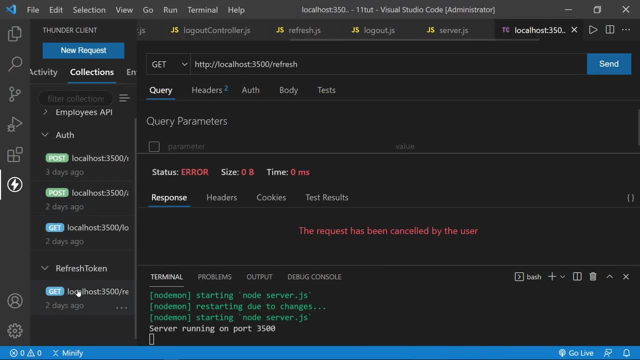 status. Status is chainable in Thunder Client, So I'm going to go ahead and do that. I'm going to hit refreshtokenauth if we're sending a response after that, But now this should work. So let's once again go back to Thunder Client and we'll hit our refresh token route, although we don't have a. 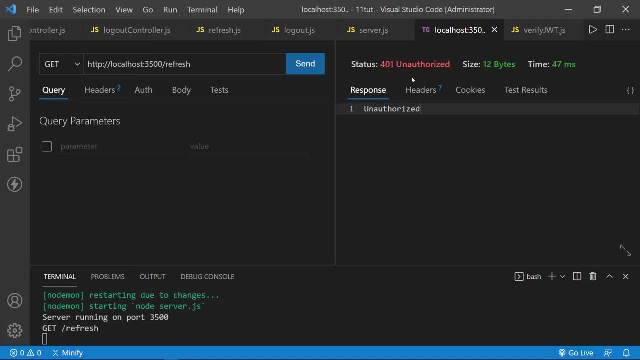 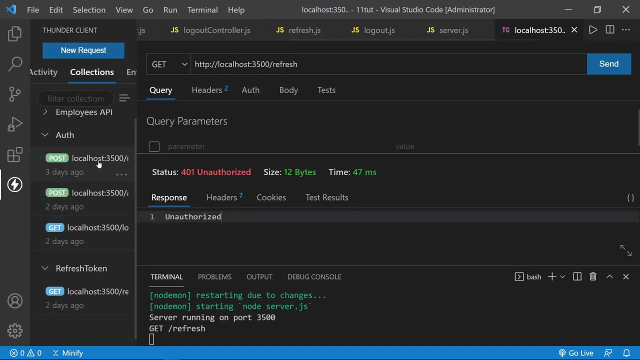 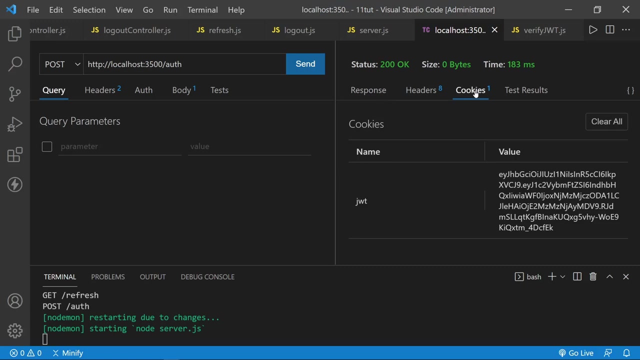 cookie And we'll see what happens. Ah, we immediately got our 401 unauthorized, because now it sends the status. So that's correct. Let's go back and log in again with our auth route: Local host, 3500. auth Send that. We have an access token, We have a cookie And everything. 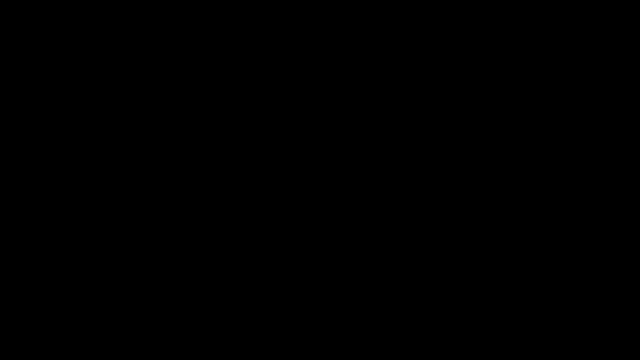 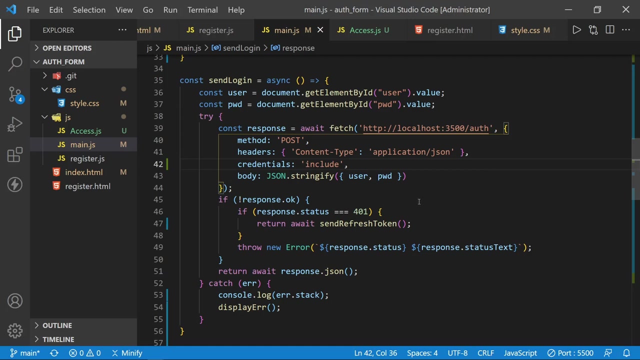 seems good, So all routes are working as expected. Okay, I thought I was at the end of the tutorial, but after playing around with some front end code, there were a few things I thought I needed to go ahead and clear up or include. One is here. This is front end code. by the way, This is not what we. 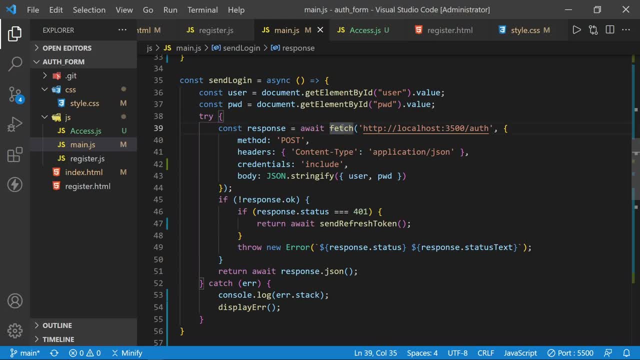 were working on in Express. If you use fetch to access what we had set up, say our auth route, well, you're going to need to include a credentials option Again on the front end to have fetch send the cookie. Now, if you use Axios, I believe there- 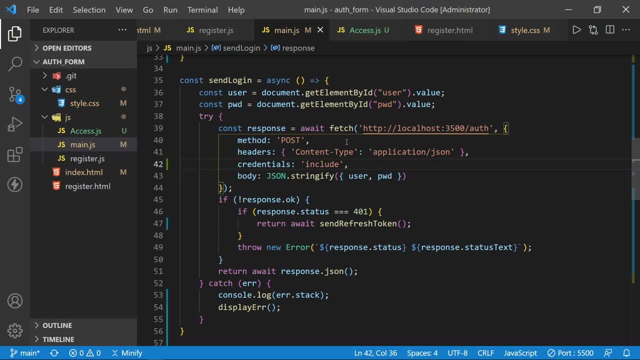 is a with credentials flag. that needs to be set as well, And we could do that in a future tutorial, But right now just looking at credentials for use with fetch. So you have to set that to include, But that sets off a chain of events. So, even though this is required here to send the cookie. 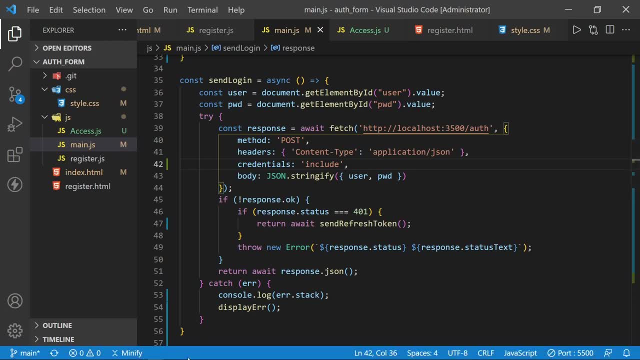 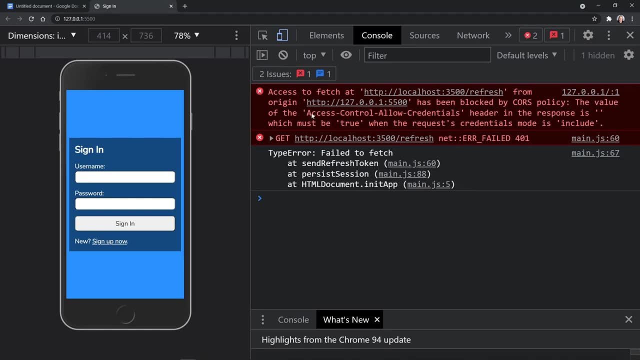 then what happens is- I'll pull up Chrome here- We get a CORS error and you will be blocked by CORS because the value of access control allow credentials in the header of the response is blank and it needs to be set to true, So CORS will block this if you don't have that set before you reach the CORS check. 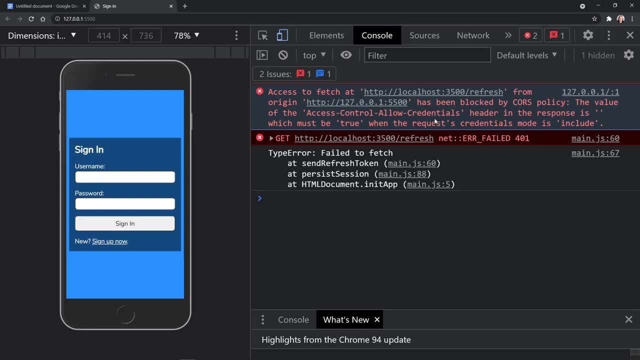 Now what is happening is a preflight options check. It's an options HTTP method request, But then you also need to have this same access control: allow credentials set to true when you do send the cookie back as well, because that's what's expected with fetch. 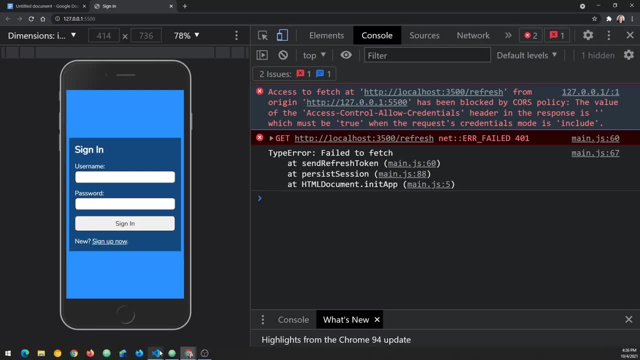 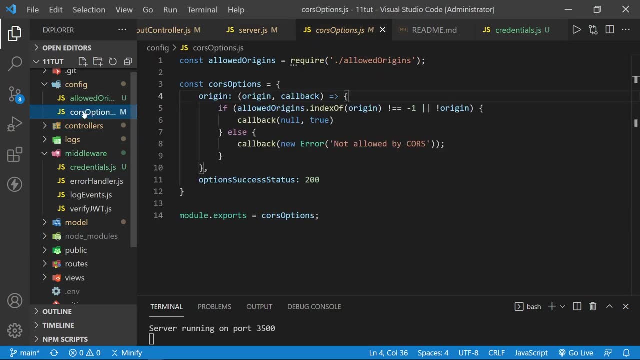 So there's a way to fix that, of course. And now let's look at some of our back-end code. and let's start in the config folder, And I went to CORS options first And we did have what was called a white list in here, which that's traditionally. 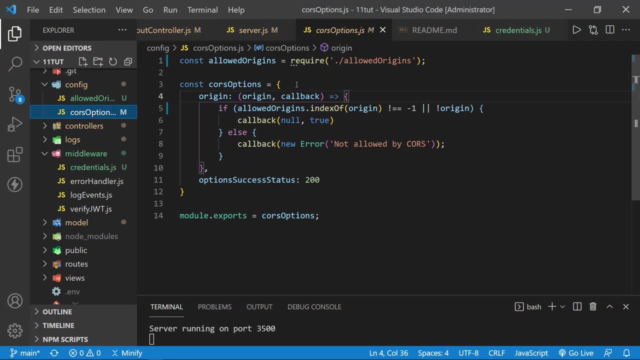 what it's called, And I've seen that in articles as well. I don't like the name so much either, Just maybe in modern day it sounds a little racist or something. So we've switched that to allowed origins, which is what it is. It's a list of allowed origins And I put it in its own file. 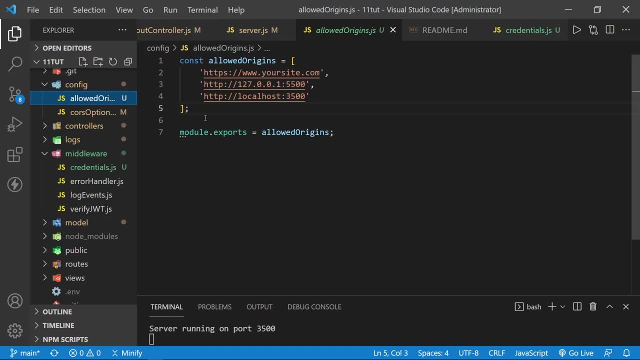 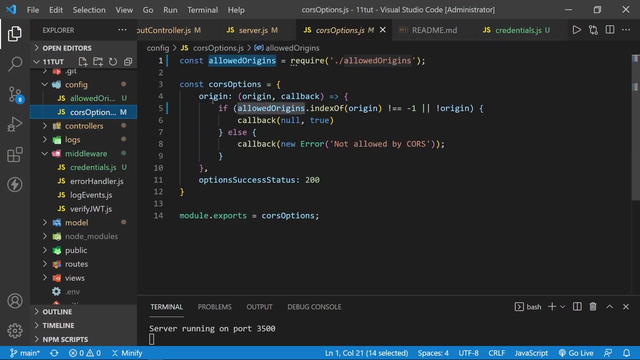 because we're going to use it in middleware also, but I only want to update it in one place. So we have our allowed origins- formerly called the whitelist in the tutorial- and we're exporting allowed origins. So we import that into our cores options and use it here. But then we also create 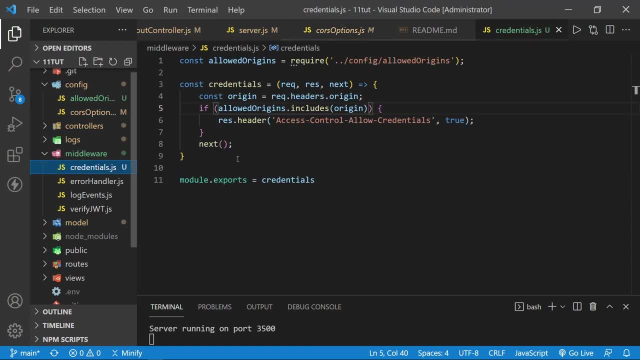 middleware called credentials. And now this credentials middleware of course has a request response. and next, and we import allowed origins. here also, All we're really doing is to say if the origins are allowed, we're going to import them into our cores And then we're going to 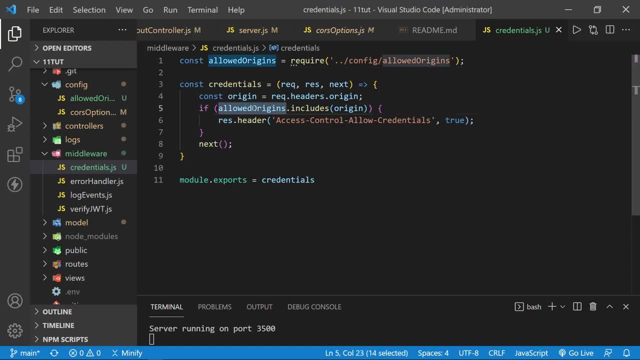 import them into our cores And then we're going to import them into our credentials And then we're origin that is sending. the request is in our allowed origins list, So it's just a little bit of extra security. If that is the case, go ahead and set this header on the response, because that's. 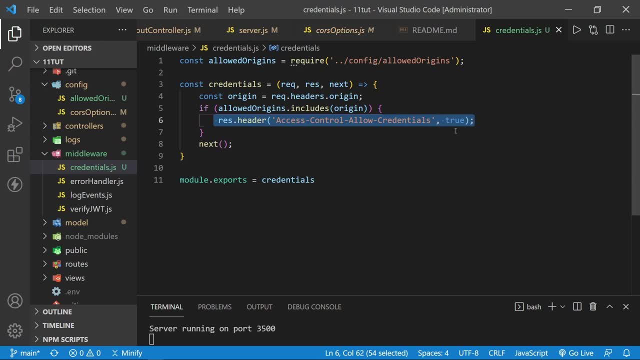 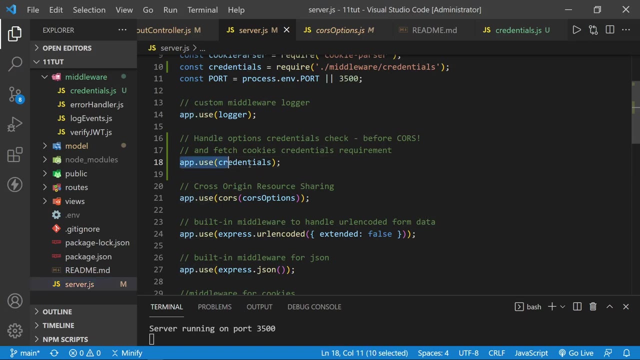 what cores is looking for? Access control allow credentials and we set that to true. So now that we have the middleware created, we go to the server file and we pull that middleware in And then you want to use the middleware. We're using credentials right here And then we're going to import. 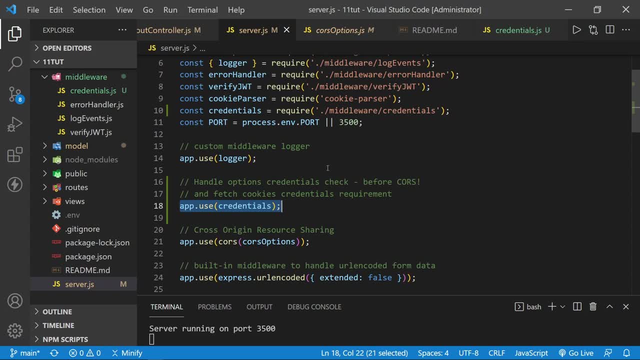 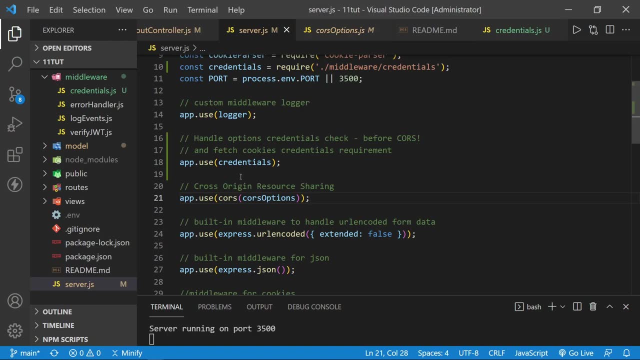 here And of course I'm importing it right up here above. You want to use that before cores because of course sees that that response header is not set. it throws that error. So that will fix that issue And I would hope that would be the end of the issues. But no, there was one other issue. 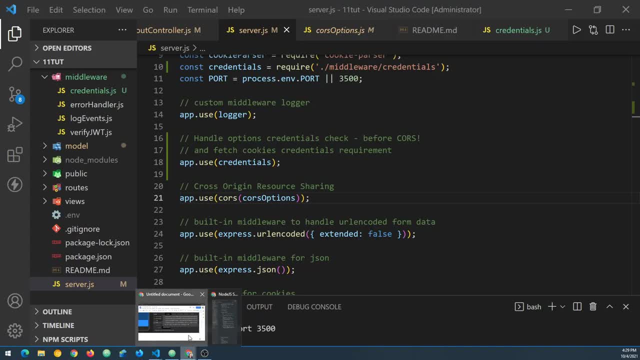 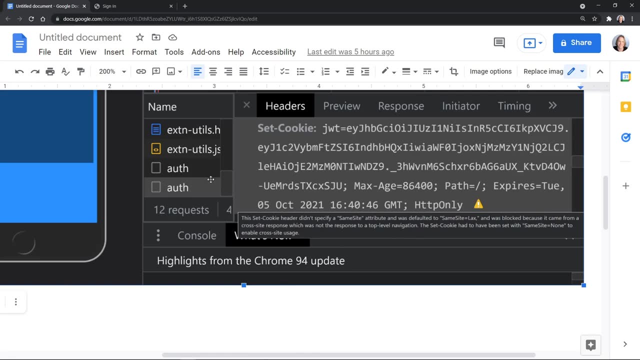 And let's take a look at what that was. I'm going to open Chrome again And I had to do a screen capture. Now I was in the dev tools in the network tab And I was looking at the auth request And then I could pull up the cookie, And then there was this: 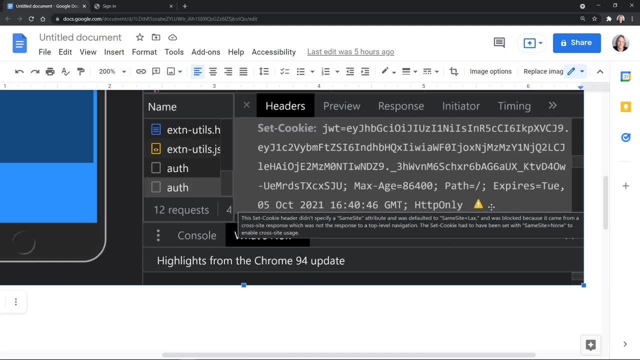 little triangle, And the reason I had to do this screen capture is because I had to mouse over the triangle for this message to pop up And it's very small print. I'm zoomed in quite a bit already just to see this- And it said: the set cookie header didn't specify a same site attribute. So 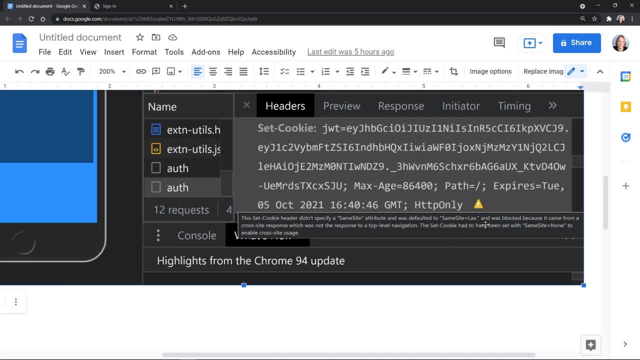 that defaulted to same site equals lax. And then I had to do a screen capture, And then I had to do a screen capture, And then I had to, And then it was blocked because it came from a cross site response, which means our front end. 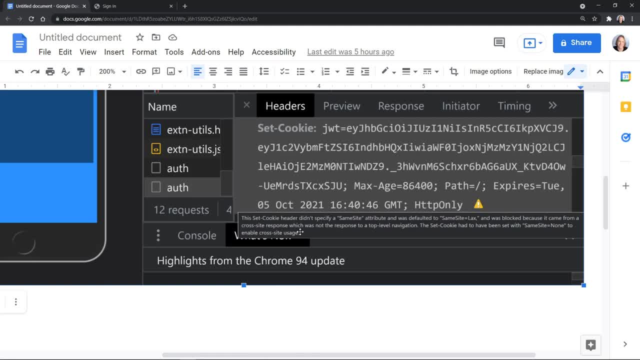 application was not on the same domain as our back end API, And that's often the case, So there's nothing wrong with that. It's just that's why they blocked it. It says the set cookie had to have been set with. same site equals none to enable cross site usage, So that tells us something else. 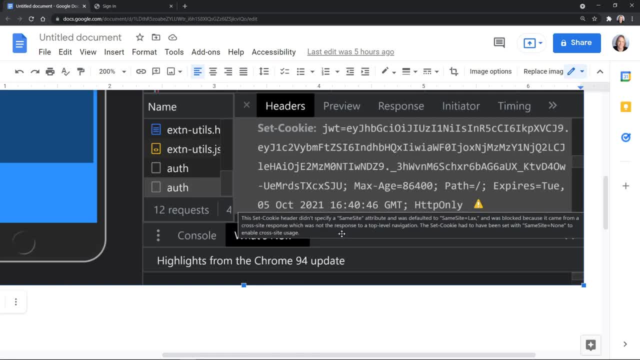 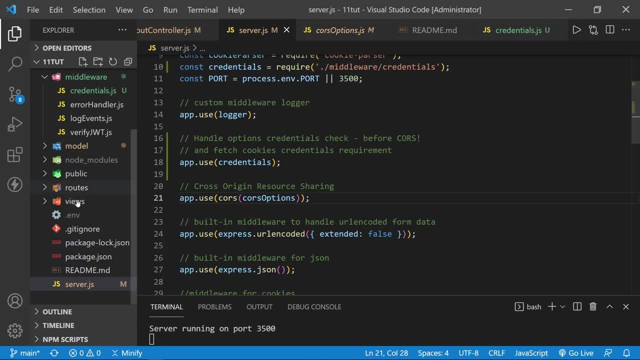 another option. we need to go And put in our set cookie response. So let's look back at the back end code here. And then, where did we set the cookies? Well, let's look at the controllers. That's where the cookies were being. 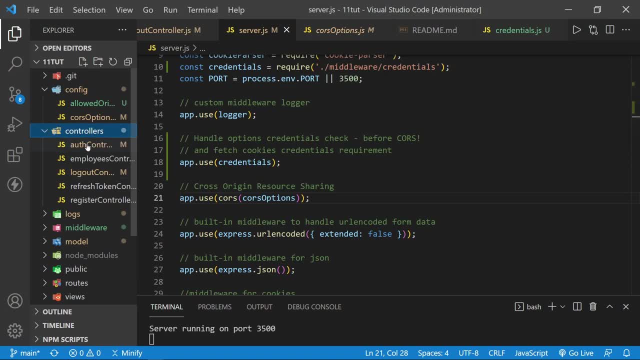 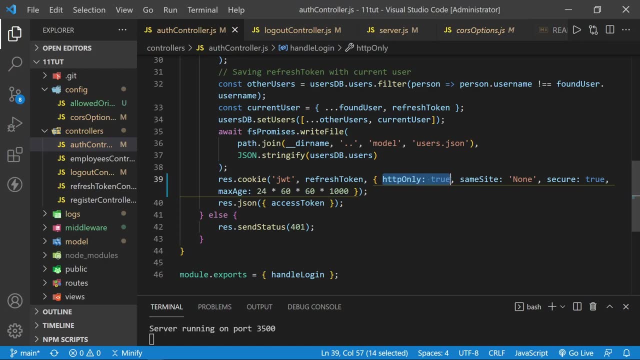 set, And I believe the auth controller is what sets the cookie specifically. And so not only do we have HTTP, only true, but then we went ahead and set same site to none, as they request here, And then, after you do that, they give you another message in the same spot, And that says: secure must. 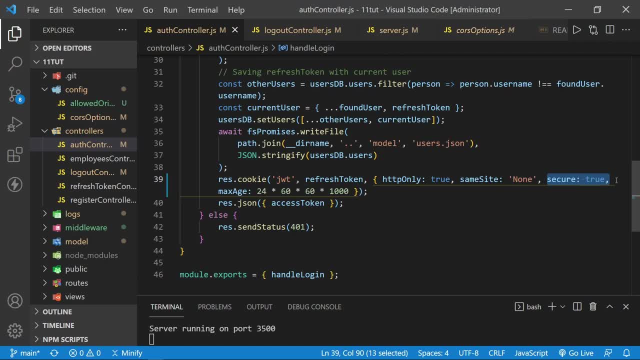 be set to true Now. previously I didn't have secure set to true there Because I thought you could only use it with HTTPS, even during development. But no, it's working in the dev server even though we're just using HTTP. Then, after that, I went ahead. I've got the code wrapping, by the way. 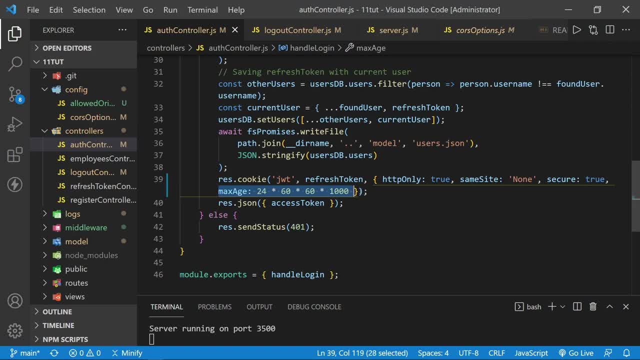 because down here on the next line, you still have the code wrapping. And then, after that, I went ahead. I've got the code wrapping, by the way, because down here on the next line, you still have the max age option. Now, when you delete a cookie, you need to set the same options, However, and